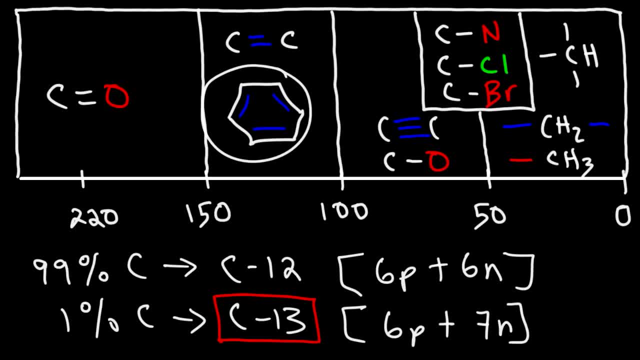 within 100 and 150 parts per million, Alkynes and a carbon, with a carbon that is singly bonded to an oxygen atom will appear between 50 and 100.. Now, this could be an ether, It could be the CO bond of an ester, but it's going to show up in that region, And then we have the 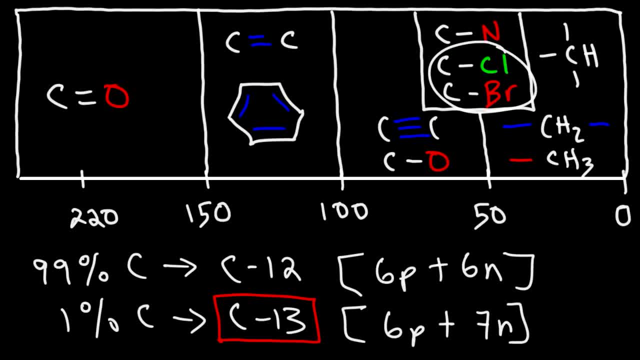 halogens and amines. They're close to 50. Sometimes they could be around 40,, sometimes they could be around 60, but usually around 50-ish. they tend to show up a lot. Now, finally, on the right, we have the sp3 carbons, which exists. 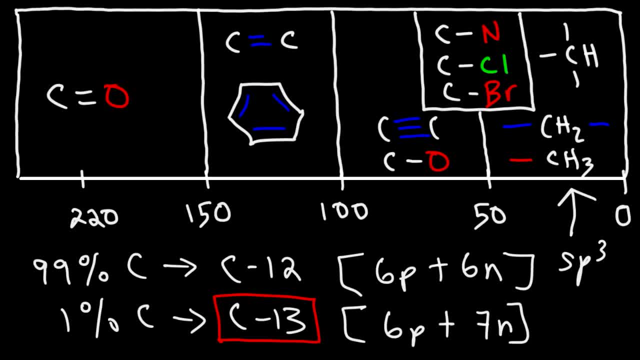 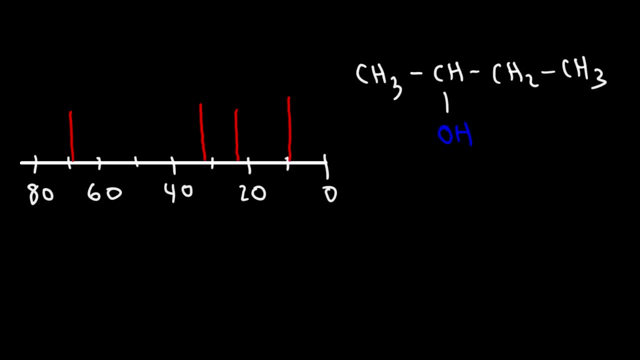 between 0 and 50. So you have the methyl groups, the methylene groups and the methane group. They will show up in that range. So now let's work on some examples. So here we have two butanol and we have the carbon-13 NMR spectrum. 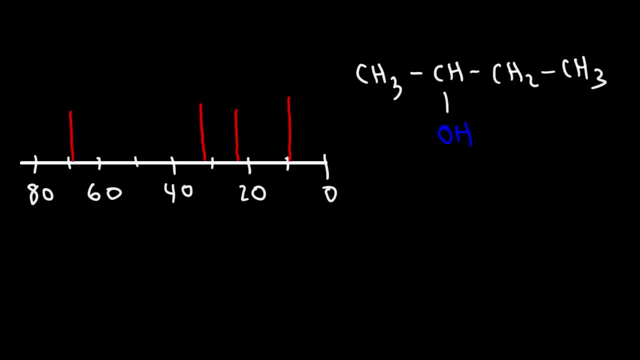 that corresponds to it. So let's match every carbon in this molecule with the appropriate peaks that we see on the graph. If you want to pause the video and try yourself, feel free to do so. So there's four different carbon atoms, which corresponds to four different 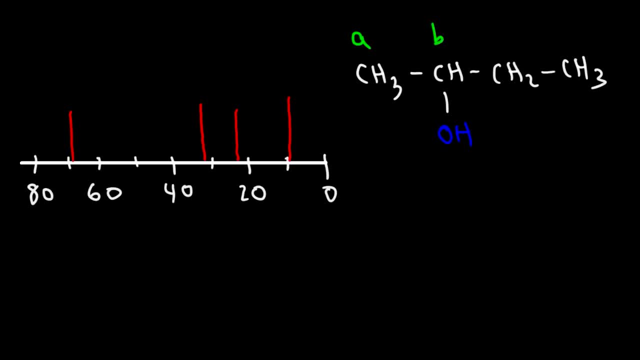 signals. So let's call this carbon A, B, C and D. So which one corresponds to the signal that's just below 70?? Is it carbon A, B, C or D? What would you say? Now? this carbon is attached to an oxygen, so we have an alcohol And, if you recall, the CO, 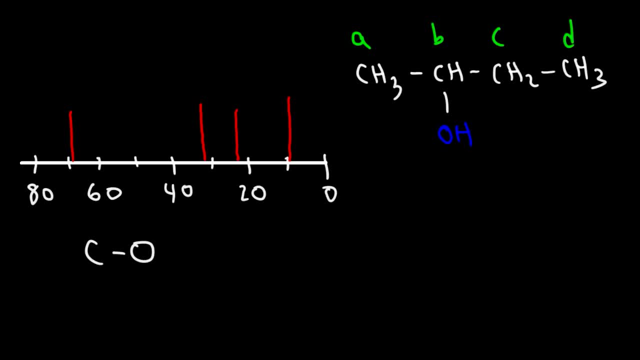 bond for an ether and ester or an alcohol is between 50 and 100. And so we see that at approximately 69. And so, therefore, this will correspond to carbon B. Now, all of the sp3 carbons that's not attached to anything special, as you can see, they're. 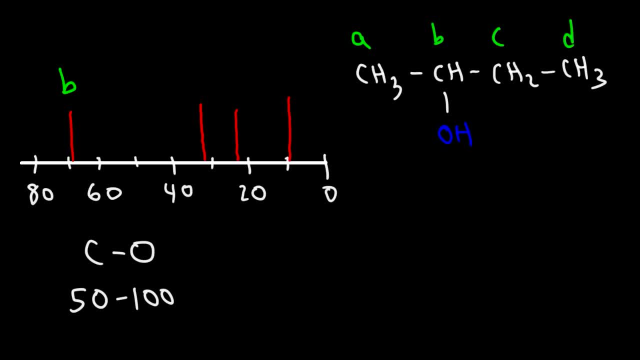 less than 50. But which one is which? What do we do at this point? Here's what we need to understand: A carbon atom that is attached to an electronegative, let's say an oxygen atom, is going to have a high chemical shift. It's going to appear. 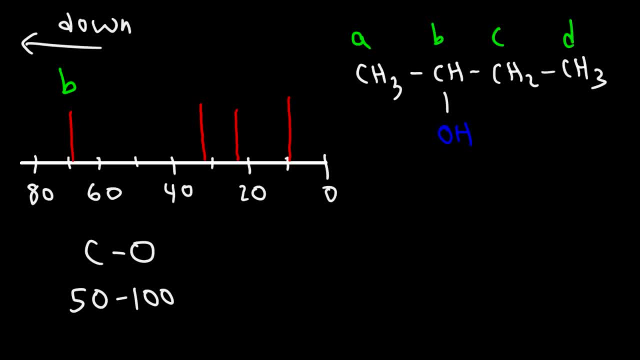 downfield in the graph. Now this methyl group is very far away from the oxygen. It's two carbons away from the carbon that has the oxygen, So therefore we should expect that it's going to be upfield. It's the most shielded carbon. 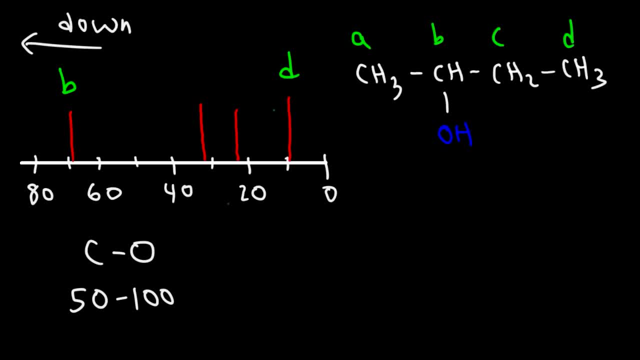 And it is. This is going to be signal D, which has a chemical shift of approximately- I'm going to write it in red- 10.. And the chemical shift for the CH group, that was about 69. Now the methyl group and the methylene group, they're. 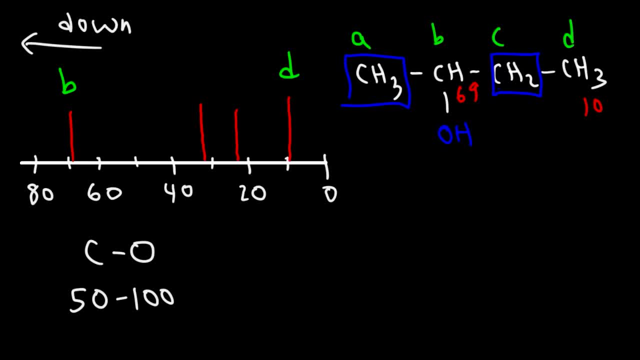 equally distant from the carbon with the OH. So at this point, which one will have the higher chemical shift? Is it carbon A or carbon C? What would you say Now this carbon? carbon C is a secondary carbon And carbon A is a primary carbon. If you study many 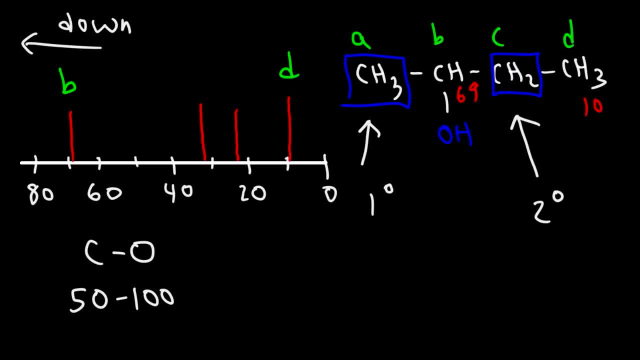 examples, you'll find that secondary carbons tend to have a higher chemical shift than primary carbons in C13 NMR spectroscopy. But now there's more to it than that, But for now this will suffice. But keep this in mind: Carbons in the interior of a carbon-carbon chain tend 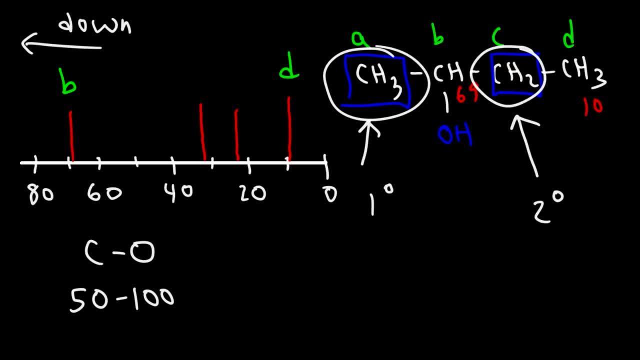 to have a higher chemical shift than the carbon atoms at the end, And that's pretty consistent. So it turns out that carbon C is the one that appears around 32. And carbon A is the signal that appears approximately around 23.. So keep that in mind: Carbon atoms in the interior of an alkane chain, or it could. 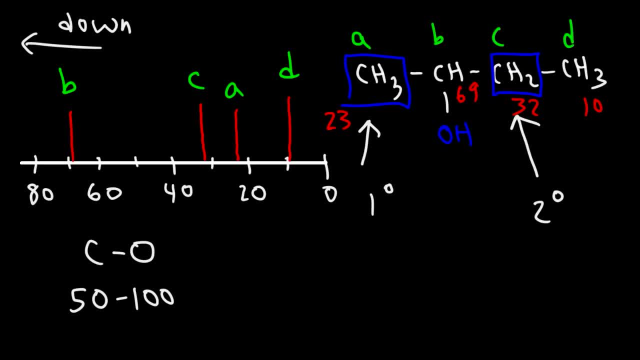 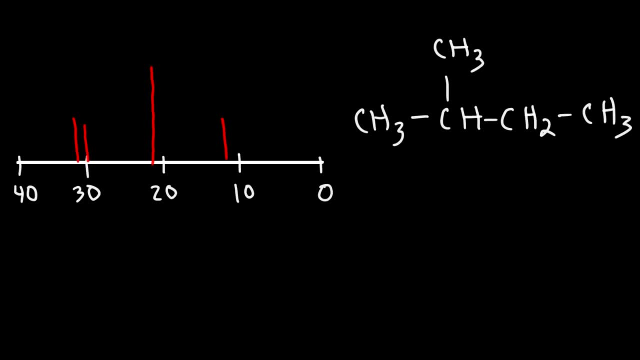 be a different functional group, tend to have a higher chemical shift than those at the end. Now let's consider our second example, which is 2-methyl butane. So if you want to pause the video and match each carbon atom with the signals that we see here, 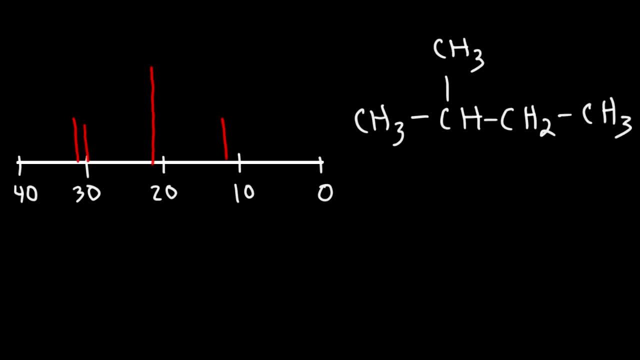 So notice that we have a total of four signals in this graph, But we have a total of five carbon atoms. That means two carbons are equivalent to each other And we can see that these two methyl groups are equivalent. So we have four different carbon atoms. So let's. call this carbon A, carbon B, C and D. Now here's a question for you: Which carbon atom will have the lowest chemical shift at 12? And which one will have the highest chemical shift at 32?? What would you say? Now, you might be inclined to think that the one with the lowest chemical shift will be the primary carbon, And for the most part you would be correct. But notice that we have two different types of primary carbons Here. this methyl group is primary and so is the methyl groups that corresponds to carbon A. So which one will have the signal? Carbon C is secondary, Carbon B is tertiary. Now you might be inclined to think that the tertiary carbon will have the highest chemical shift. In this example, it turns out that the secondary carbon has the highest chemical shift, That's signal C, And the tertiary carbon has a chemical shift at 30.. 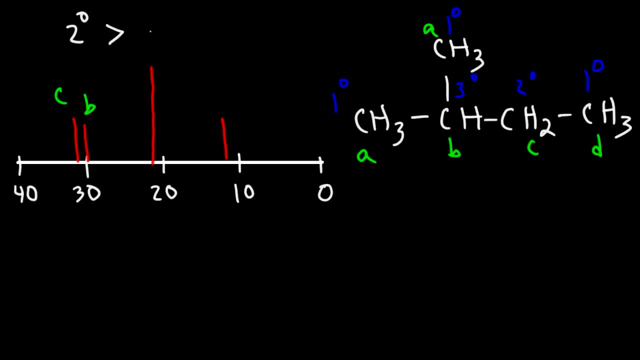 So in this case, the secondary carbon has a higher chemical shift than the tertiary carbon. Now you might be wondering: why is that? I'll give you a hint. The key is not to focus on the carbon you're analyzing, but on the adjacent carbon atoms, Because it is the adjacent carbon atoms that will create a shielding or 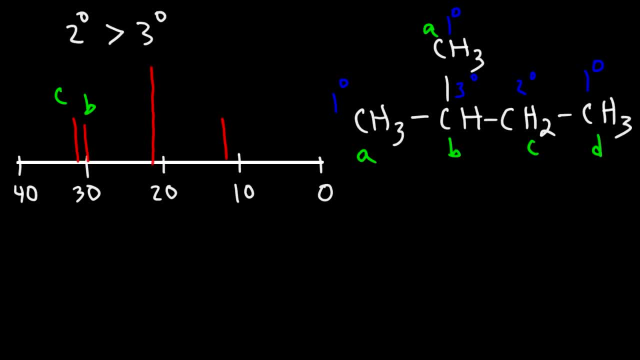 deshielding effect on the carbon that you're analyzing, And we'll talk more about that later. Now these two signals. the remaining two has to represent the two different primary carbons, Carbon A and carbon D, But which one? Now there's a way that you 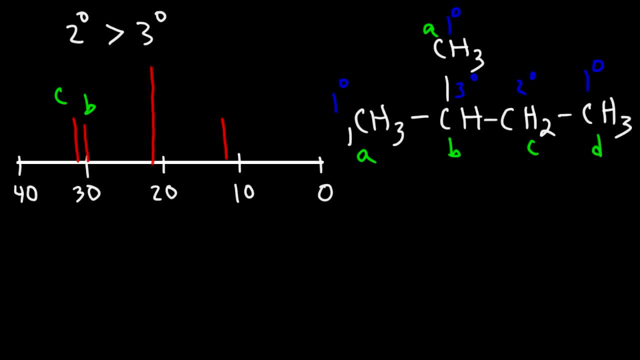 can tell the difference between the two. Notice that there's two carbon atoms that correspond to signal A, So therefore we should expect that the peak should be taller, Which we do. see that this peak is taller than the rest, And so this corresponds to C. 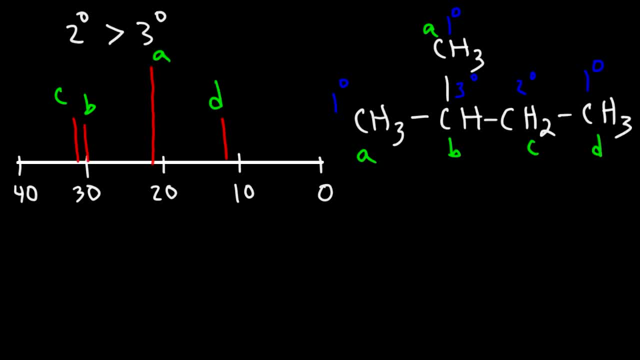 To signal A, Which means the other one corresponds to signal D. But if these are both primary carbons, why does signal A has a significantly higher chemical shift than signal D when they're both primary? And once again you need to look at the 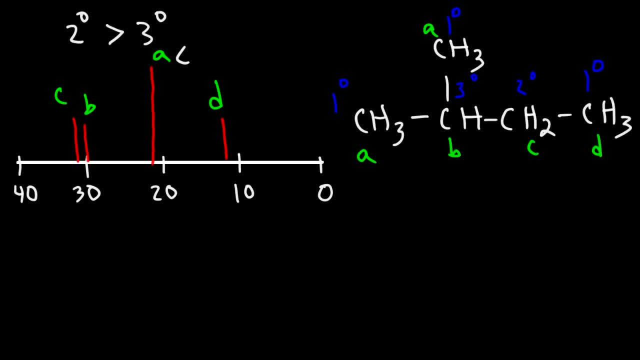 adjacent carbon atoms, And so let's talk about that. right now. We're going to discuss a system that will help us to determine which carbon atoms will have a higher chemical shift and which ones will have a low chemical shift. Now it's just a score system, and it's very useful when dealing with sp3. 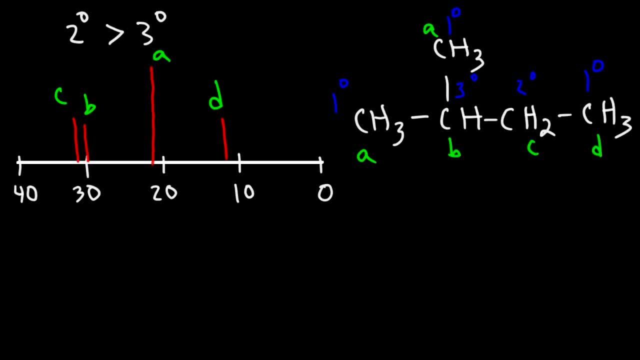 carbon atoms And, generally speaking, it usually works. You might find some exceptions, but for the most part, the results are pretty consistent. So let's look at carbon D Now focus on the adjacent carbon. Carbon D is attached to a secondary carbon, So we're going to give it a score. 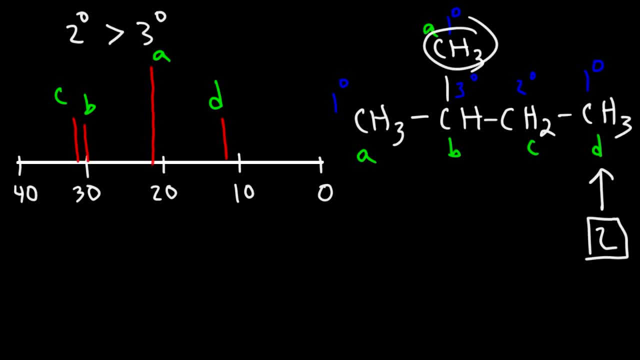 Of 2.. Now carbon A is attached to a tertiary carbon, So we're going to give it a score of 3. And so, using this system, we could see why signal A has a higher chemical shift than signal D. Now, looking at the tertiary carbon, Carbon B. 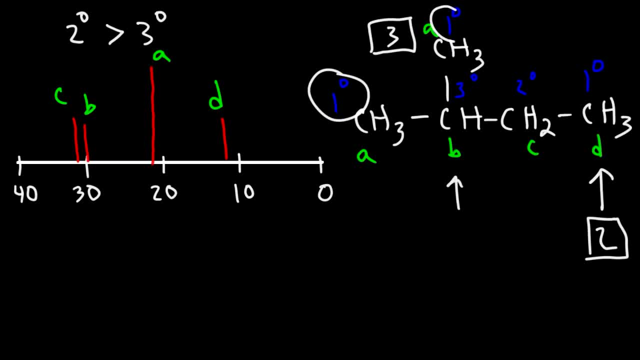 It's adjacent to a primary, another primary and a secondary carbon. So 1 plus 1 plus 2.. That's going to be a 4.. Now, if we look at the secondary carbon, it's adjacent to a tertiary carbon and a primary carbon. 3 plus 1 is 4.. Now these? 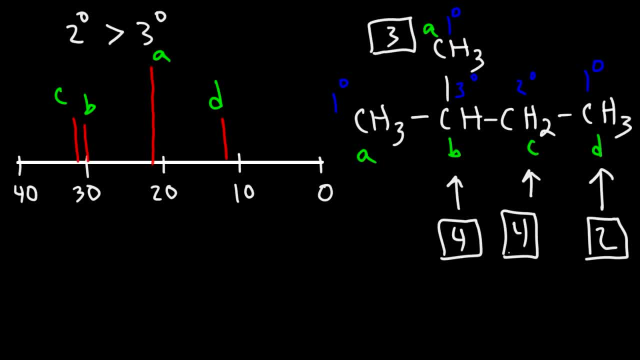 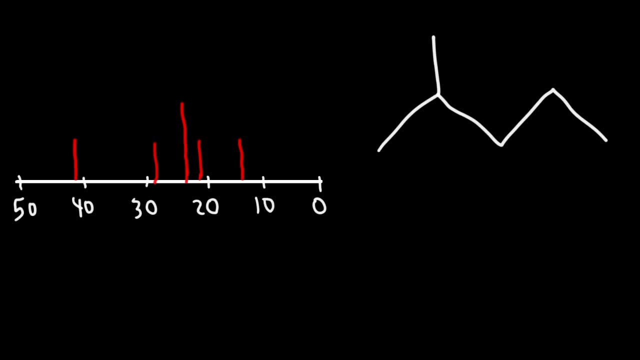 two have an equal score And so when you get to a situation like this, you can't really tell them apart. As you can see, they're pretty close here, But if the score is different, the chemical shifts will be significantly different that you can tell them apart. Now, in this example, we have two. 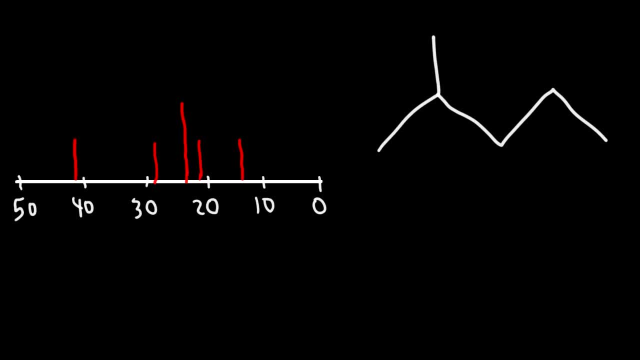 methylpentane. So go ahead and assign the carbon atoms to the chemical shifts that we see in the spectrum. So first let's identify the carbon atoms. These two methyl groups are equivalent to each other, So we'll call it carbon A and then 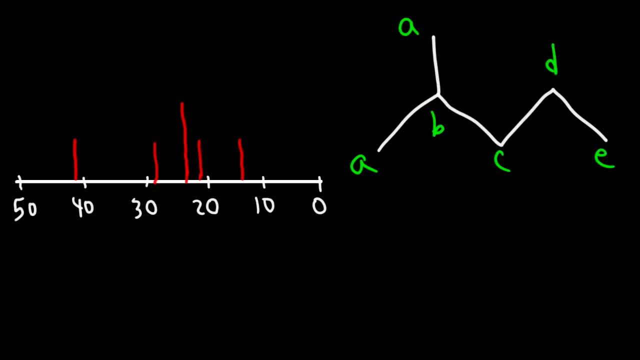 B, C, D and E. So automatically, because there are two methyl groups corresponding to signal A. we're going to have two methyl groups corresponding to signal B. So automatically, because there are two methyl groups corresponding to signal A. we know it's going to be the tallest peak, So it's going to have a chemical. 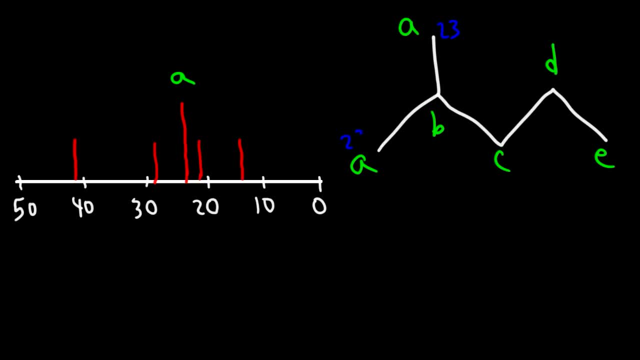 shift of approximately 23.. Now, what about the rest? Well, we know E, the other primary carbon, has to be the one with the lowest chemical shift. So that's going to be the signal of about 14.. To distinguish the others, we need to use a 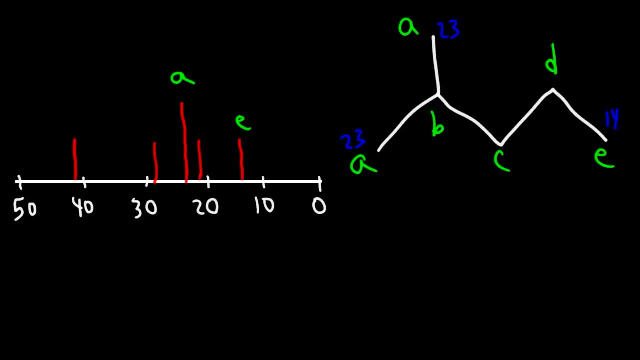 little more information, So we're going to have to use a little more information. So let's begin by identifying each carbon atom as either primary, secondary or tertiary, So we know the signals for, or the carbon atoms that correspond to. signal A is primary and carbon E is primary, D and C are secondary carbons and 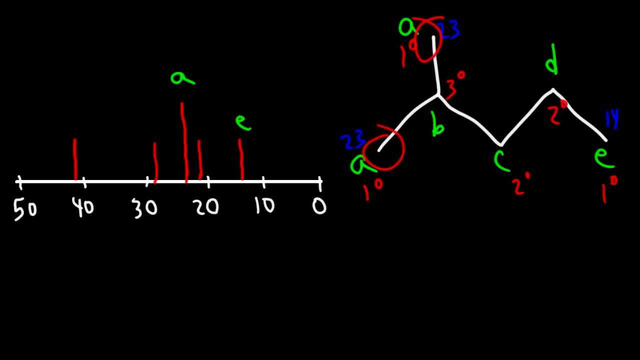 B is a tertiary carbon because it's attached to three other carbon atoms, So we're going to give it a score of 2.. Now, starting with signal E. this carbon is attached to a secondary carbon, So we're going to give it a score of 2.. Now for 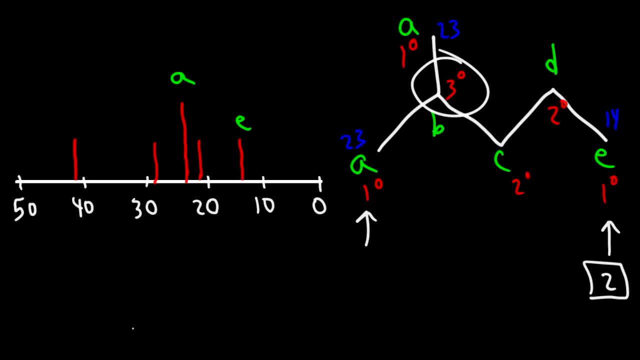 signal A, that carbon is attached to a tertiary carbon, So it's going to get a score of 3.. And so we can see why signal A has a higher chemical shift than signal E. Now let's go ahead and take a look at the other carbon atoms. So we're going to 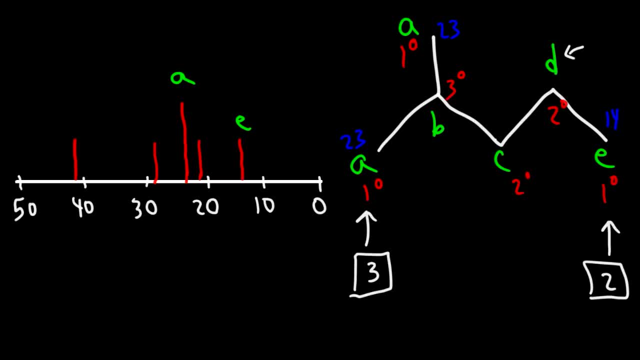 look at that signal d. It's between a second carbon and a primary carbon, So it has a score value of 3.. Now for carbon C: it's between a tertiary and a secondary carbon, So we're going to give it a score value of 5, because 3 plus 2 is 5.. Now for 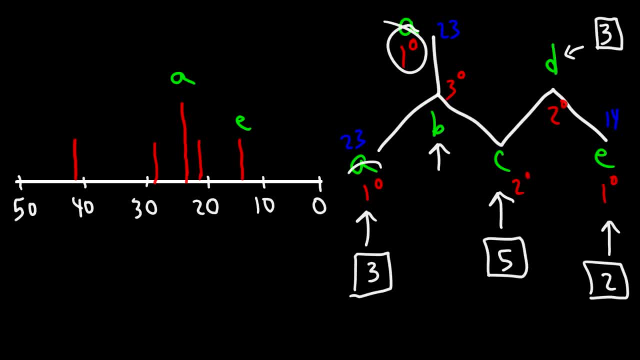 carbon B, it's adjacent to a primary carbon and a primary carbon Corp. 3 is so 7 to and a secondary. 1 plus 1 plus 2 is 4.. So it's going to have a score value of 4.. 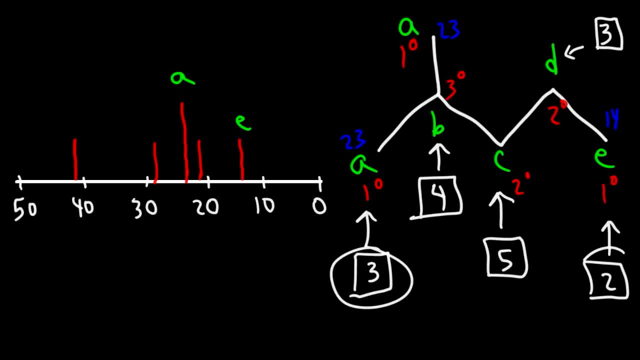 So if we look at carbon A and carbon E, both are primary, but because carbon A has a higher score value, it has a significantly higher chemical shift: 23 compared to 14.. Now, which one do you think is the one with a signal of 42?? This is going to be carbon. 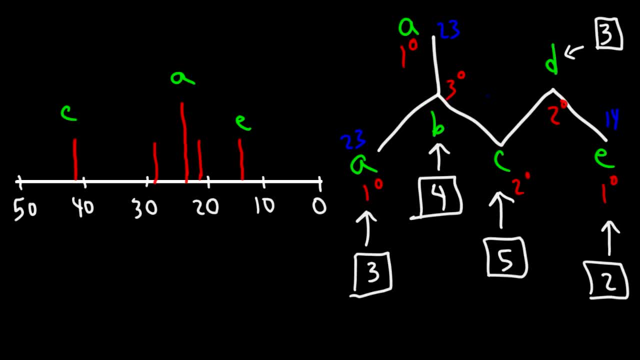 C, because it has the highest score value of 5.. Next up is carbon B, because it has a score value of 4.. And then, by default, this has to be carbon D. Now notice that A and D are close to each other, And it makes sense because they have 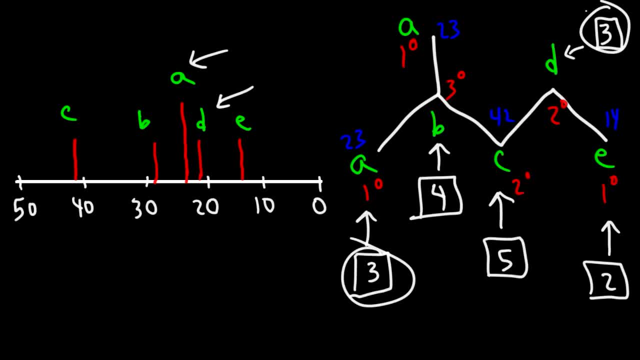 the same score value, So you can't really tell which one is going to have the higher chemical shift, even though D is secondary and A is primary. So sometimes a primary carbon can have a higher chemical shift than a secondary carbon. Carbon B is a tertiary. 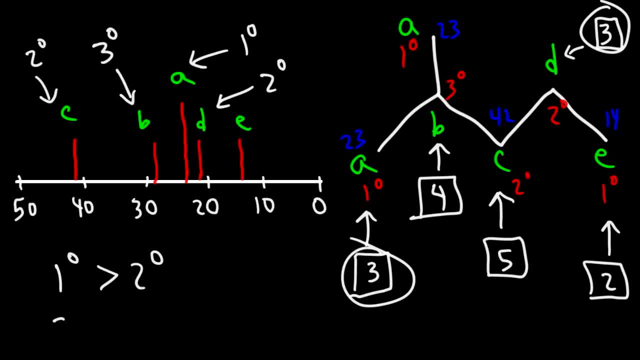 carbon and carbon C is a secondary carbon. So sometimes carbon A is secondary and carbon C is secondary. So sometimes carbon B is a tertiary carbon and carbon C is a secondary carbon, And sometimes a secondary carbon can have a higher chemical shift than a tertiary carbon. 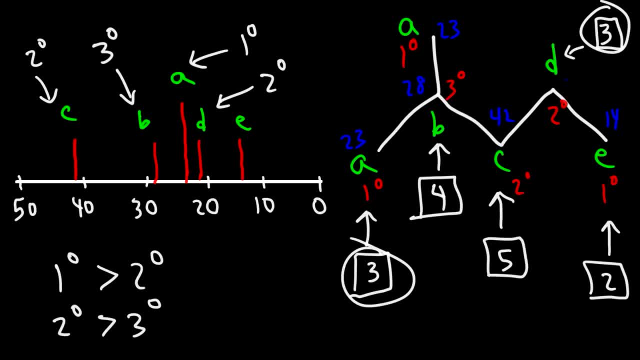 So carbon B has a signal of 28, and D has a signal of, we'll say, 21.. But notice that the score system is pretty consistent, Because carbon C has the highest score. it has the highest chemical shift of 42. Next up is carbon B, with a score of 4,, which has the 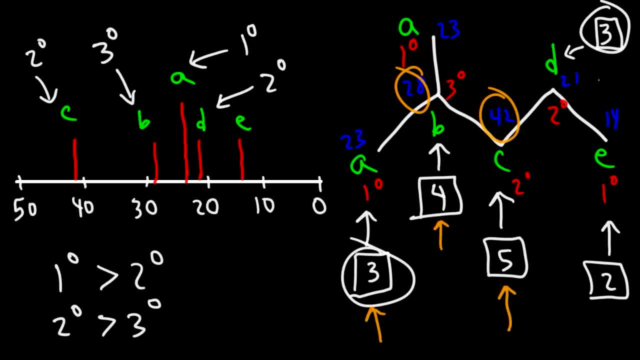 second highest chemical shift of 28.. These two have the same score, so their chemical shifts are very close. And finally, carbon E has the lowest score, so it has the lowest chemical shift, And that technique is very useful for ranking the different carbon atoms. 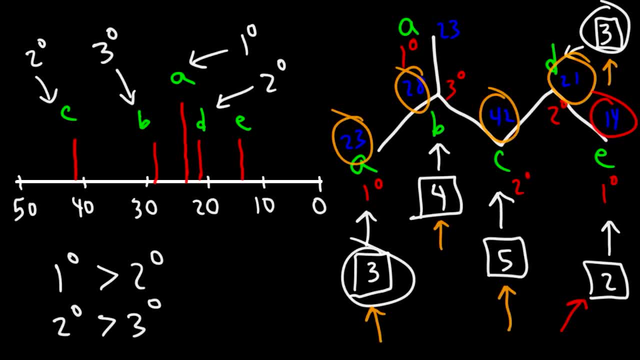 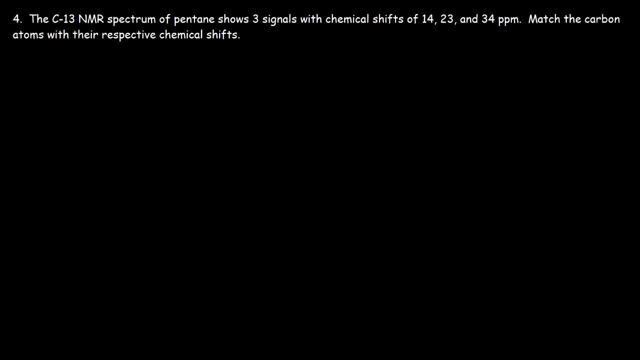 when dealing with alkanes in carbon-13 NMR spectroscopy. Let's work on our fourth example. So let's start with our first example, where we have a spectrum of pentane and we're going to look at the spectrum of pentane and we're going to look at the spectrum of pentane. 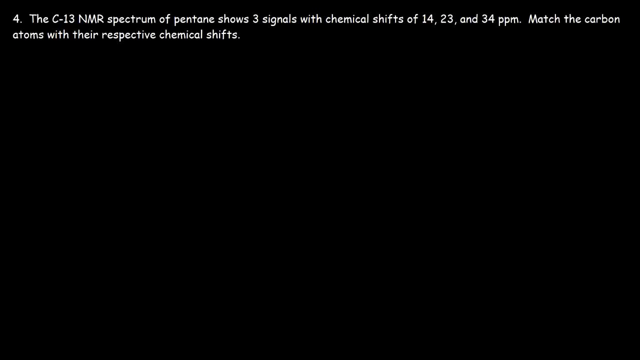 So the spectrum of pentane shows three signals with chemical shifts of 14,, 23, and 34 parts per million. Match the carbon atoms with their respective chemical shifts. So let's begin by drawing pentane, These two methyl groups on the left side and the right side. they're going to be identical. 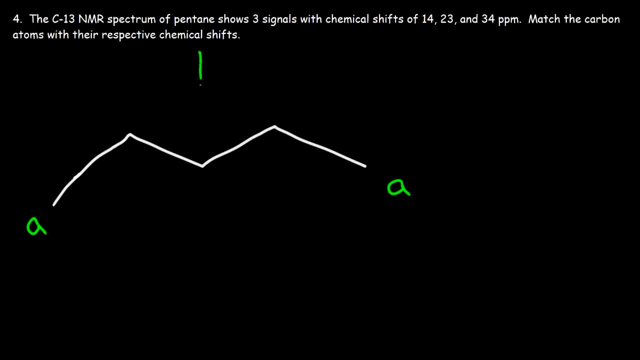 They have the same exact chemical environment, And here is the line of symmetry. So therefore, these two carbon atoms will be similar and carbon C will be in the middle. It will be different from the rest. Now let's determine the types of carbon atoms that we have. Carbon A are primary Carbon. 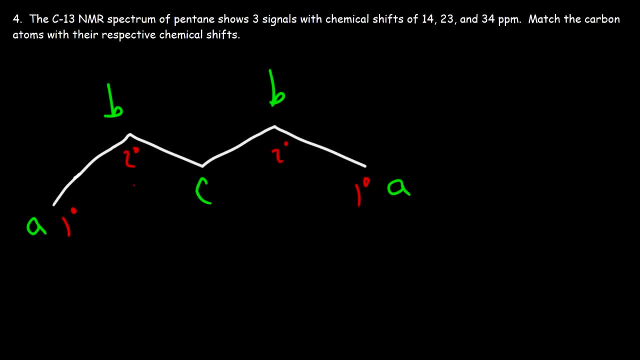 B. they're secondary carbons because they're attached to two adjacent carbon atoms, And carbon C is also a secondary carbon atom. So now let's calculate the score for each different type of carbon. So for carbon A, it's adjacent to a secondary carbon, So let's give it a score of 2.. Carbon B is adjacent. 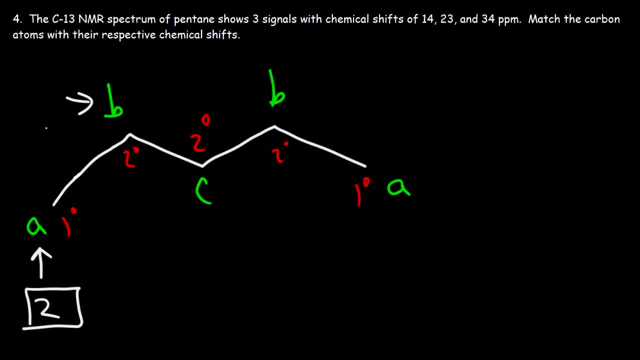 between a primary and a secondary. So 1 plus 2 is 3, and carbon C is next to two secondary carbons. 2 plus 2 is 4.. Now, since carbon C has the highest score value, it turns out that it has the highest chemical shift, in this case of 34.. 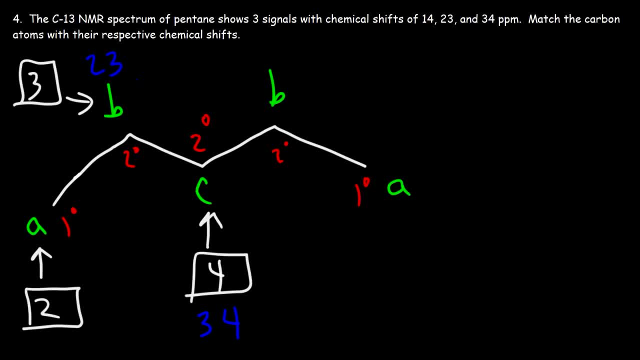 Carbon B has the second highest, which is 23,. and carbon A is going to have the lowest. And you can look this up If you type in the C13 NMR spectrum of pentane, you do a Google search and if you look at chemicalbookscom they'll have those values. 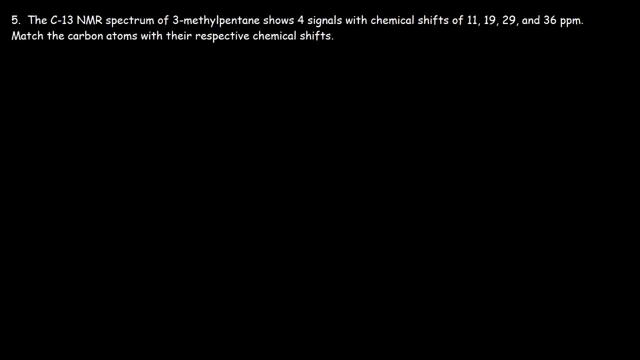 So that's it for this example. Try this one. So this time it's 3-methylpentane and it has four signals, with chemical shifts of 11,, 19,, 29, and 36 parts per million. So let's begin by drawing pentane and let's put a methyl group on carbon 3.. 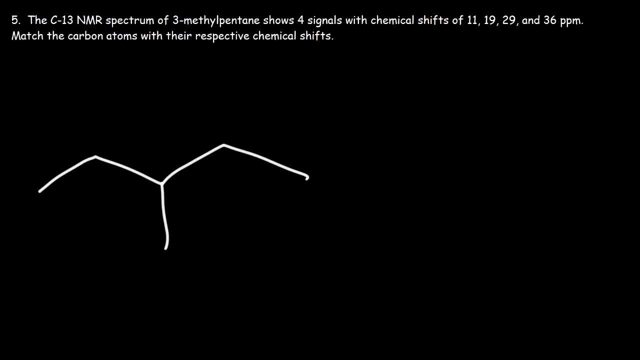 So, just like before, let's identify the different types of carbon atoms that we have. So here is the line of symmetry. So this is going to be carbon A, B, C and D. So we have four different types of carbon atoms, which correspond to the four signals that we see here. 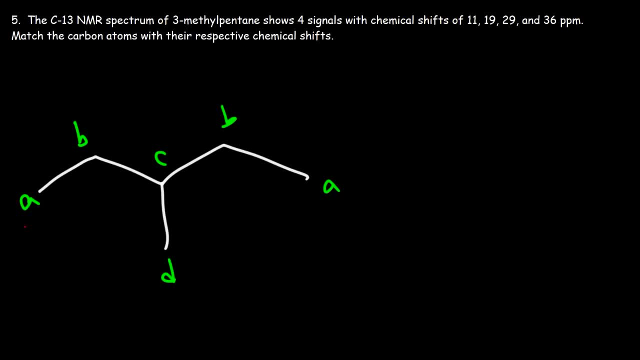 Next let's identify each type of carbon. Carbon A is primary, carbon B is secondary, C is tertiary and D is primary. Now let's focus on the score values. So carbon A is adjacent to a secondary carbon. It's going to have a score value of 2.. 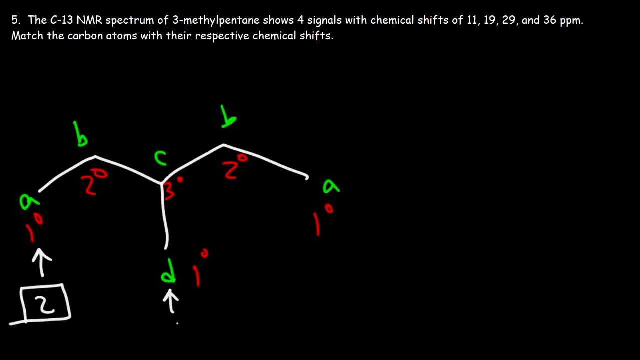 Carbon D is adjacent to a tertiary carbon. It's going to have a score value of 3.. Carbon B is between a primary and a tertiary carbon. 2 plus 3 is 4.. And carbon C is adjacent to a secondary, another secondary and a primary. 2 plus 2 plus 1 is 5.. So, based on this score system, carbon C is going to have the highest chemical shift of 36.. Carbon B is next. It's going to have a chemical shift of 29. And then carbon D has a score value of 3.. 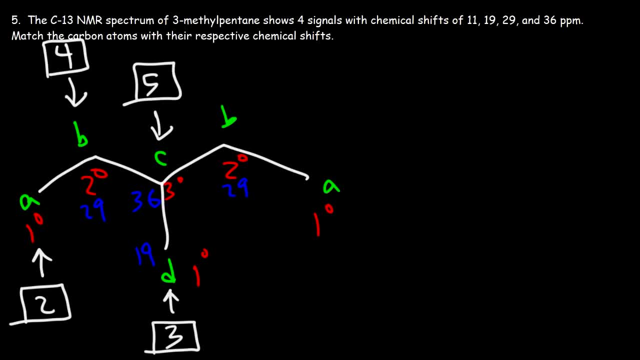 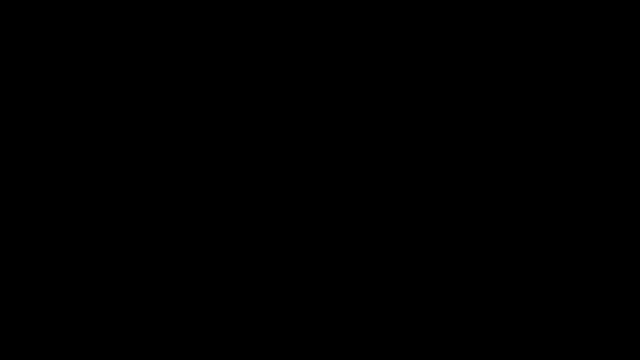 The chemical shift will be 19.. Carbon A has the lowest score value of 2,, which means the chemical shift is going to be 11.. Earlier in this video we said that alcohols, ethers, esters, their CO bonds, have a chemical shift between 50 to 100. 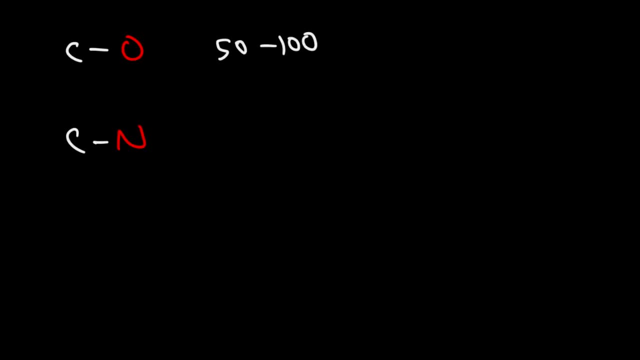 And then we grouped the amines with halogens such as chlorine and bromine To be close to 50. So we're going to talk about that in this case. So first, here we have. this is going to be 1-hexanol. 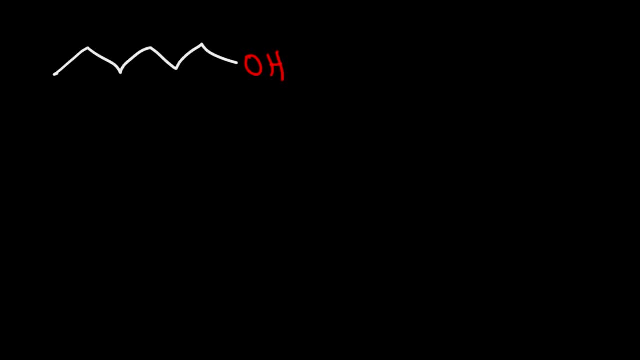 And the chemical shift for the carbon that is attached to the OH is about 63 for this example. Next, we have an amine, And the carbon that is attached to the amine has a chemical shift of about 42.. Now let's compare that to 1-chlorohexane. 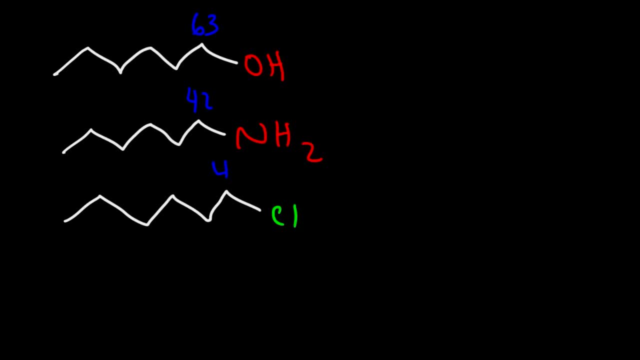 The chemical shift for that carbon with the Cl is 45. And then for 1-bromohexane, The chemical shift is 34. And finally, for 1-iodohexane, The chemical shift is very, very low. 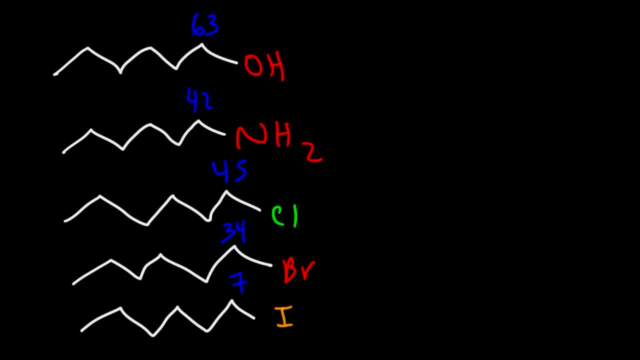 It's 7.. And we can see why that's the case. Iodine has a relatively low electronegativity value compared to the other elements on this board. According to Wikipedia, oxygen has an electronegativity value of 3.44.. 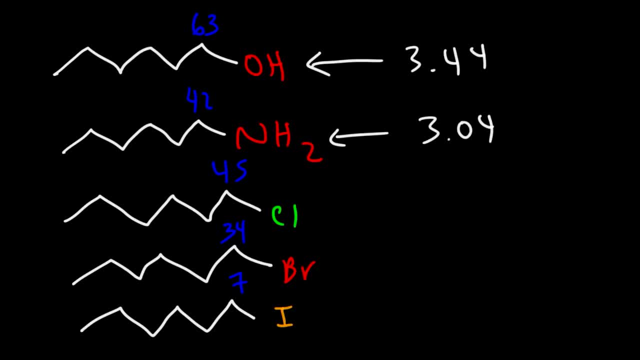 And nitrogen is 3.04.. Chlorine is a little bit more electronegative than nitrogen. According to Wikipedia, it's 3.16.. And bromine is 2.96.. And for iodine it's 2.66.. 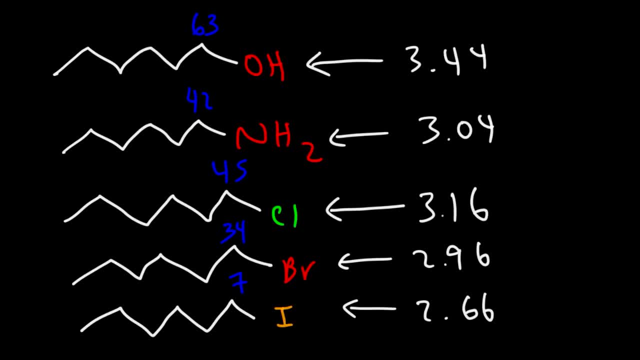 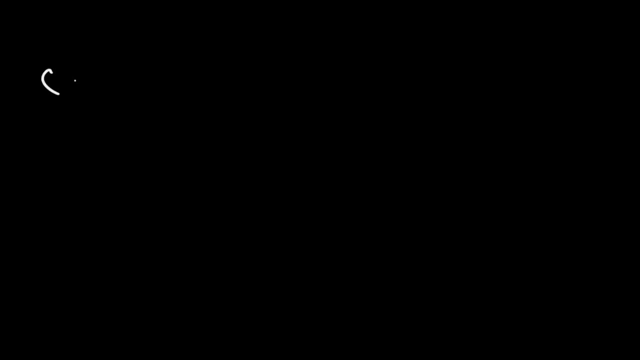 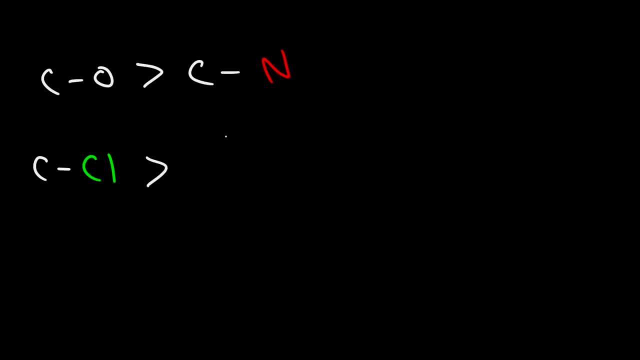 And the Cl bond or the carbon attached to the chlorine bond is a higher chemical shift than the Cl bond. And the Cl bond or the carbon attached to the chlorine bond is a higher chemical shift than the Cl bond Or the carbon attached to the chlorine atom typically has a higher chemical shift than a carbon that's attached to a bromine atom. 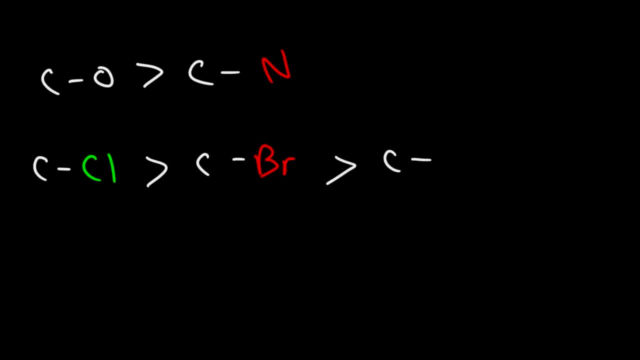 And that usually has a higher chemical shift than a carbon atom attached to an iodine atom. So those are some things that you want to keep in mind. Here's another question for you: Which carbon atom will have a higher chemical shift- Carbon A or carbon B? 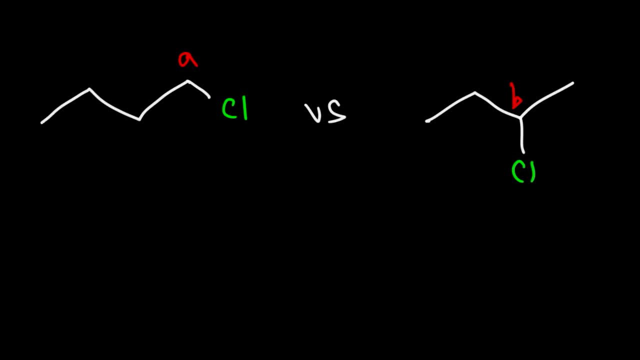 Both of them are attached. What would you say? Well, because the functional group is the same, we need to use the score system to determine the answer. So carbon A is adjacent to a secondary carbon, So we're going to give it a score of 2.. 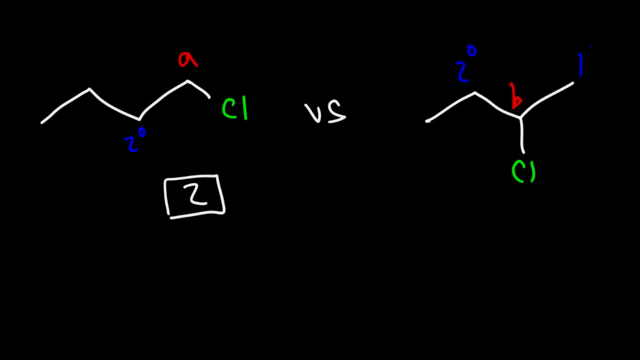 Carbon B is between a secondary and a primary carbon, So we're going to give it a score value of 3.. Because carbon B has a higher score value, it's going to have a higher chemical shift. It turns out that carbon B has a chemical shift of 60, and carbon A has a chemical shift of 45.. 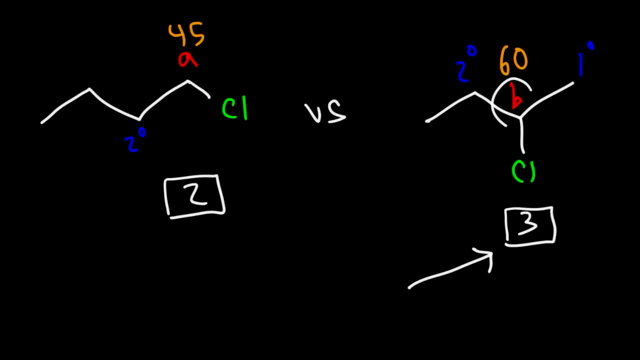 So keep this in mind. When a carbon atom is in the interior of a chain, it usually has a higher chemical shift than the carbon atoms at the end of a chain. So, based on that, which of these two is the higher chemical shift? 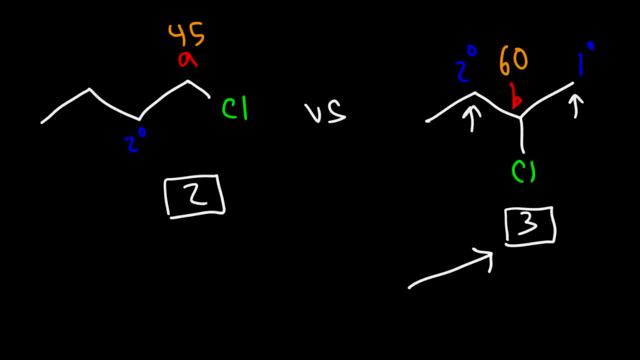 these two carbon atoms is going to have the higher chemical shift. this one is at the end, this one is in the middle. it's going to be the one in the middle. so the primary carbon has a chemical shift of 26. the secondary carbon has a chemical 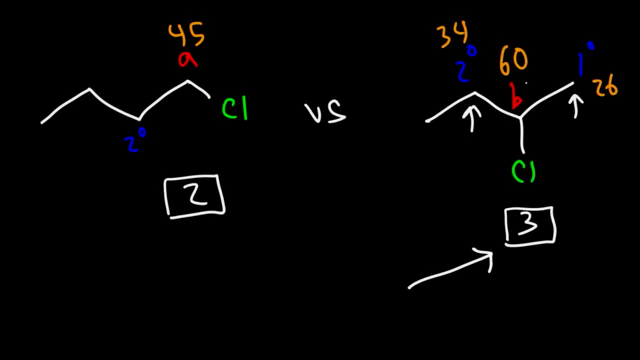 shift of 34 now between the primary carbon on the right and the primary carbon on the left, which one is going to have the higher chemical shift? this one is closer to the carbon with the chlorine atom, so it's going to be more deshielded. in addition, it has a higher score value. the primary carbon on the 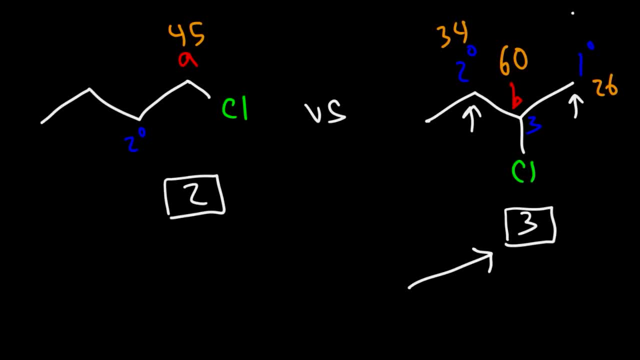 right is adjacent to a tertiary carbon, so it's going to have a score value of three. the primary carbon on the left is adjacent to a secondary carbon, so it's going to have a score value of two. so therefore we should expect that this one is going to have a higher chemical. 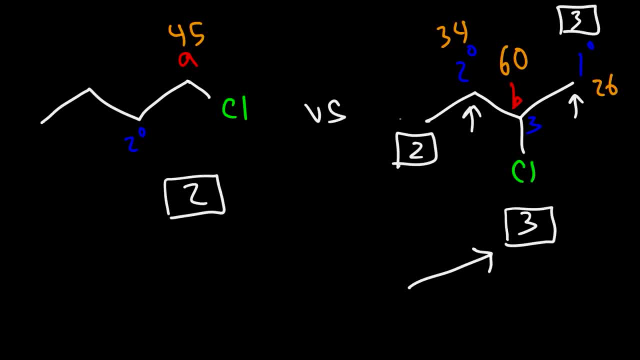 shift and the data supports that. the value for the primary carbon on the left is 11 ppm. so you need to consider two factors: the score value and the proximity to an electronegative atom. in the case of the primary carbon, here it had a higher score value and it was closer. 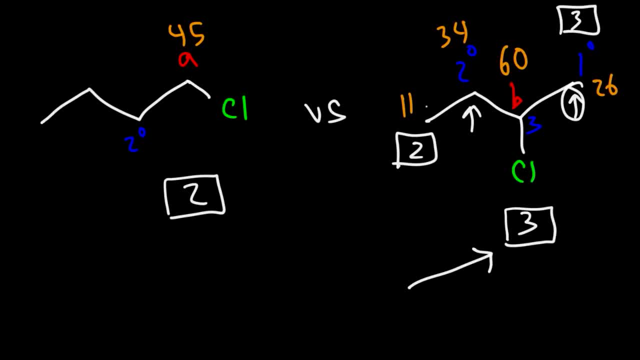 to the primary carbon on the left, so it's going to have a higher score value to the electronegative chlorine atom compared to this carbon, and so both effects favored this carbon, and so we can see why it has a significantly higher chemical shift that the other primary carbon on the left. now let's look. 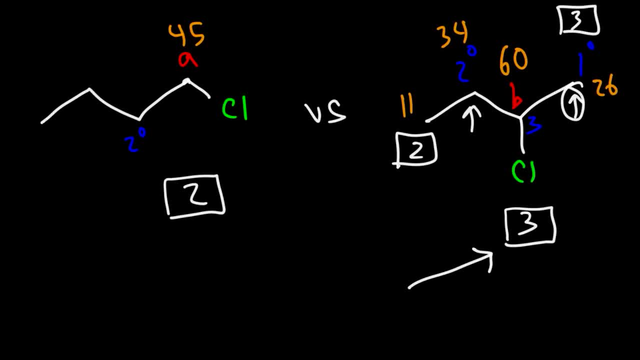 at one chloral butane. let's compare these two carbons. let's call it carbon a and carbon C. carbon a has the chlorine atom, but carbon C has a higher score value. so which one will take priority: the proximity effect to an electronegative atom or the score system? let's calculate. 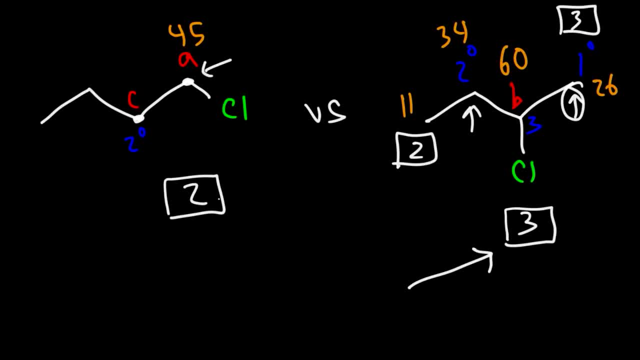 the score values first. so carbon a, we said, has a score value of two. carbon C is adjacent to a secondary and a primary carbon, so we're going to give it a score value of three. so C has the higher score value, but a has the electronegative atom, which one is going to have the higher chemical. 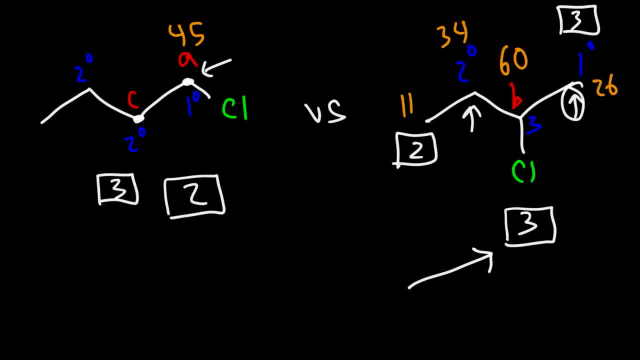 shift, since chlorine is a strong electronegative element for this example, it turns out that the proximity effect is going to win out. the chemical shift for carbon C is 35, for the carbon to the left of that it's 20, and then for the 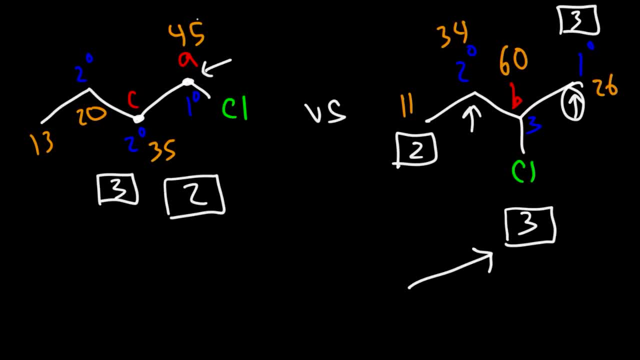 primary carbon on the left is 13, so we could see that the electronegative element had a stronger of impact or a stronger effect on carbon a. now here's another example: instead of one chloral butane, let's use one bromo butane for an example. let's call this carbon a, B, C and D. so which one? 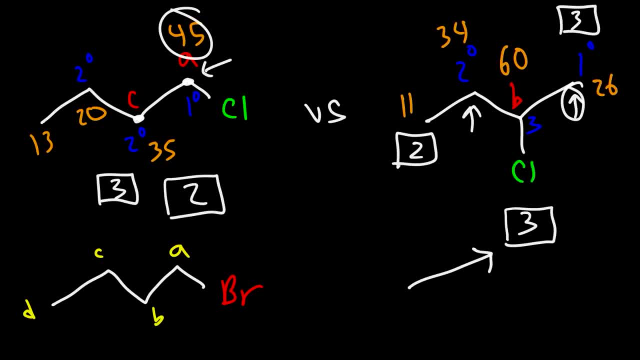 is going to have the higher chemical shift, carbon a or B? which one is going to win out? the proximity to an electronegative out, excuse me on the electronegative element, or carbon B, which has the higher score value? keep in mind: carbon B has a score value of three, just like this one and carbon a. 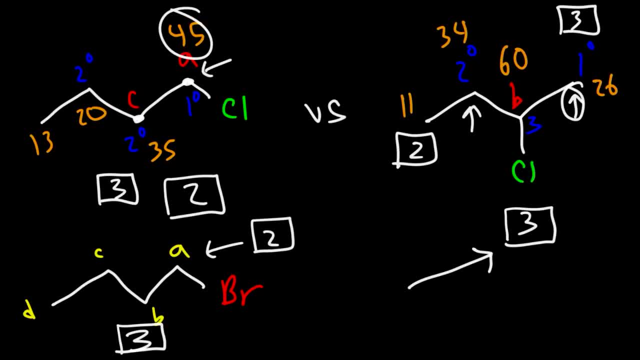 has a score value of two. now, this is going to be a close battle, but it turns out that carbon B is going to win, but not by much. carbon B has a chemical shift of 35, just like this one, but carbon a is 33 because bromine is not as electronegative as chlorine. and so when 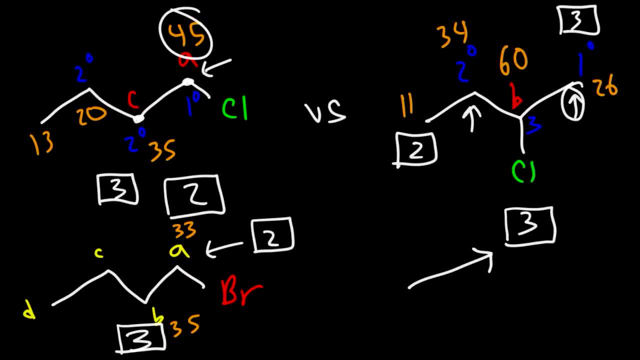 dealing with a proximity effect, you need to think about how, or you need to think about the strength of the electronegative atom. if it's a very powerful electronegative atom, the proximity effect will win. if the atom is not very electronegative, and then the score value may take precedence for. 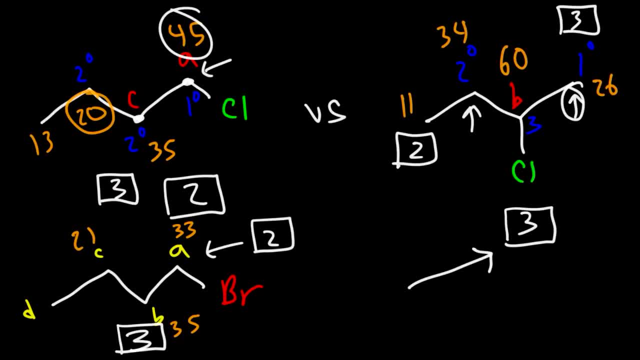 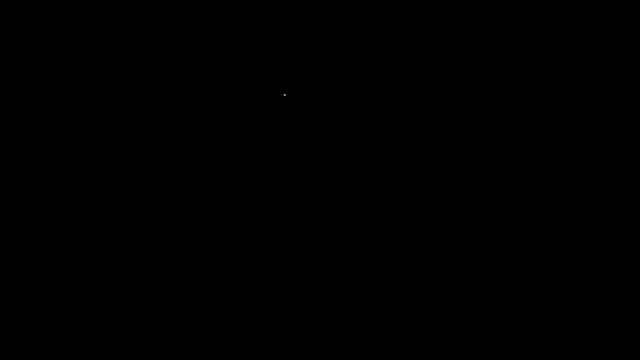 carbon C, the score value is 21, close to this one, and for carbon D, the score value is 13, which is identical to that one. consider this example: let's say we have two iodobutane. which carbon atom will have the higher chemical shift? carbon a or B, because this time both. 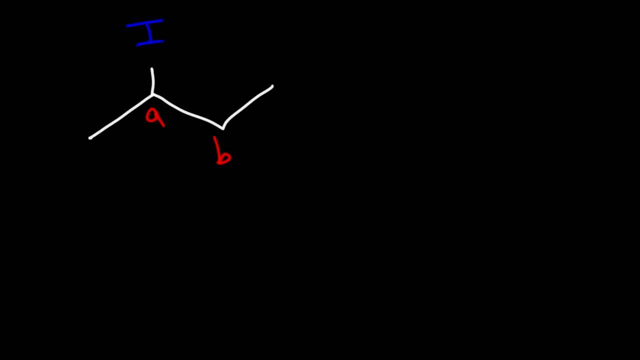 carbon atoms have the same score value. this is primary, secondary, secondary and primary. so analyzing carbon a is adjacent to a primary and a secondary carbon, given a score value of three, and looking at carbon B is adjacent to a secondary and a primary, which also gives it the same. 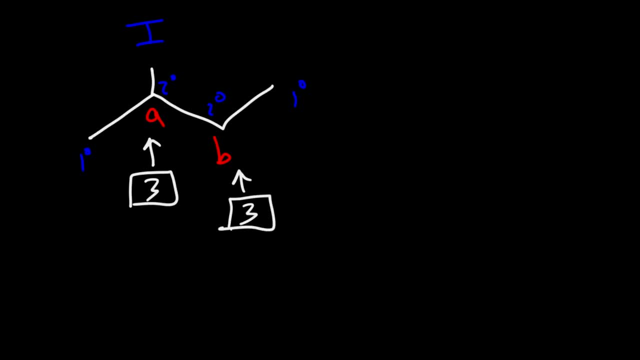 score value. so which one will have the higher chemical shift? it turns out that it's carbon B. carbon a has a chemical shift of 32, carbon B is 36, this is 14 and this is 29, for some reason. now the question is why? why is carbon B higher than carbon a in terms of its? 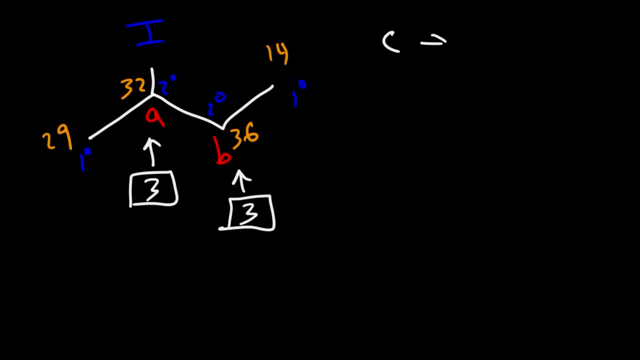 chemical shift. now keep in mind: according to Wikipedia, the electronegativity for carbon is 2.55 and for iodine is 2.66. so iodine is not very electronegative and if we consider the example that we mentioned before, that is of one. 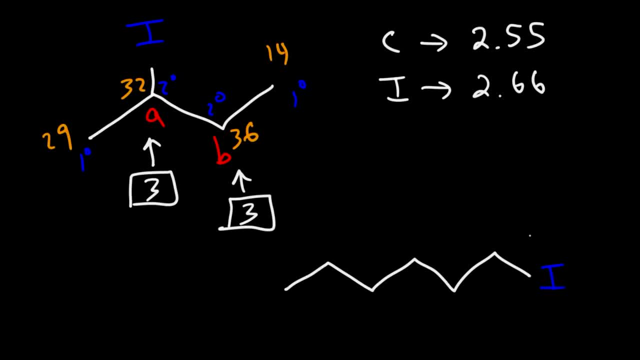 iodohexane. notice the chemical shift of the carbon that has the iodine atom on its 7. the chemical shifts of a typical methyl group is usually between 10 and 15, and those two examples it's 14, but this is unusually lower and so iodine has the 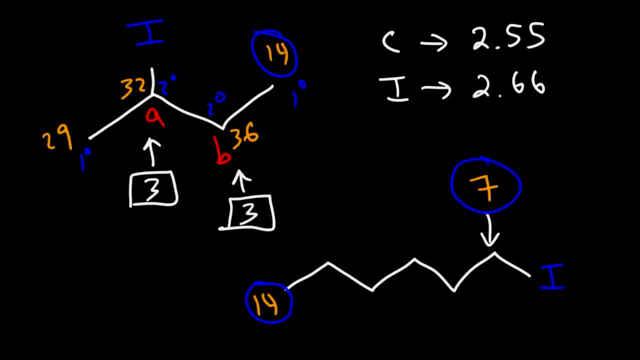 effect of lowering the chemical shift of the carbon that it's attached to, and so this is one reason why the chemical shift of carbon a, which is 32, it's less than the chemical shift of carbon B, which is 36. now let's focus on alcohols. 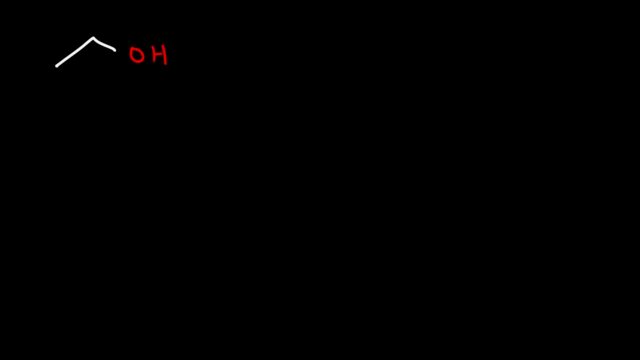 I'm going to give you a list of alcohols and I want you to determine which carbon atoms that are attached to the OH group have a higher chemical shift. so I'm going to write down a few of them. feel free to pause the video or fast-forward it if you want to. 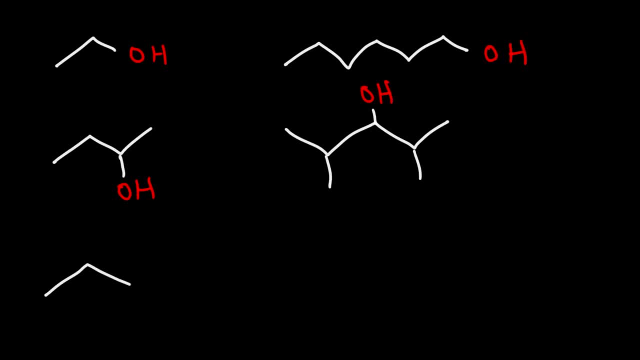 now have two more examples to draw, and then the last one is going to be 3-methyl-3-pentanol. so go ahead and rank each carbon atom. let's call this carbon a, b, c, d, e and f. ethanol and 1-hexanol are primary alcohols. 2-butanol is a secondary alcohol, and this here, that's a 2,4-dimethyl-3-pentanol. that's a secondary alcohol, and the last two are tertiary alcohols. now, tertiary alcohols don't always have the highest chemical shift, and let's see why. so let's 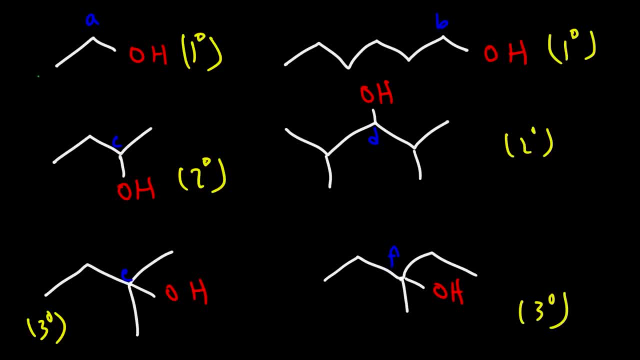 analyze this one first. carbon a is attached to a primary carbon, and so we're going to give it a score of 1. carbon b is attached to a secondary carbon, and so we're going to give it a score of 2. carbon c is adjacent to a secondary and a primary. 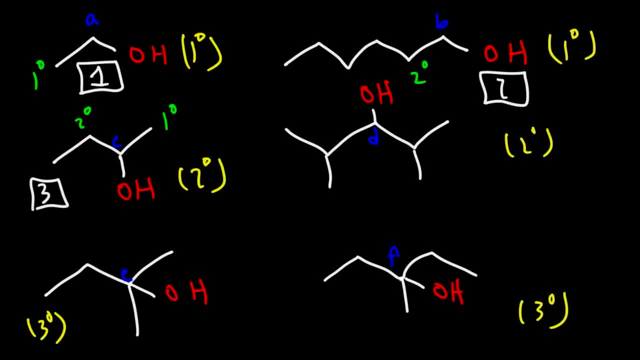 carbon, so we'll give it a score of 3. carbon d is adjacent between two tertiary carbons, and so we're going to give this one a score of 6. carbon e is next to two primary carbons and the secondary, so we're going to give 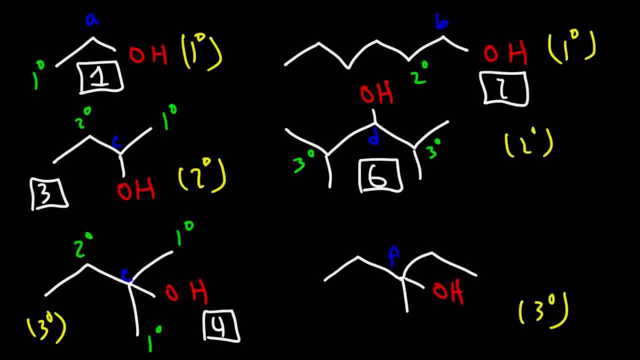 it a score of 4, and carbon f is next to two secondary carbons and a primary one, and so we're going to give it a score of 5. the chemical shift for carbon a is 58. the chemical shift for carbon b- we saw that before- that's 63. 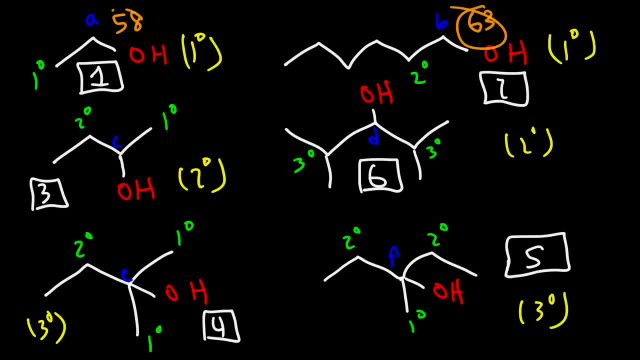 And so notice that this one is higher than this one, even though they're both primary alcohols. since carbon B has the highest score value, Carbon C 2-butanol, that has a chemical shift of 69.. And then for carbon D, so that's this one here that has a very high chemical shift of 82. 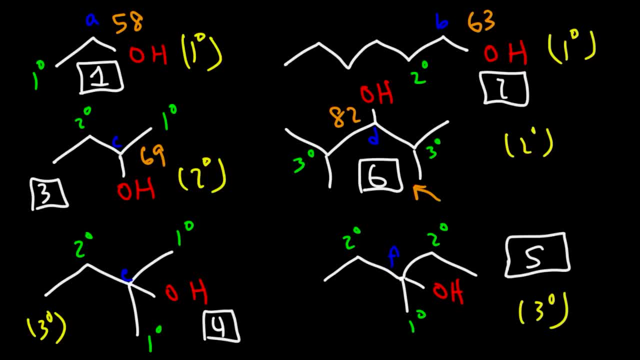 And we can see that because it has a high score value of 6.. Even though both of these are secondary alcohols And then carbon E that has a chemical shift of 71. So it's a little bit more than this one. 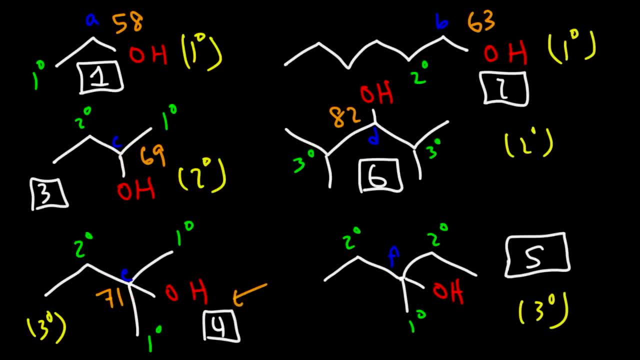 Since this is a score value of 4, that's a score value of 3, but they're pretty close. And carbon F has a score value of 73. And so this is 5 compared to 4, so we expect that this one is higher than this one. 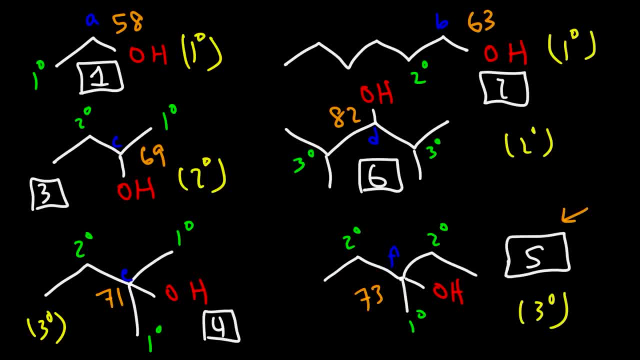 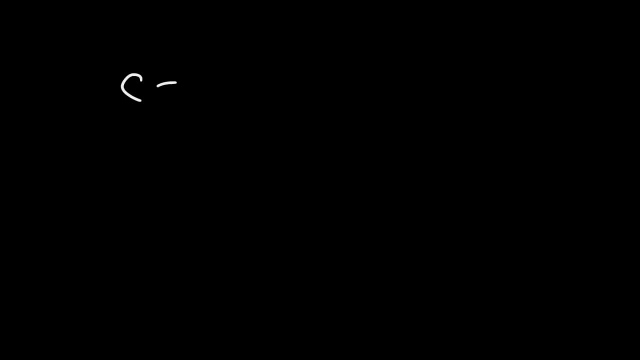 So this is going to be slightly higher. So notice that sometimes a secondary alcohol can have a higher chemical shift than a tertiary alcohol, And so there's many factors that you need to consider. But, in summary, when dealing with alcohols, the carbon that has the oxygen typically has a chemical shift between 50 and 100. 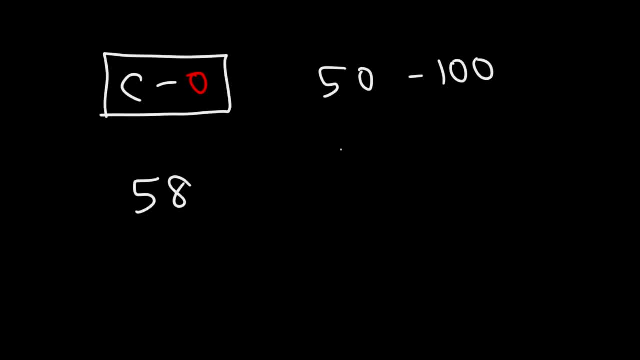 We saw a low value for ethanol, which was 58,, and a high value For the one with a score value of 6,, which was 82. But the carbon with an oxygen will usually be in this range: 50 to 100 parts per million. 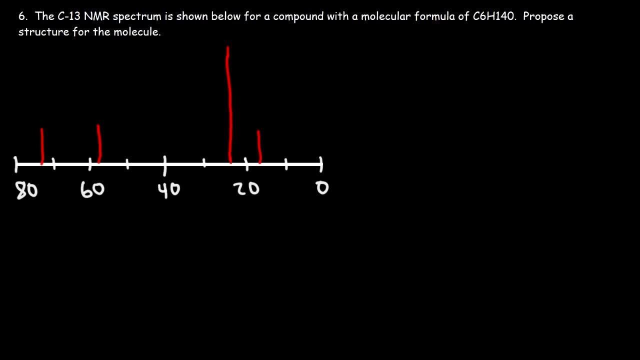 Number 6.. The carbon-13 NMR spectrum is shown below for a compound with a molecular formula of C6H14O. Propose a structure for the molecule. So the first thing I would like to focus on is the functional group. 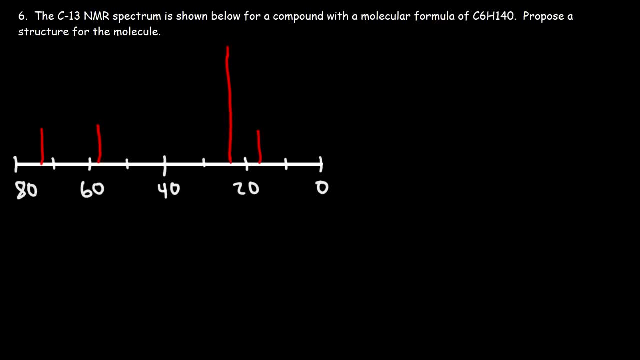 We have an oxygen atom, So this could be an ether, an alcohol It could be. It can't be an ester because that will have two oxygen atoms And it cannot be a carboxylic acid. Now could it be an aldehyde or a ketone? 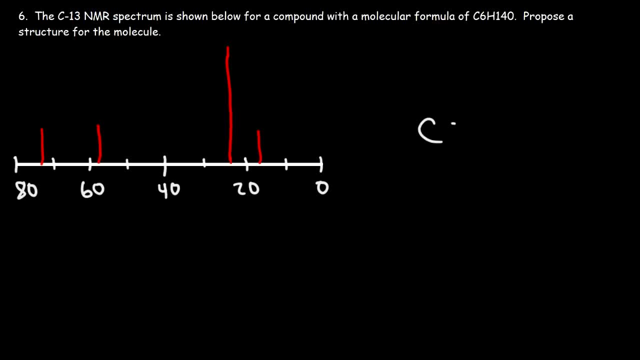 It can't be an aldehyde or a ketone, because we don't have the carbonyl signal between 150 and 220.. So that's out. Now, something we need to take into consideration is the presence of any rings or double bonds. 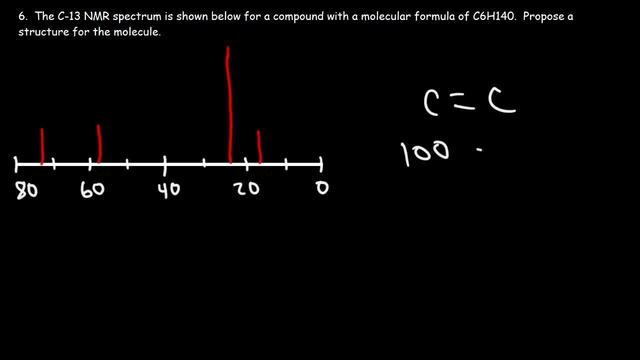 Now a double bond would show up between 100 and 150.. So we don't have that. So we don't have a benzene ring or a double bond. Now there's something else that we could use that will help us to eliminate some possibilities. 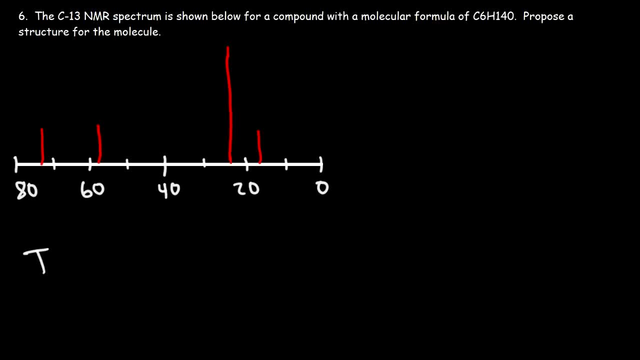 And that is the IHD, The index Of hydrogen deficiency. It's equal to 2N plus 2 minus the number of hydrogen atoms divided by 2.. So N is the number of carbon atoms. We have 6 carbon atoms in this molecule. 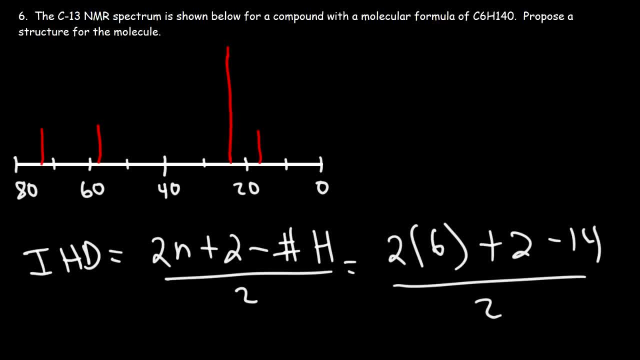 And we have 14 hydrogen atoms. Now, 2 times 6 is 12. And 12 plus 2 is 14.. 14 minus 14 is 0. So the IHD is 0.. In order to have a double bond, the IHD has to be 1.. 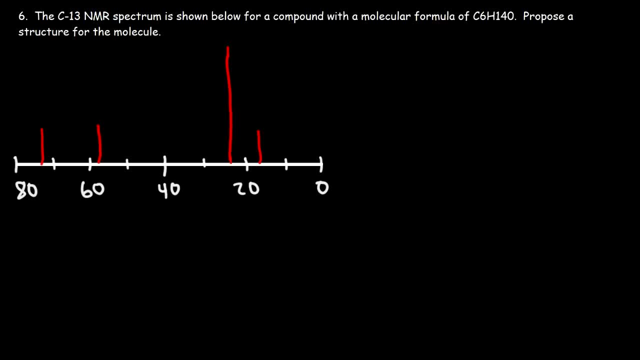 For a ring, the IHD is also 1. And for a triple bond, the IHD is 2.. So, because the IHD is 0, we have no double bonds, no rings and no triple bonds. So all of the carbon atoms that we're dealing with are sp3 carbon atoms. 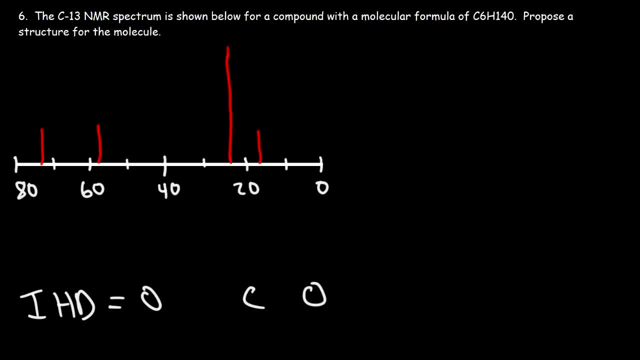 Now, since the IHD is 0. And, as we mentioned before, we have a double bond And, as we mentioned before, there's no signal between 150 and 220.. We don't have any carbonyl groups, So it can't be an ester or an aldehyde or a carboxylic acid or a ketone or an amide. 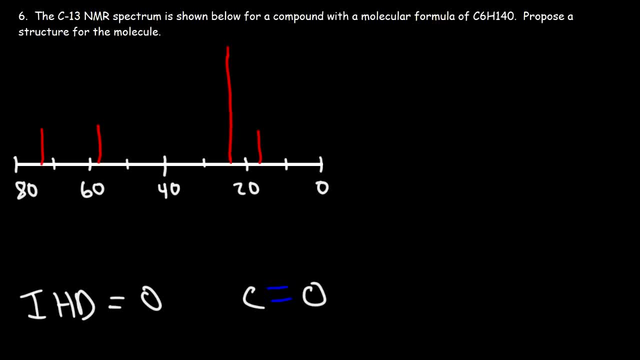 And there's no nitrogen atoms here. So the only other functional groups that contain an oxygen atom are alcohols and ethers. So how do we tell if we have an alcohol or if we have an ether? We have an ether, Because for a CO bond the signal will vary between 50 and 100. 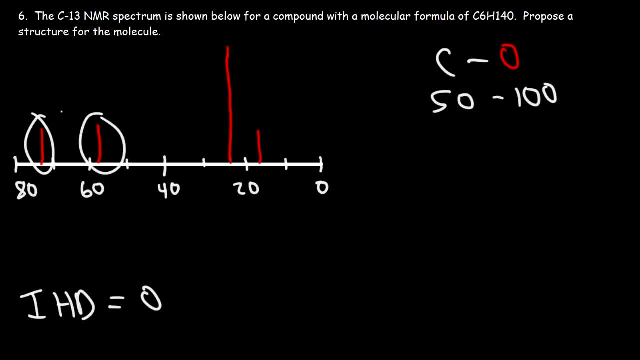 And notice that we have two signals between 50 and 100.. So does that mean it's an alcohol or an ether? So if we have an alcohol, how many CO bonds do we have? An alcohol only contains one: carbon oxygen. But what about an ether? 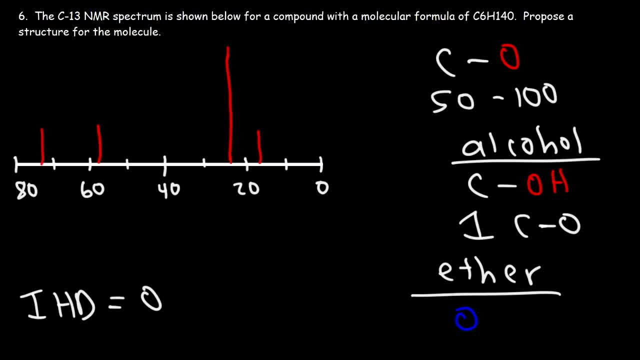 In an ether, the oxygen is between two carbon atoms, So an ether contains two CO bonds. So therefore we should see two signals, between 50 and 100, which we do. So therefore, the functional group that we're dealing with is an ether. 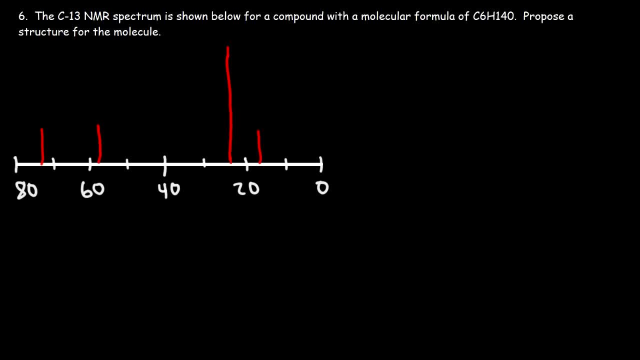 So now, what type of ether do we have? How do we draw the carbon structure around it? So now, the next thing we need to focus on is the number of signals. So we have a total of four signals, but six carbon atoms. 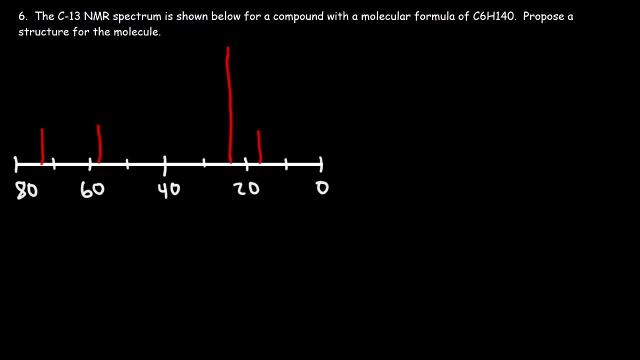 So that means we need to have some equivalent carbon atoms. So let's try the different possible ways in which we can make an ether with six carbon atoms. We could put one carbon on one side and five on the other side And five carbons on the other side. 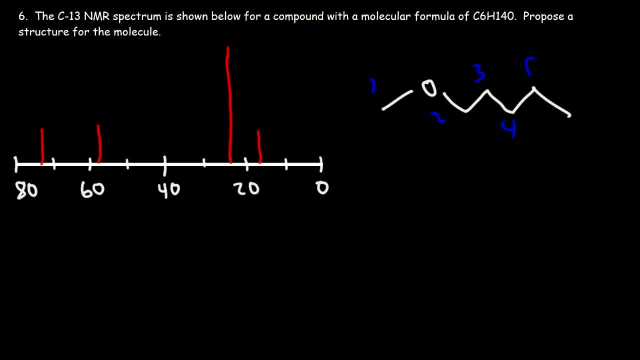 But this would give us a total of six signals, because all carbon atoms are different. If we put, let's say, two carbons on the left, four on the right, this won't work either, because all the carbon atoms are different. 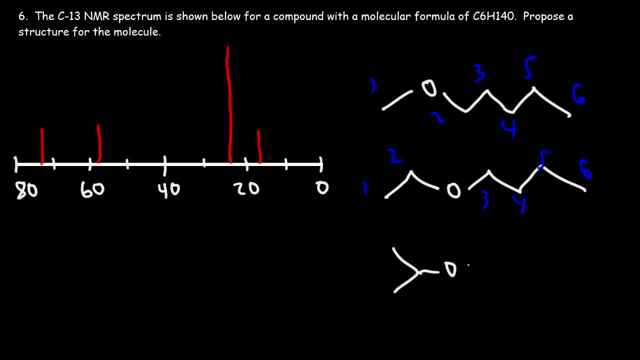 So we could try an isopropyl group, Because by doing so we can get two methyl groups that are identical to each other. These two carbons are the same due to the symmetry of the molecules, And these four methyl groups are identical, giving us a total of two signals. 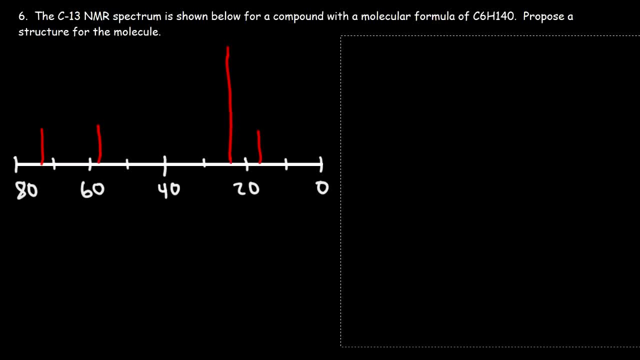 So that's not going to work. Now we can try an isopropyl group on the left and a propyl group on the right, So these two are identical. this is different, And so we have a total of five signals in this example. 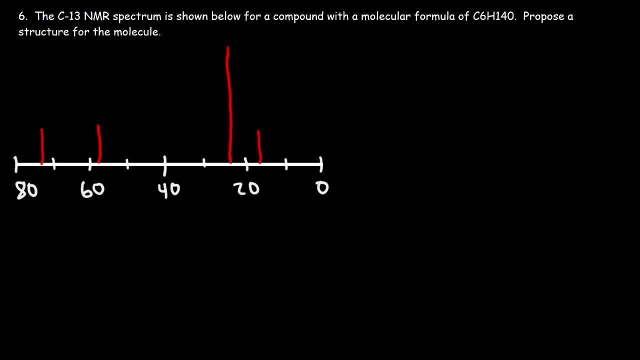 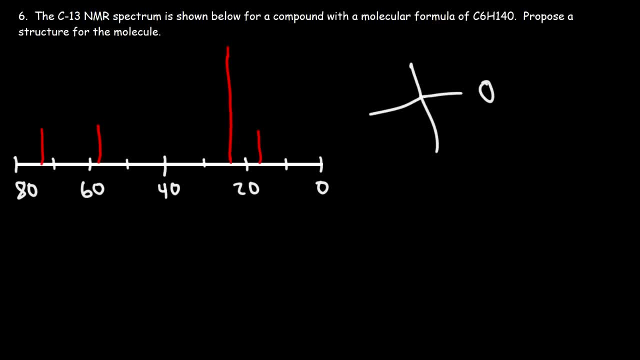 torpedo group. So we have a total of four carbons at this point, so we're going to put two on the right. So now this will be carbon A. the three methyl groups are identical: carbon B, C and D. So now we have a total of four carbon atoms. So 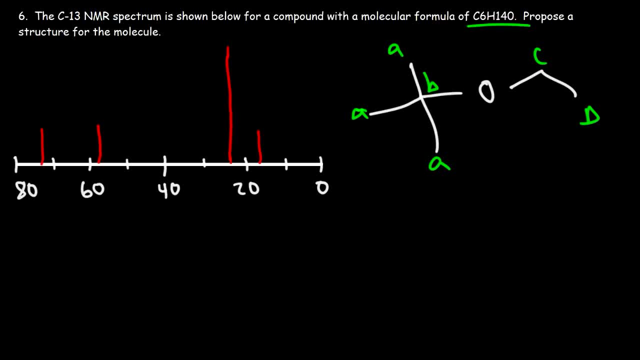 this is the structure that corresponds to this particular molecule. Now let's determine where each signal goes. Now, automatically, we can see that this is the tallest peak. so that's going to correspond to the three methyl groups that we see for signal A. These three carbons will add up to form a large 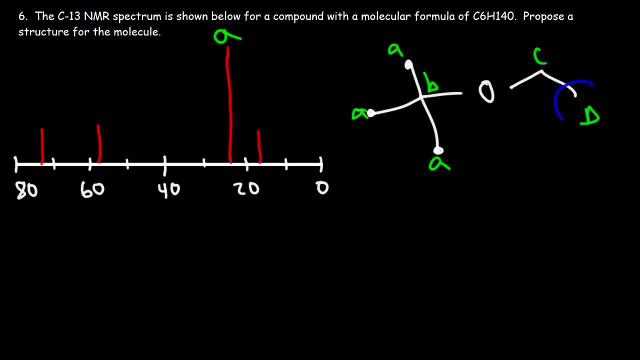 signal. Now this methyl group on the right side must be signal D, which corresponds to a chemical signal A. This is a chemical signal of 16. So this is 16 and this is about 23.. Now carbon A is adjacent to a quaternary carbon, which gives it a score value of 4. Carbon D is 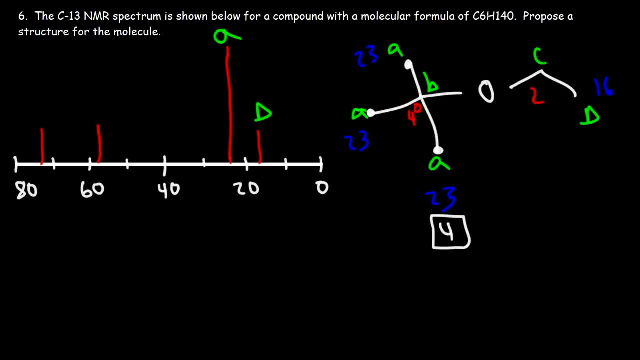 adjacent to a secondary carbon. I mean, that's not a secondary carbon, but that is a primary carbon, and so it has a score value of 1.. So we can see why A has a higher chemical score. Now, carbon B and C are both attached to an oxygen, and so we can see that the 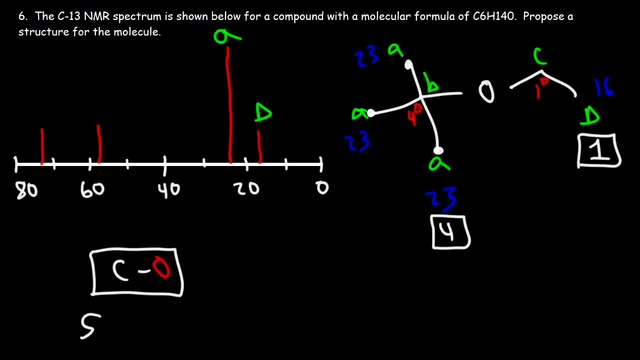 chemical shift is between 50 and 100.. Now which one is going to be higher, B or C? So now let's consider the score value for each. For carbon B, it's adjacent to three primary carbons, and so we're going to. 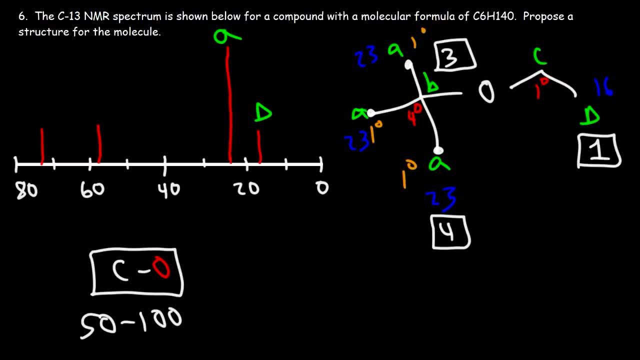 give it a score value of 3.. Carbon C is adjacent to a primary carbon, and so we're going to give it a score value of 1.. So between B and C, B has a higher score value, given that they have the same functional group. So therefore, 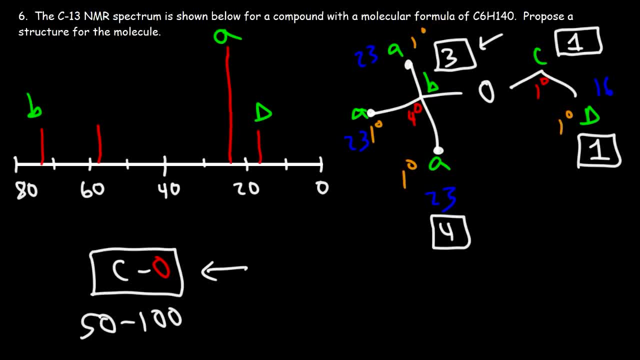 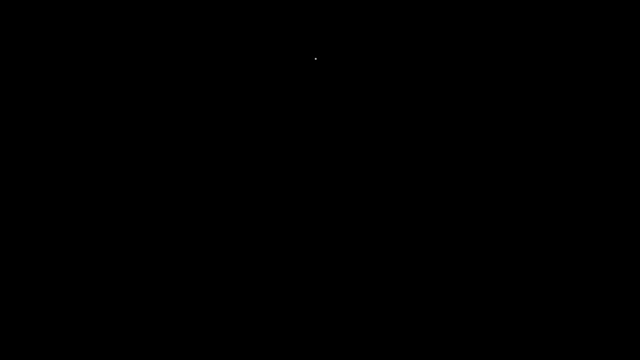 signal B will be the one that's at 73. And signal C is, or carbon C is going to have the signal at 57. And so that's it for this problem. Now, the next functional group that we're going to talk about is the alkyne, the carbon-carbon triple bond. Now in the 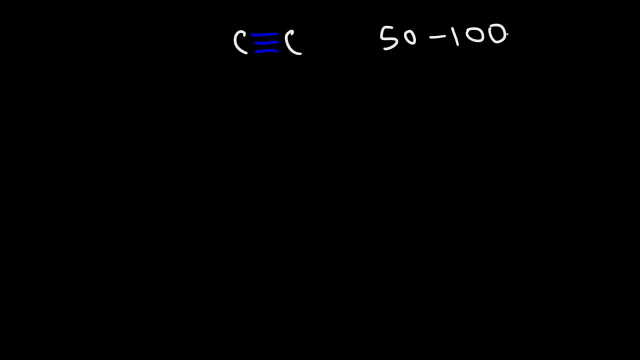 beginning we placed it between a value of 50 and 100, but in practice you'll see that most alkynes fall between 70 and 100.. Now let's work on some examples. Actually, I'm going to draw this out. So here we have 2-butyne and, due to the 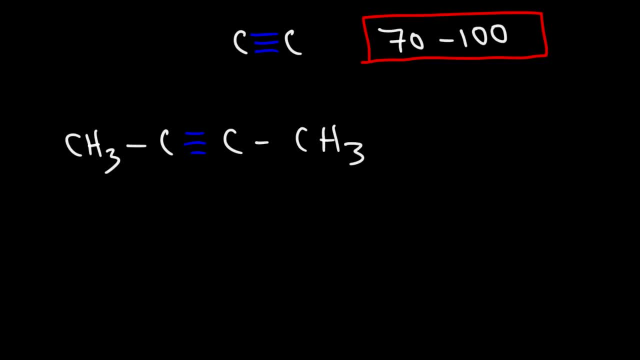 symmetry of this molecule. there's going to be two signals. It turns out that the signal for the carbon atom, that's part of the triple bond, is 75. But what do you think the signal is going to be for the methyl group? Now, most methyl groups that we've seen so far are usually around 10.. We've seen 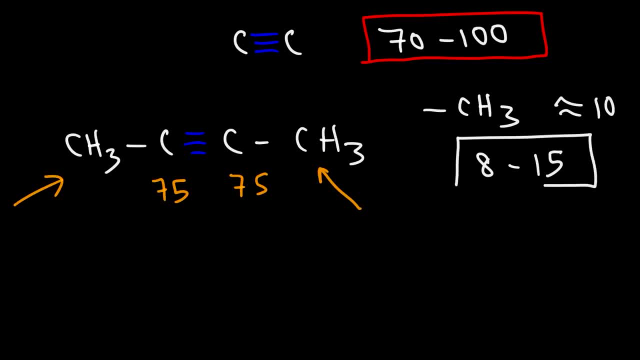 them vary between 8 to 15,. if there's nothing special around it Now, this is usually the case. However, there were some exceptions where a methyl group was attached to a tertiary carbon, and we've seen values as high as 19,, 21, or 23.. But most methyl groups. usually it's around. I guess we could say 10 to 20.. Maybe that's a better range, But the methyl group that is close to an alkyne, that's one carbon away from it. it's actually much less. In this example it's. 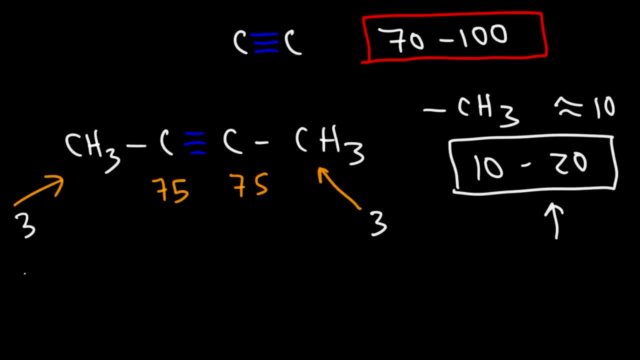 three, And so what you need to keep in mind is that the carbon atom, which we'll call the alpha carbon- that is basically one carbon per second- away from the alkyne functional group. those carbon atoms tend to be lower than normal. The alkyne functional group has the effect of lowering the chemical 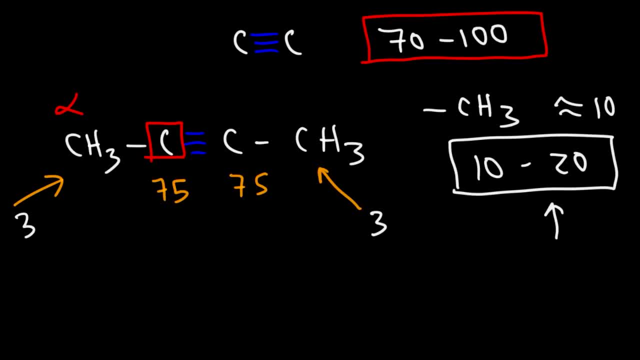 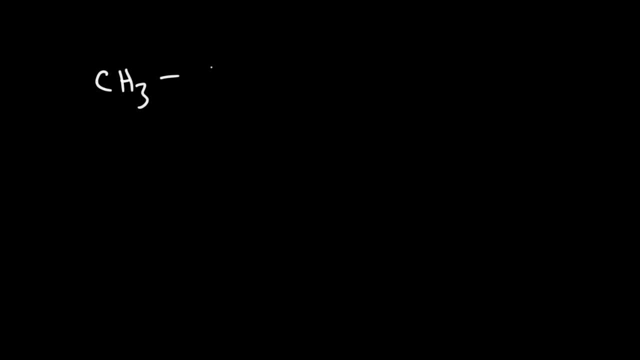 shift of the adjacent carbon atom, And we're going to see that in a few upcoming examples. So let's consider the example of 2-pentine. So let's call this carbon A, B, C, d and E, So there's a total of five signals. So 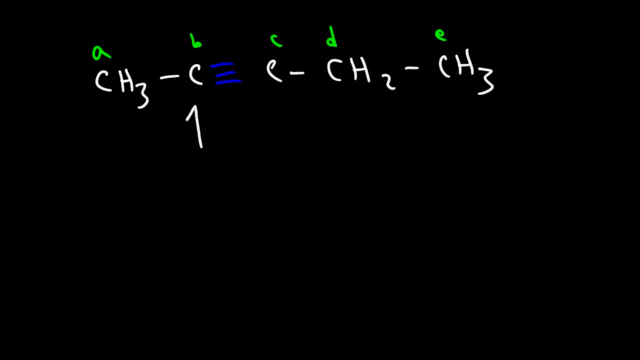 which carbon will have the higher chemical shift: Carbon B or carbon C. Now they're part of the same functional group, so the only difference that we can take advantage of is the score system. Carbon B is the adjacent between a primary carbon and a secondary carbon, So we're going to give it a score value of 3.. 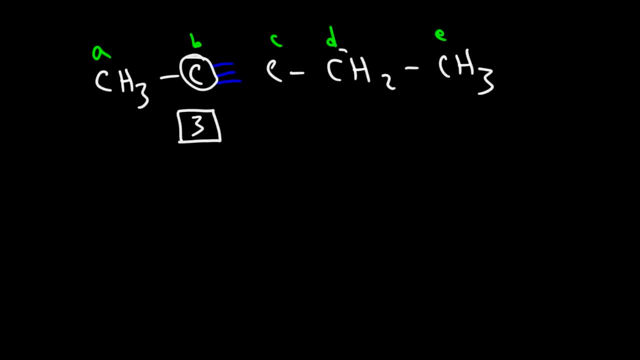 Carbon C is between a secondary carbon and another secondary carbon, So we're going to give it a score value of 4.. So, based on that, we're going to say that carbon C has the higher chemical shift which it does, And so the chemical shift for carbon C is 80.. For carbon B it's 75.. 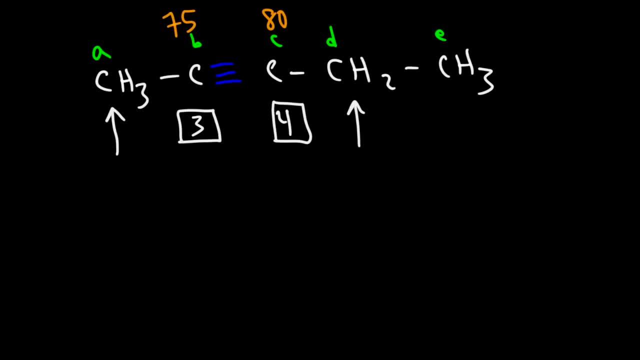 Now, what about between carbon A and D? They're both next to the same functional group, the alkyne. They're one carbon away from it. So in terms of proximity, it's the same. So in this case, because all factors are equal, 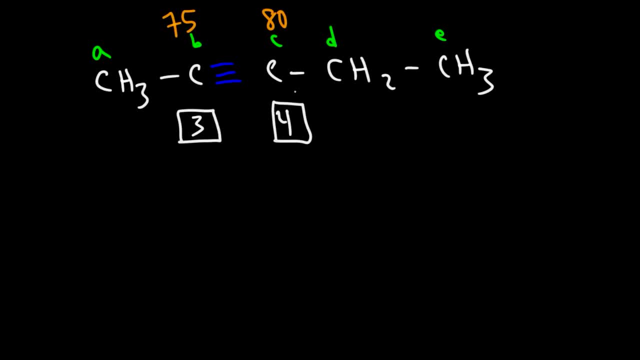 we could use the score system to see if there's a difference. Carbon A is next to a secondary carbon, So let's give it a score value of 2.. Carbon D is between a secondary and a primary, So we're going to give it a score value of 2.. So we're going to give it a score value of 2.. 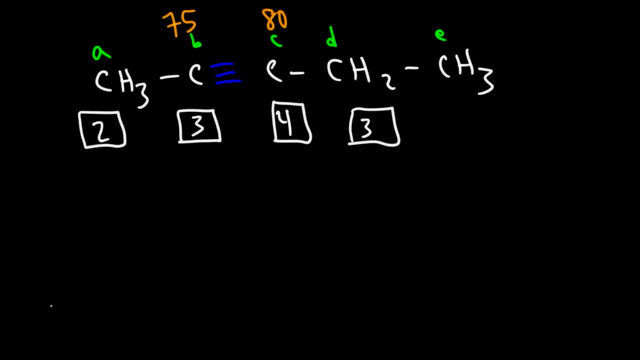 So let's give it a score value of 3.. It turns out that the chemical shift of the methyl group on carbon A, it's 3,, just like in the case of 2-butyne. But the methylene group corresponding to carbon D has a chemical shift of 13.. And so we can see that when everything 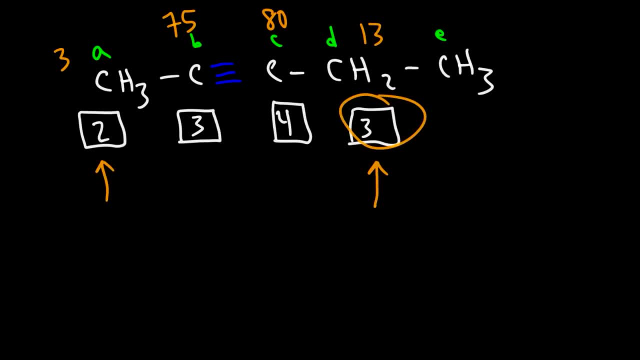 else is equal. the one with the higher score value usually has the higher chemical shift. Now let's compare carbons D and E together. Which one will have the higher chemical shift? Now, carbon E is adjacent to a secondary carbon, so it has a score value of 2.. 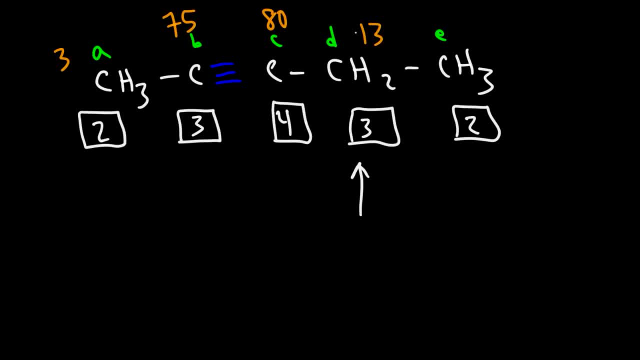 So you might be inclined to think that carbon D should have the higher chemical shift because it has a higher score value. Even though the score value is a factor, it's not the only factor, So in this case it may not always give you the best answer. 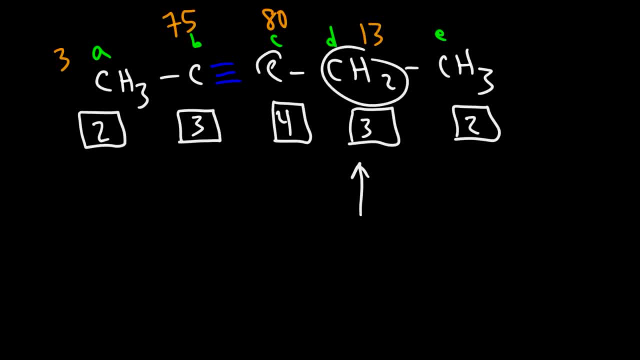 We do have to consider the fact that carbon D is adjacent to the alkyne, which has the effect of lowering the chemical shift. So sometimes this carbon will be lower than this one, And for this example, that's what's going to happen. Carbon E has a chemical shift of 14.. 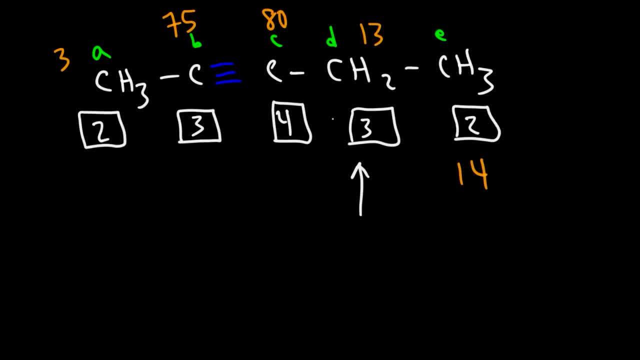 So it's a little bit more than carbon D. So because this is a lower chemical shift, it's going to have a lower score value. So if this is next to an alkyne, the chemical shift is lower. It's been lowered to the point where it's less than carbon E. 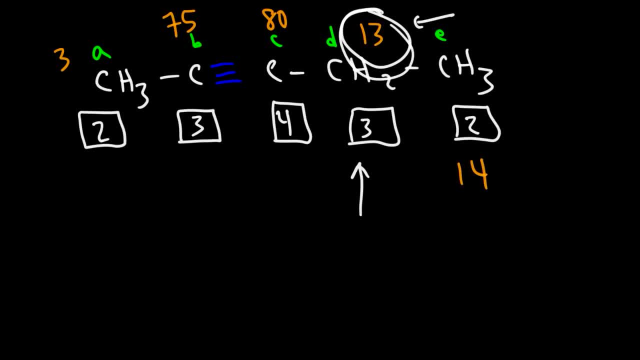 Sometimes this might be a little bit more, Sometimes they might be the same. There's a lot of factors to consider, But just know that the carbon that's next to the alkyne will be lower than usual. Now let's consider an example with a carbon E. 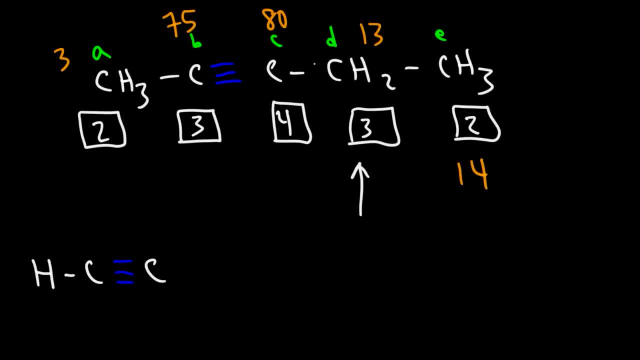 A terminal alkyne as opposed to an internal alkyne. Let's see what we can learn from it. So here we have one hex sign. Let's call this carbon A, B, C, D, E and F. So which one is going to have the higher chemical shift, A or B? 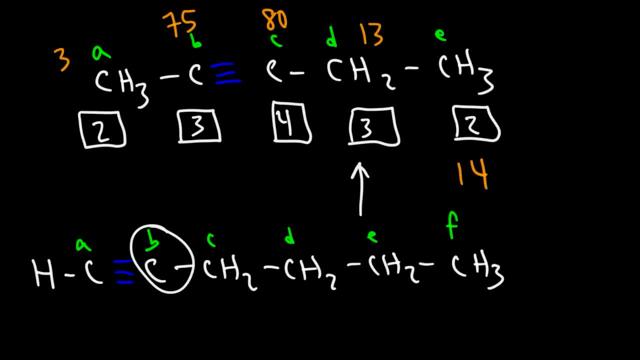 So the carbon atom that is in the middle of the chain usually has the higher chemical shift than the one at the end. There are some exceptions, though, as in the case of that one, But if you look at the score value, the score value for this one is going to be 2, because it's adjacent to a secondary carbon. 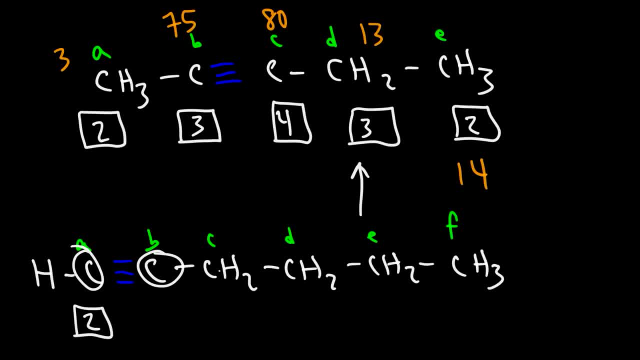 The score value for carbon B is going to be 1 plus 2, which is 3.. It's adjacent to a primary and a secondary carbon, So B should have a higher chemical shift, And it does. The chemical shift for carbon B is 85.. For A, it's 68.. Now, something that I want you to pay attention to is that for internal alkynes, the chemical shift of the carbon atoms are fairly close, But for terminal alkynes they're not as close As you can see. 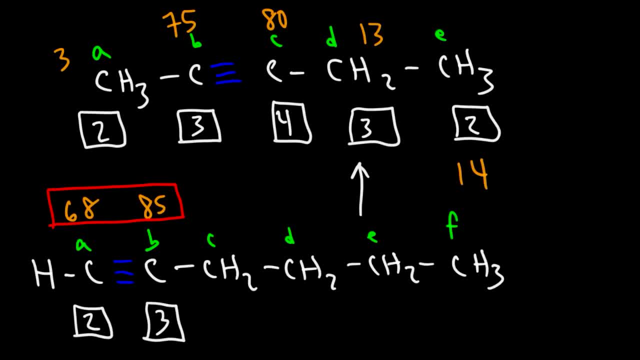 they're further apart, And so knowing that that can help you to distinguish an internal alkyne from a terminal alkyne. Now, looking at the four remaining carbon atoms, which one will have the highest chemical shift and which ones will have the lowest chemical shift. 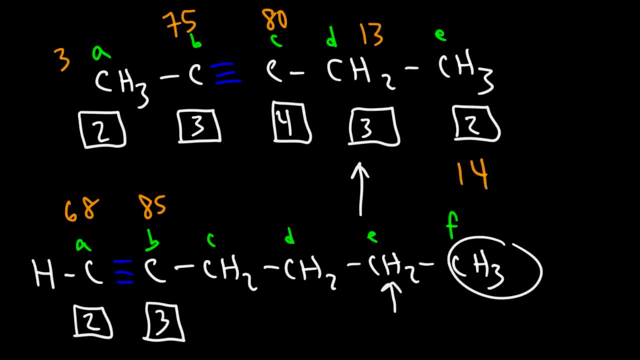 So, starting with carbon F, it's adjacent to a secondary carbon, So that's a score value of 2.. For carbon E, it's between a primary and a secondary carbon, So 2 plus 1 is 3.. And for carbon D it's between two secondary carbons. 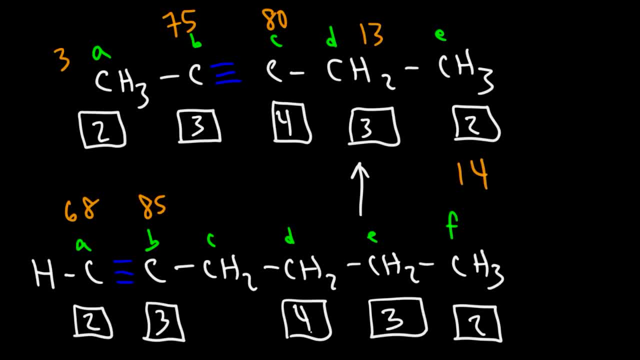 So that's going to give it a score of 4.. And for carbon C it's between two secondary carbons as well, So that will also give it a score of 4.. So between E and F, which one is going to have the higher chemical shift? 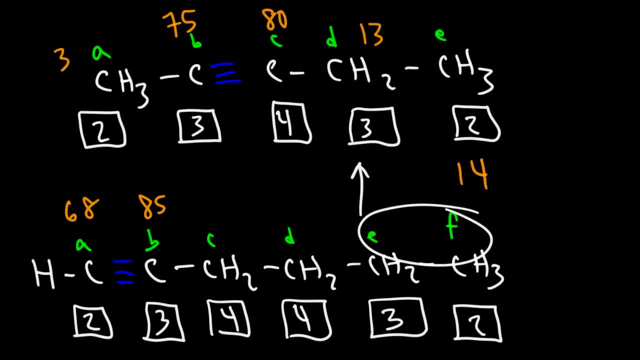 Now, none of these are one carbon away from the alkyne, so we could use the score system. E is going to be higher than F, and it is. The value for E is 22, and for carbon F it's 14.. 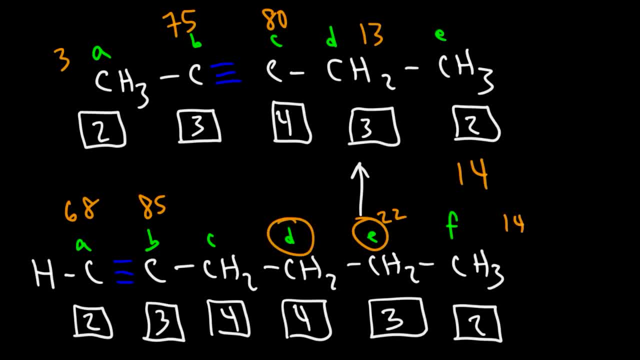 Now between D and E. none of them are one carbon away from the alkyne group, So D has a higher score, D is going to have a higher chemical shift and it's 31.. Now between C and D, the score value is the same. 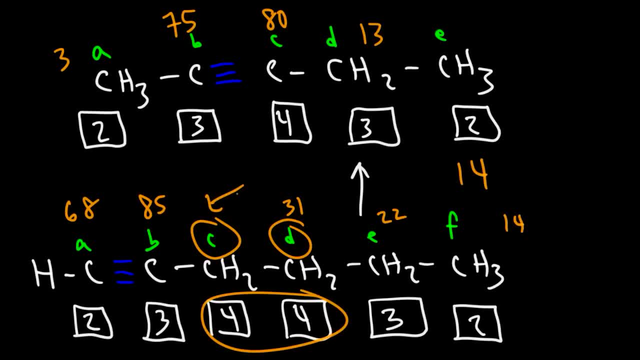 But C is one carbon away from the alkyne. Therefore, C is going to be lower than D And the signal for C is 18.. So, as you can see, this is a significant drop compared to 31. Number 7.. 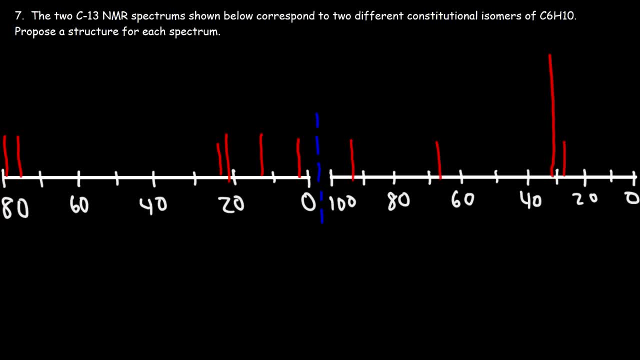 The two carbon-13 NMR spectrums shown below correspond to two different constitutional isomers of C6H10.. Propose a structure for each. Now let's begin by calculating the IHD, the index of hydrogen deficiency. So the formula is 2N plus 2 minus the number of hydrogen atoms divided by 2.. 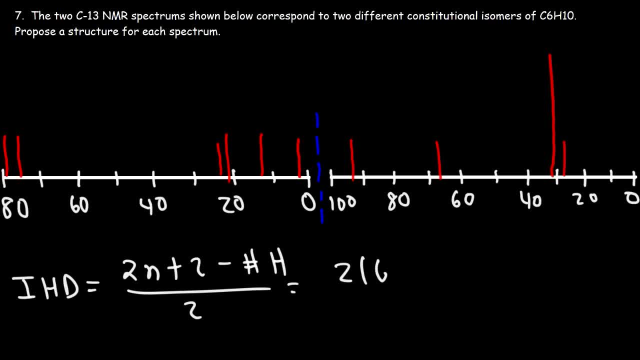 So in C6H10, there's a total of 6 carbon atoms and we have 10 hydrogen atoms. Now, 2 times 6 is 12, plus 2, that's 14.. 14 minus 10 is 4.. 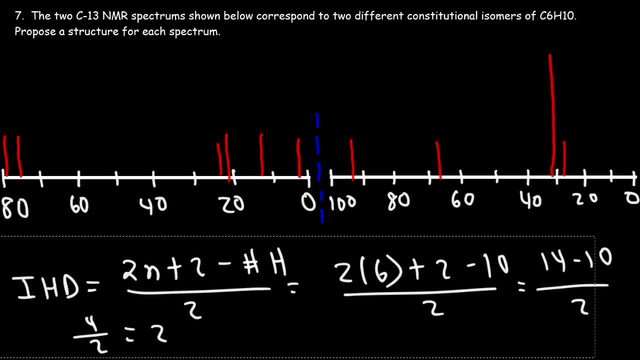 And 4 divided by 2 is 2.. So the IHD is 2.. Now keep in mind: a double bond has an IHD of 1.. A triple bond has an IHD of 2. And a ring has an IHD of 1.. 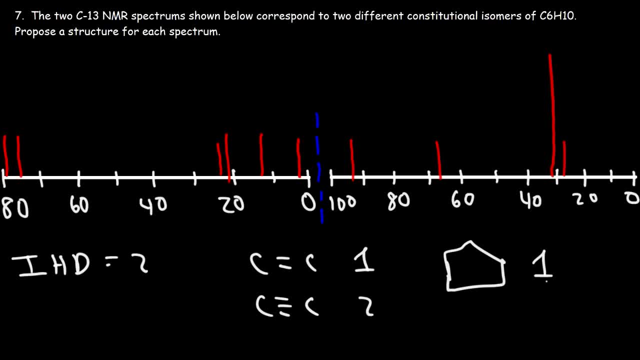 So this could be two rings, It could be two double bonds, It could be a double bond and a ring or one triple bond. So those are the possibilities. Now notice that we have a signal between 70 and 80.. 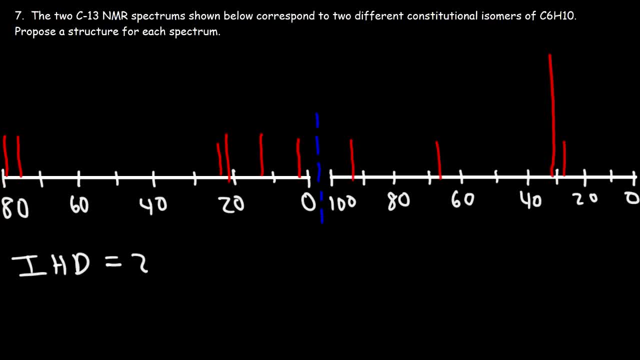 We have two of them, And so this can't be a double bond, because the alkenes they exist between 100 and 150.. So that is not going to be the situation here. Now a ring won't give us a signal between 70 and 80.. 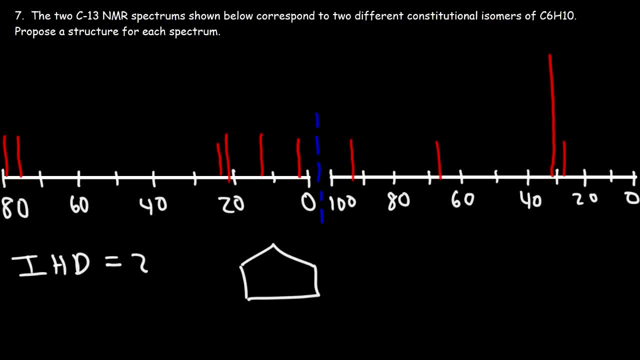 And we don't have a double bond. We don't have any oxygen atoms, So there's no ethers or alcohols. The only possibility is the alkyne. Now, looking at this structure, would you say this is a terminal alkyne or an internal alkyne? 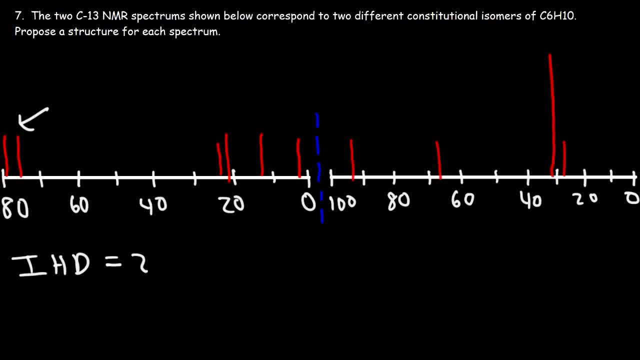 So these two peaks are close to each other. So therefore, we're going to say that this is going to represent an internal alkyne. Now, these two peaks, We have a terminal alkyne. We have one that's a little bit less than 70 and one that's 90.. 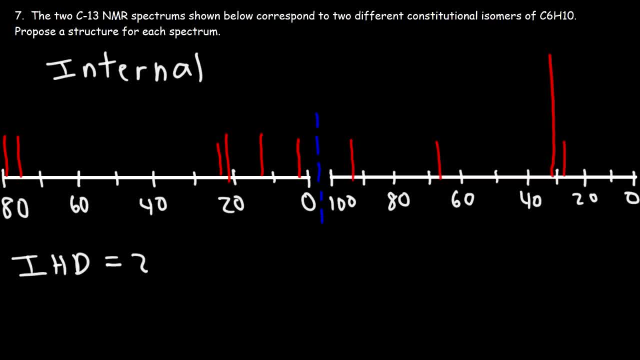 But notice how far apart they are. So because they're so far apart, this is going to represent a terminal alkyne. So alkynes can range between 50 and 100.. But, as we said before, typically it's 70 to 100. 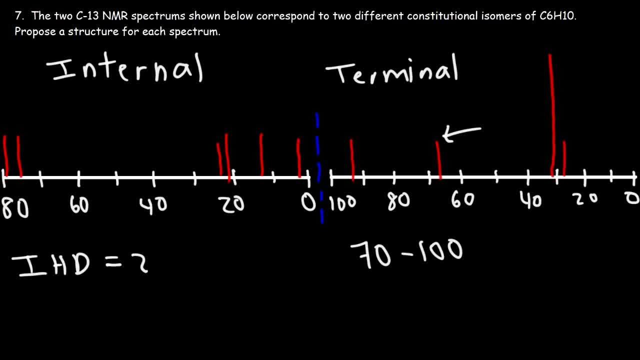 But sometimes you'll see some that are less than 70.. Now, focusing on this spectrum on the left side, notice that we have a total of six signals. So therefore we can't have any equivalent carbons And it has to be an internal alkyne. 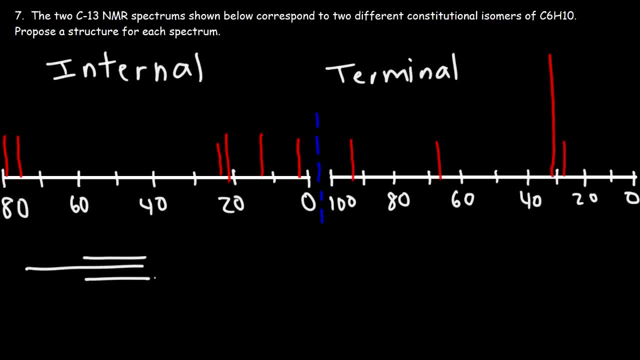 So let's draw six carbon atoms where the triple bond is in the middle. So we have to put at least one carbon atom on the left of the triple bond, So we could put the other three on the right. So this is one possibility. 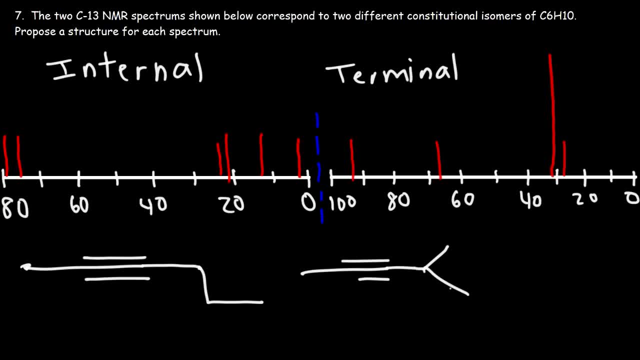 Now notice what happens if we try to branch it. We'll get this possibility. Or let's say, if we put two carbons- Let me start with the triple bond. Let's say if we put two carbons on the left and two carbons on the right. 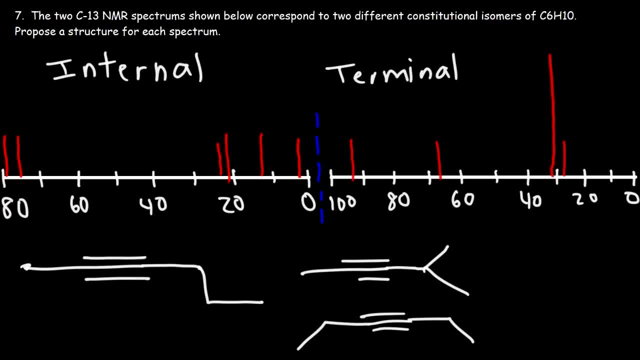 So, due to symmetry, we're going to have equivalent carbons. This would be the first signal. This is the second, third, fourth, fifth signal. So that's out. We don't have five signals. These two are the same. 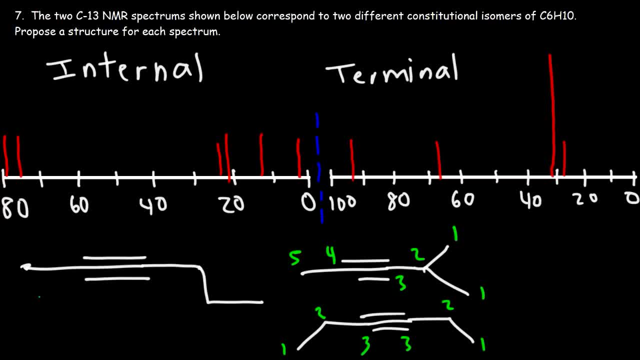 Those two are the same, So this will give us three signals. This would be one, two, three, four, five, six. All of them are different, And so this could work. We can't really use the tert-butyl group because, for one thing, we don't have a tall peak here. 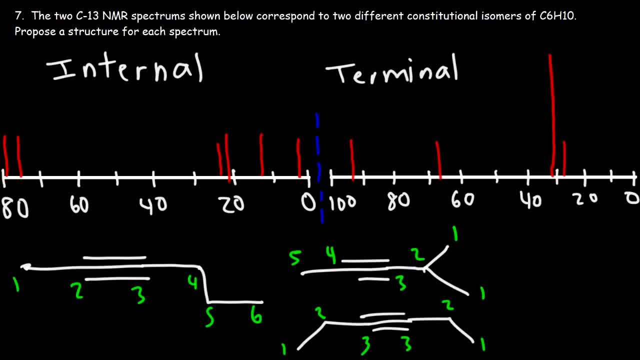 So that's another indication that we don't have any equivalent carbon atoms. Because these two are equivalent, we should expect a tall peak, but there is none. So right now this is the only best possibility that we can come up with for a six-carbon alkyne. 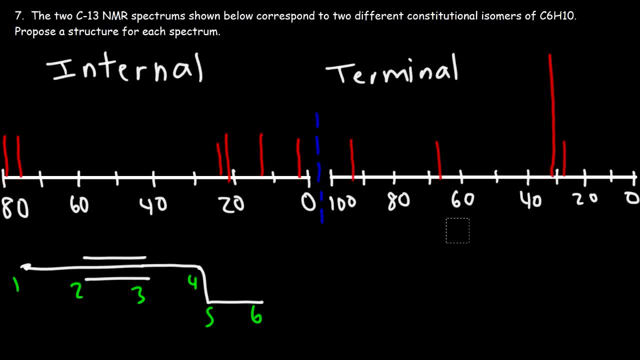 And it turns out that this is indeed the structure for the spectrum on the left. Now let me give you the values. that corresponds to the signals that we see on the graph. So this is three. This signal is 14.. The next one is 21, and then 23.. 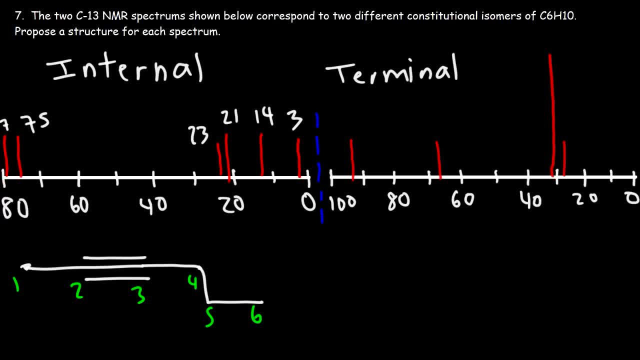 And we have one at 75. And the last one is at 79. Let me see if I can space this. So, looking at carbons two and three, we know it has to be these two values at 75 and 79.. 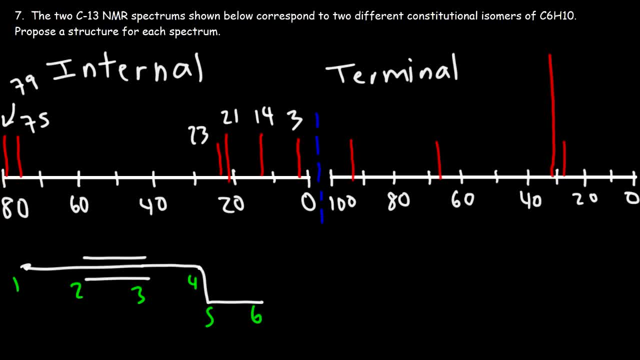 So which one is going to be the one at 75, and which one is the one at 79?? So carbon two is between a primary and a secondary carbon, so it has a score value of three. Carbon three is between two secondary carbons, so it has a score value of four. 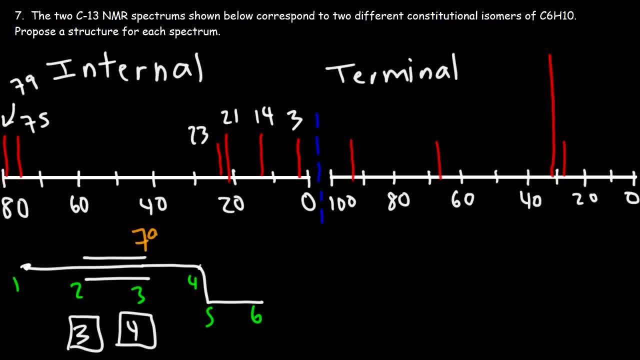 So therefore carbon three is the one that has the higher chemical shift, at 79.. Carbon two has the lower one. Now carbon one. we saw multiple examples where a methyl group attached to an alkyne has a chemical shift of three. 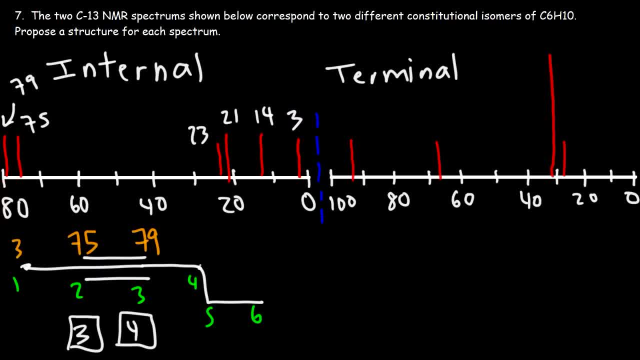 And so this is going to be the same in this example. So that's pretty consistent. Now, what about carbons four, five and six? Carbon four has a score value of four because it's adjacent to two secondary carbons. 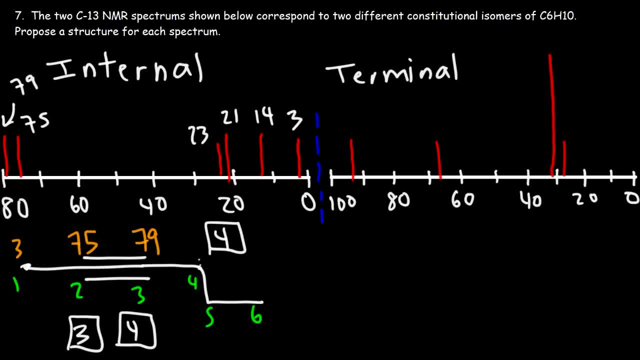 Carbon five has a score value of three because it's next to a secondary and a primary, And carbon six is adjacent to a secondary carbon, given it a score value of two. So what do you think the signal will be for carbon six? 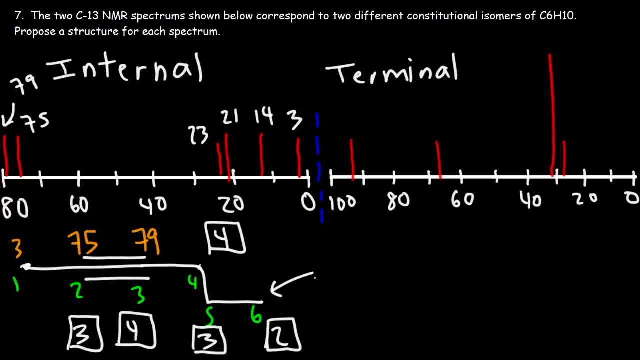 Based on the many examples that we've covered so far, when a methyl group is next to, let's say, a CH2,, typically the signal is around 10 to 15.. And this methyl group is far away from the alkyne, so it's not really affected by it. 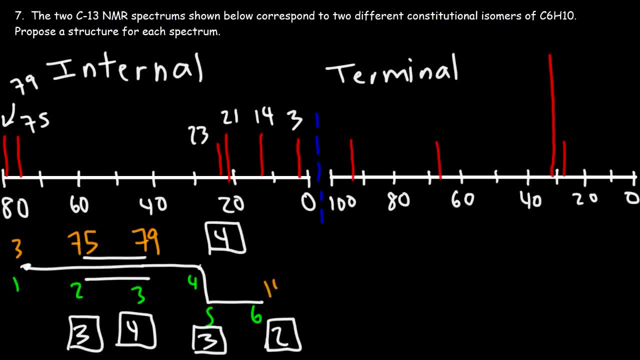 So thus, the signal at 14 is reasonably attached to carbon six, And it turns out that it is Now, between carbons four and five, which one will go, which one will be 21 and which one will be 23?. 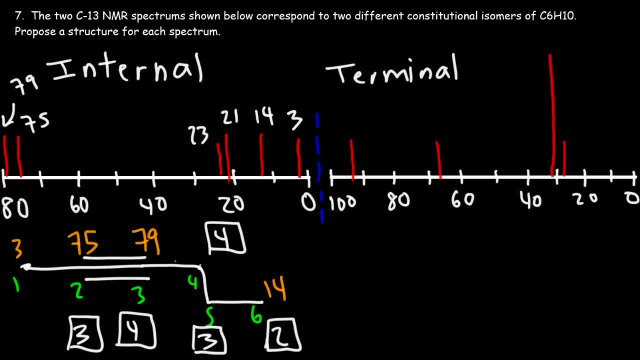 Now we do expect a drop at carbon four, And so it turns out that this one is going to be at 21, and carbon five is going to be at 23.. They're pretty close, though, even though carbon four has a higher score value. 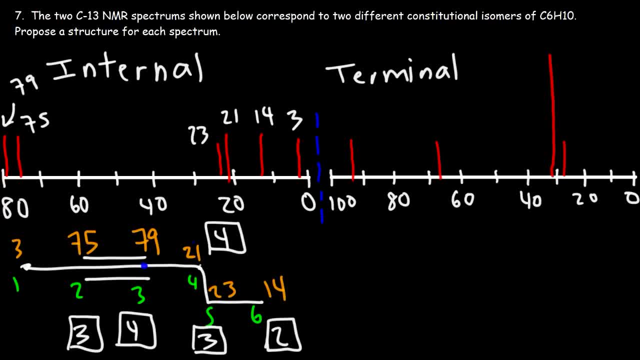 But because it's adjacent to the alkyne, we see the drop in the signal, So it's a little bit lower than this one. Now let's move on to the structure on the right side. So we have a terminal alkyne, which means that we need to put the triple bond at the end. 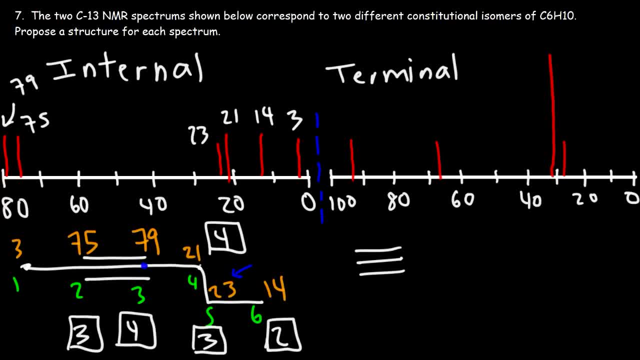 And there's only four signals. So we can maybe put an isopropyl group- one, two, three, four, five, six carbons, But this will give us five signals. So therefore we have to use a turbidor group. 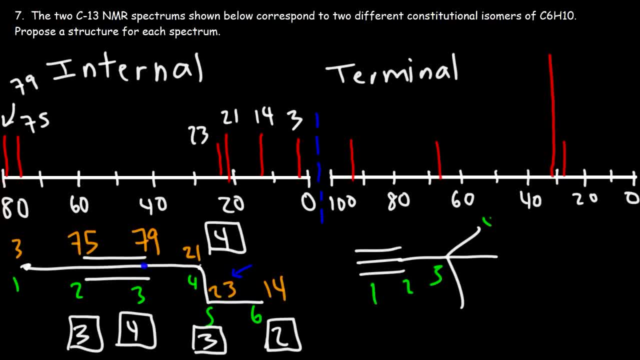 So this would be one, two, three and then four, which is consistent with the spectrum above, And so this is the structure for this particular spectrum. Now let me give you the numbers. So this signal is at 27.. 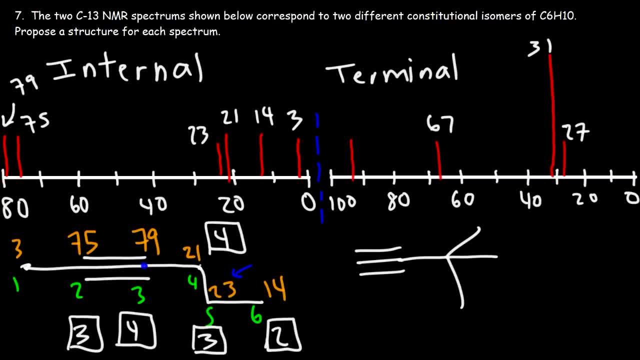 This one is at 31. And this is at 67. And this is at 93. So which signal corresponds to which carbon? So, looking at the two carbon atoms that are part of the triple bond, the carbon at the end is going to have a lower score value. 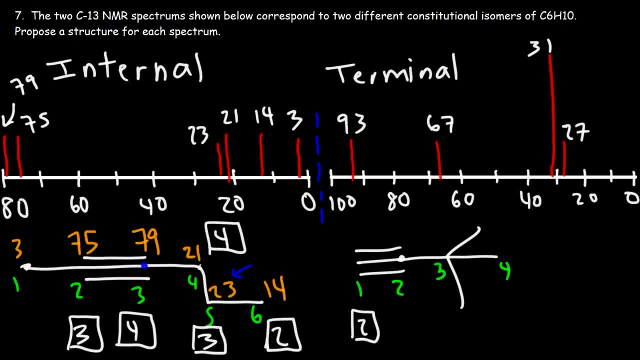 It's going to have a score value of two And the carbon two is going to have. it's adjacent to a primary and a quaternary, So it's going to have a score. So it's going to have a score value of five. 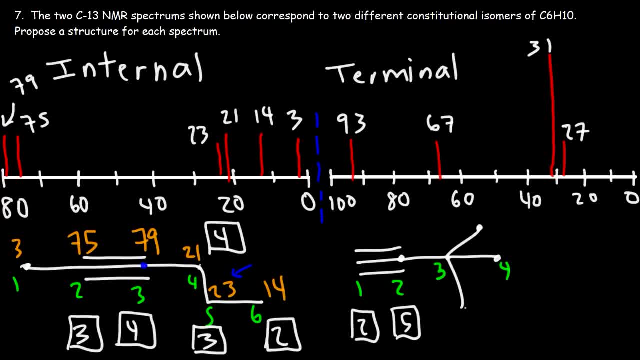 Carbon three is adjacent to three primary carbons and a secondary carbon, So therefore it's also going to have a score value of five. And carbon four is adjacent to a quaternary carbon, giving it a score value of four. So between the two carbon atoms that are part of the alkyne- 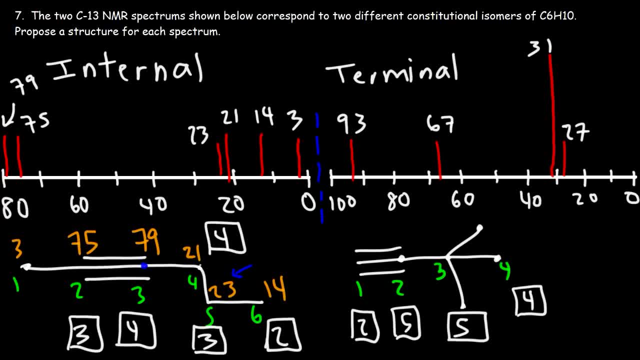 this one is clearly going to be the one that's higher, So that's the one of the chemical shift of 93. And the other one is 67. Now, which one is going to be higher? three or four? We really don't need to think too deeply about it, because the tall peak is at 31.. 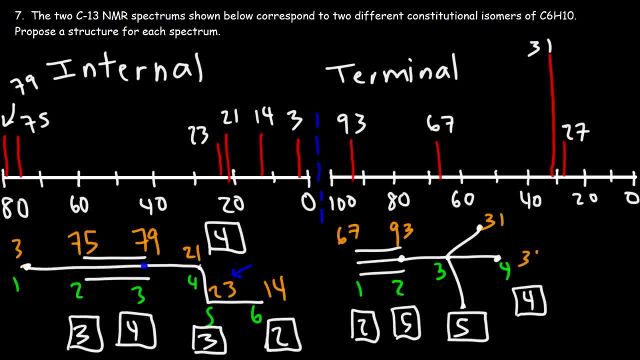 And that's going to correspond to the three methyl groups. So carbon four has that chemical shift. Carbon three has to be 27.. And we can see why it's a little less than 31. Because it's one carbon away from the alkyne group. 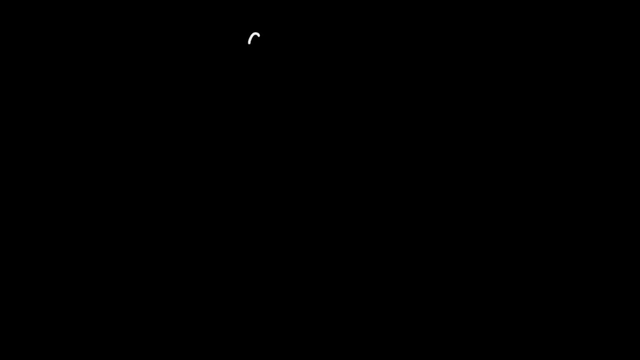 And so we see that. We see that drop in chemical shift. Now let's talk about alkenes. The carbon atoms in an alkyne have a chemical shift between 100 and 150 parts per million. And so let's consider an example. 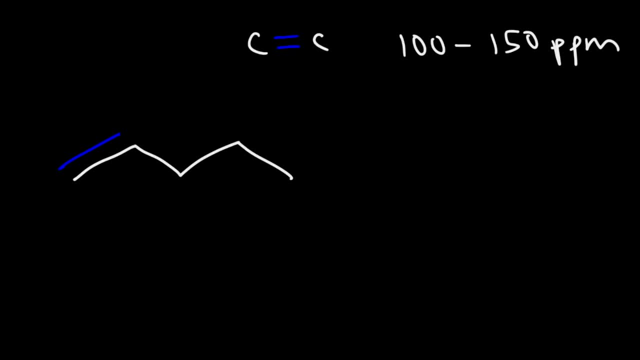 This is going to be one pentene, And so let's call this carbon A, B, C, D and E. Between carbons A and B, which one is going to have the higher chemical shift? Carbon A is next to a secondary carbon. 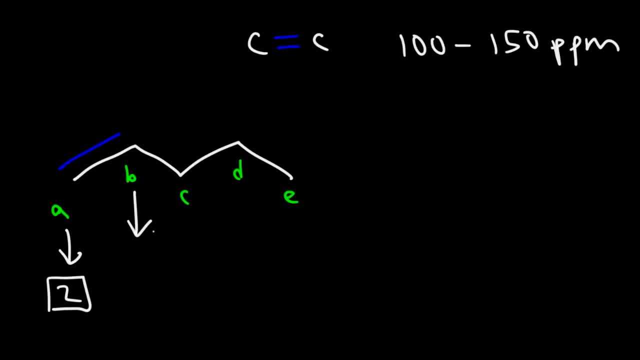 It has a score value of two. Carbon B is going to have a score value of three. This is primary and this is secondary. Carbon C is between two secondary carbons, So that's a score value of four, And then for D it's between: 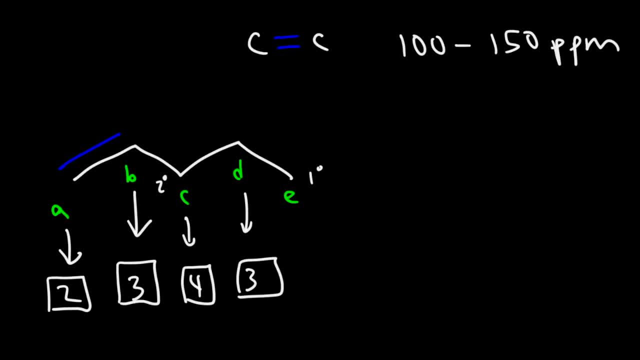 A secondary and a primary. That's a score value of three. And for E it's attached to or adjacent to a secondary carbon, Giving it a score value of two. So let's compare these two, because they're part of the double bond system. 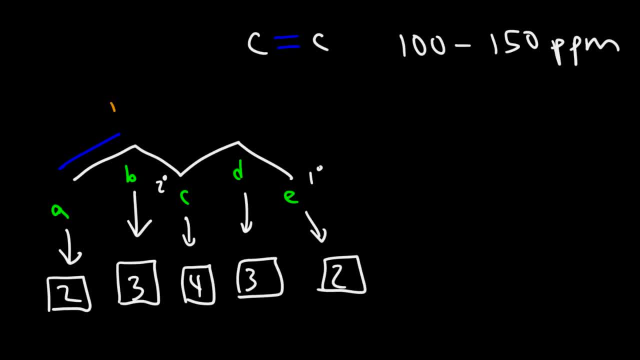 Carbon B is going to have a higher chemical shift And the value for it in this example is 139.. For carbon A it's 114.. So it's between 100 and 150, as we can see here. Now carbon C, D and E: we can rank them based on the score system. 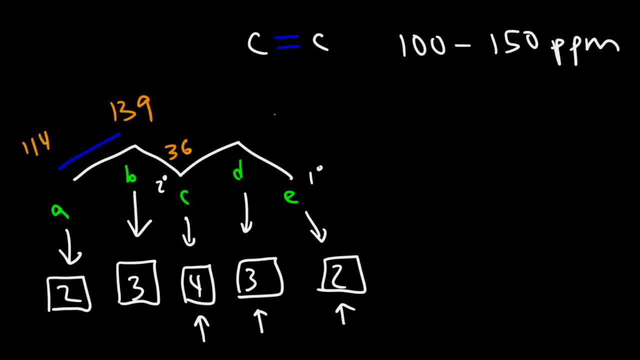 Carbon C is going to have the highest chemical shift, 36. Carbon D is 22.. Carbon E is 14. And so when dealing with alkenes, we don't see an unusual drop on the adjacent carbon. So we could use the score system to rank them. 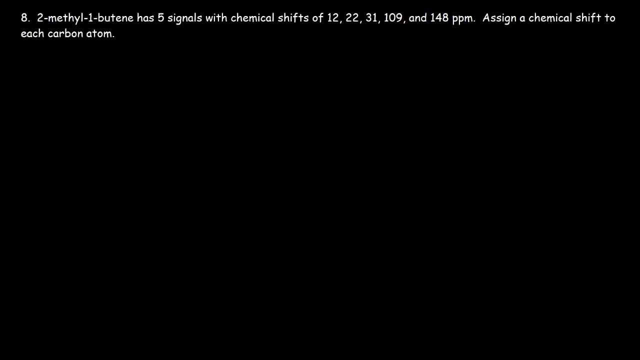 But for alkynes, watch out, for Let's work on this example. 2-methyl-1-butene has five signals with chemical shifts of 12, 22,, 31,, 109, and 148.. Assign a chemical shift to each carbon atom. 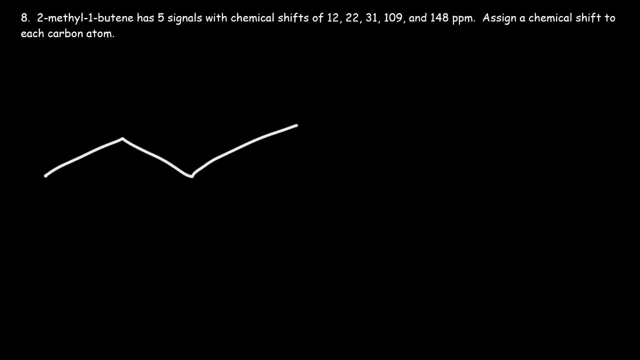 So let's begin by drawing butene. So we have a double bond on carbon 1.. So this is carbon 1,, 2,, 3, and 4. And there's a methyl group on carbon 2.. 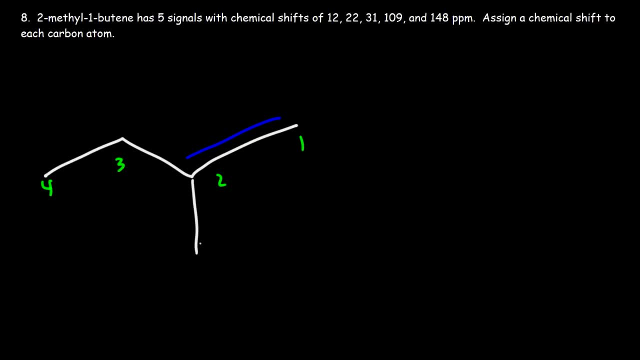 Now looking at carbons 1 and 2, let's call this carbon 5,. by the way, We know that carbon 1 is going to have a signal between 100 and 150.. And the same is true for carbon 2.. 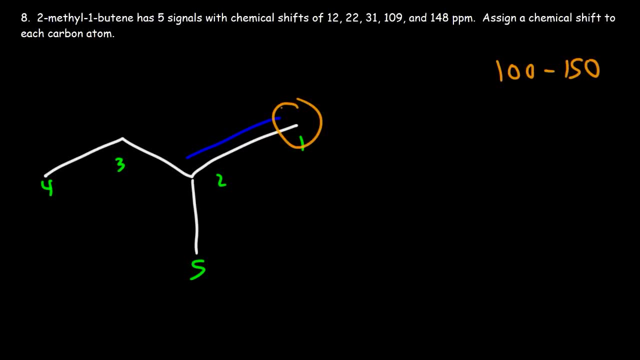 But carbon 1 is going to have a lower score value because it's at the end of the chain. So carbon 1 is going to be at 109.. And the carbon atom that is part of the double bond that is towards the interior of the molecule. 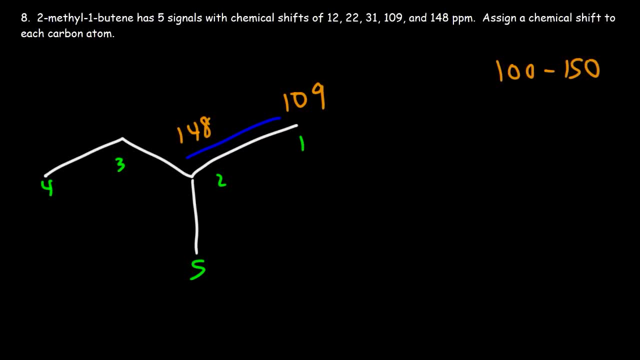 that's going to have a higher score value. So this is going to be 148.. Now for the other carbon atoms we need to actually calculate the score value. Carbon 5 is adjacent to a tertiary carbon, So that gives it a score value of 3.. 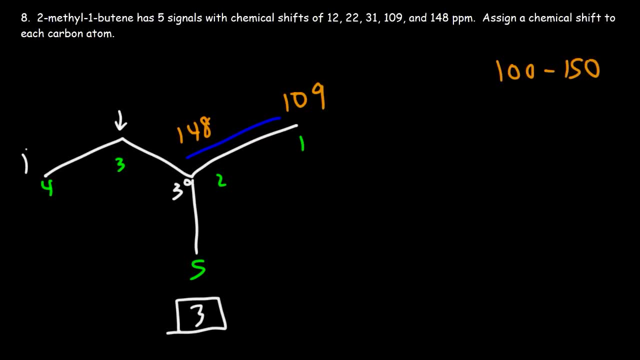 Carbon 3 is between a tertiary and a primary, So that gives it a score of 4.. And carbon 4 is next to a tertiary, So that gives it a score of 4.. And carbon 5 is next to a secondary carbon, giving it a score of 2.. 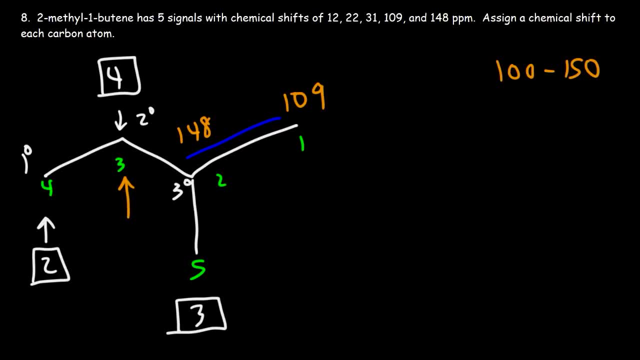 So carbon 3 is going to have the highest of the three remaining chemical shifts, which is going to be 31.. Carbon 5 has the next highest score value of 3.. So it's going to have the chemical shift of 22.. 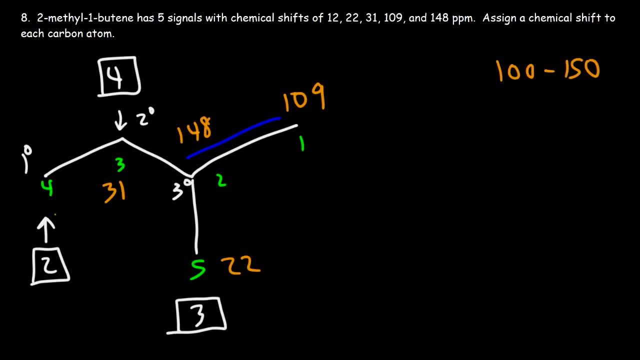 And the last one, carbon 4, with the lowest score value. that's going to have a chemical shift of 12.. And so that's it for this problem. So you could use the score system when dealing with alkenes. 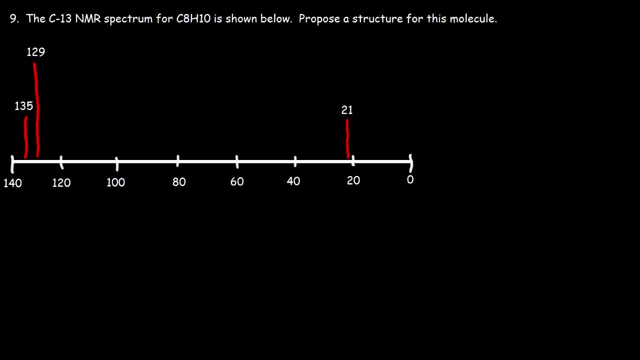 Number 9.. The carbon 13 NMR spectrum for C8H10 is shown below. Propose a structure for this molecule. So let's begin by calculating the index of hydrogen deficiency. So it's 2N plus 2, where N is the 8 carbons. 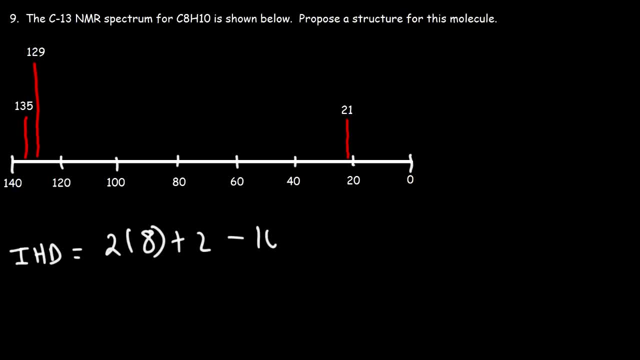 minus the number of hydrogen atoms, which is 10, divided by 2.. Now, 2 times 8 is 16.. 16 plus 2 is 18.. 18 minus 10 is 8.. And 8 divided by 2 is 4.. 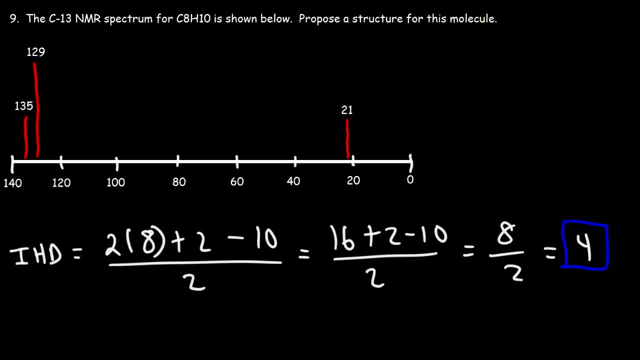 So the IHD is 4.. Now, looking at the signals that we see here, it's between 100 and 150.. So we have two possibilities: Either we have an alkene functional group or we have a benzene ring. 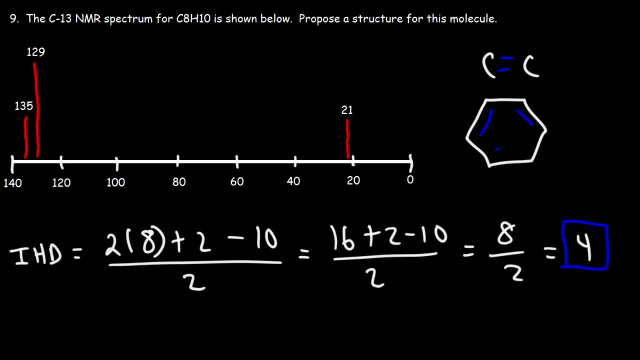 Now a benzene ring with 3 double bonds, and 1 ring has an IHD of 4.. An alkene has an IHD of 1.. So this could be a benzene ring or it can be a molecule with 4 double bonds. 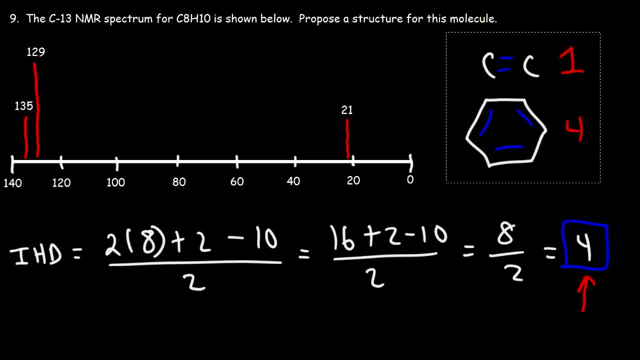 Which one do you think makes sense? Well, let's draw a structure with 8 carbons and 4 double bonds. So this would be 1, 2,, 3, 4.. This particular structure will not give us 3 signals. 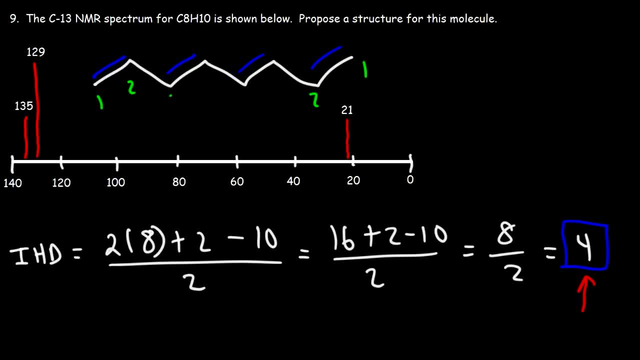 This would show up as signal 1,, 2,, 3,, 4.. And that's not including cis and trans effects. Now, if we attempt to, let's say, branch it off, which we could, this still won't give us the answer that we need. 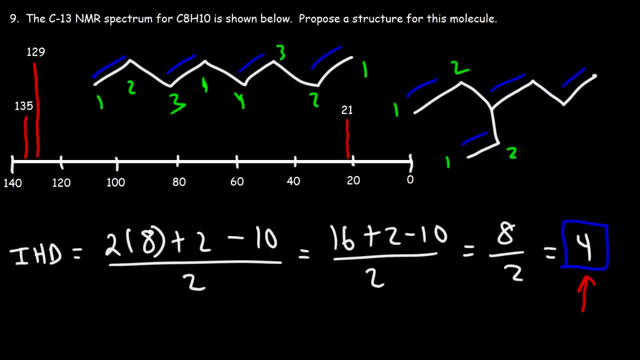 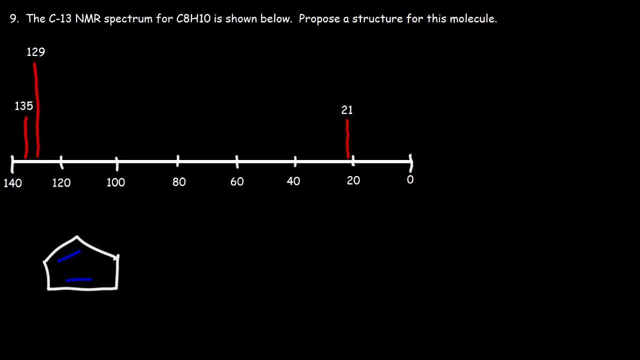 So this would be 1,, 2,, 3,, 4,, 5,, 6.. Now we could have some double bonds and a ring. That's another possibility. For instance, we could have a ring and 2 double bonds. 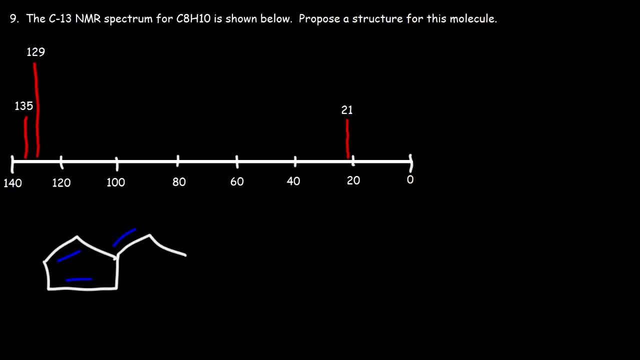 and perhaps another double bond outside of the ring. So right now we have a total of 7 carbons. We need 1 more And if we count, let's say, the number of signals, these 2 are identical. 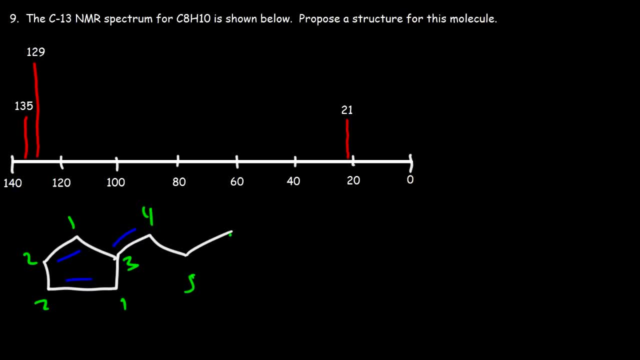 And then it's 3,, 4,, 5,, 6.. So that's not going to work either. What if we were to do something like this? Now, let's say we have another ring, So this is 6 carbons, 7, 8.. 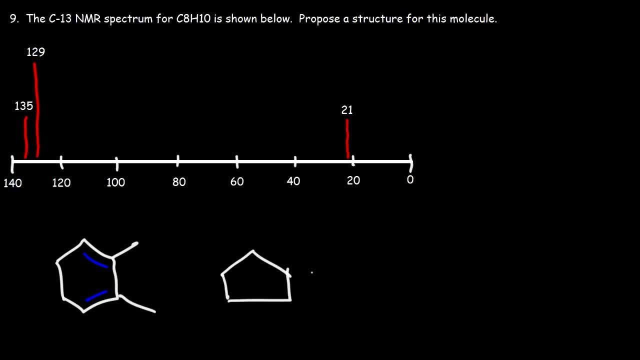 So that's not going to work. What about this one? This has an IHD of 4.. The structure I mean 3.. The structure on the right has an IHD of 4. And this has a total of. 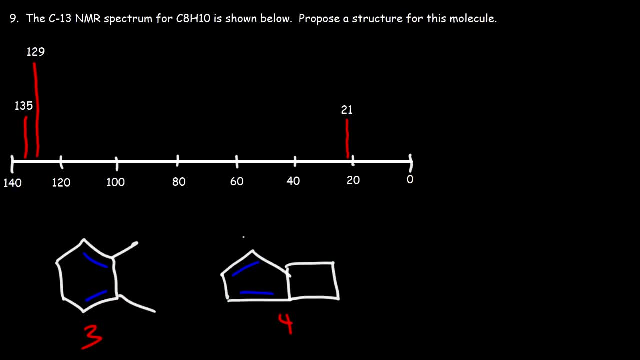 that's 7 carbons. So we've got to put a methyl group somewhere. Automatically that's not going to give us 3 signals. This is going to be 1, 2,, 3,, 4.. And then let's see 5,, 6,, 7,, 8.. 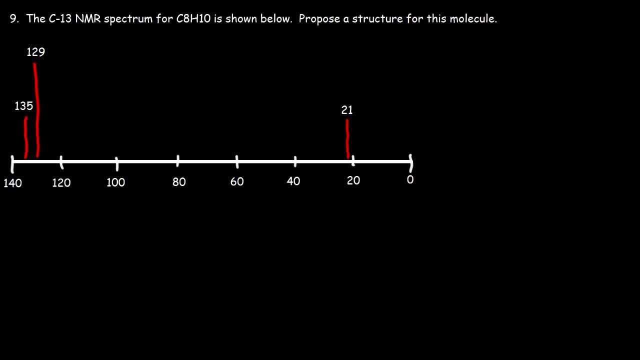 When in doubt. the best structure to draw when having an IHD of 4 or more is the benzene ring, Because this is going to be the most common structure that you're probably likely to encounter. Besides that, if it's something else, 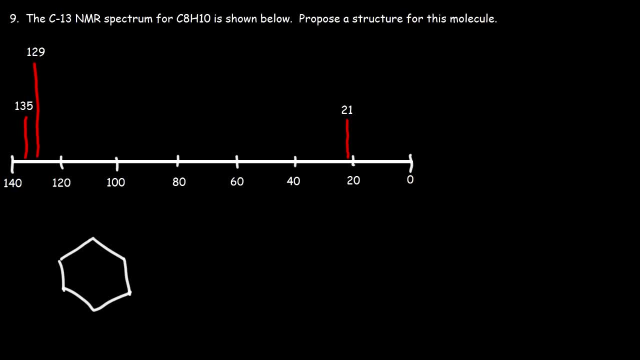 you'll need other forms of spectroscopy to basically pinpoint what it might be. So here we have a total of 8 carbons. This is ortho xylene. Here's another possibility. We could have ethyl benzene. So this has an IHD of 4. 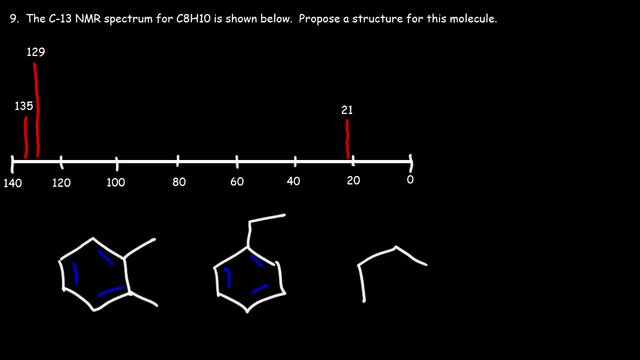 with 8 carbons. Another possibility is para xylene And another one could be meta xylene. So these all have 8 carbons, 10 hydrogen atoms. Now let's count the number of signals. So this is going to be 1,, 2,, 3, and 4.. 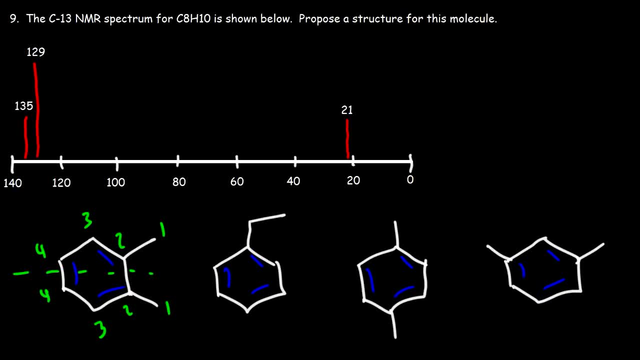 So you can see the line of symmetry here. For the next one, this is going to be 1,, 2,, 3,, 4,, 5,, 6.. And then these two are identical. Here's the line of symmetry. 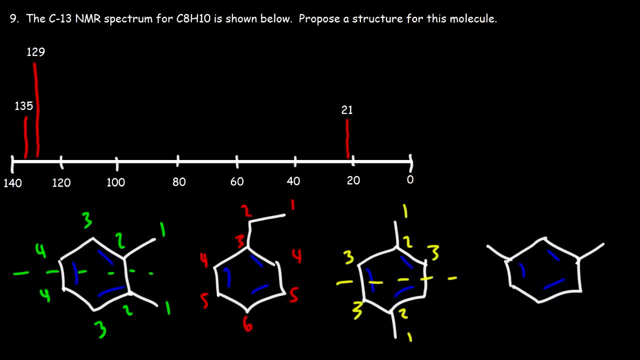 This is carbon 2.. And then carbon 3.. So this is the one that's going to work. Now, if we look at the last one, this is 1,, 2,, 3,, 4, and 5.. 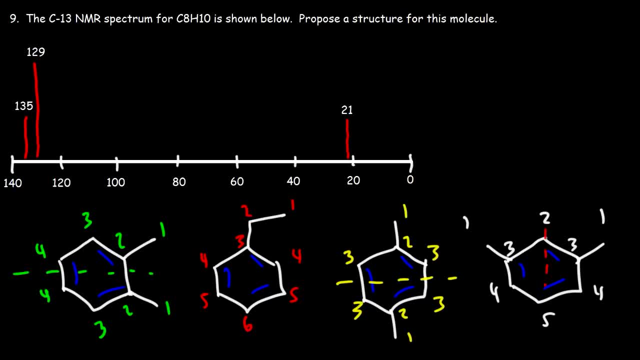 The line of symmetry is right down the middle. So this is going to be our answer. So let's redraw this molecule, but sideways. So let's call this carbon A and then B and carbon C. So clearly carbon A. 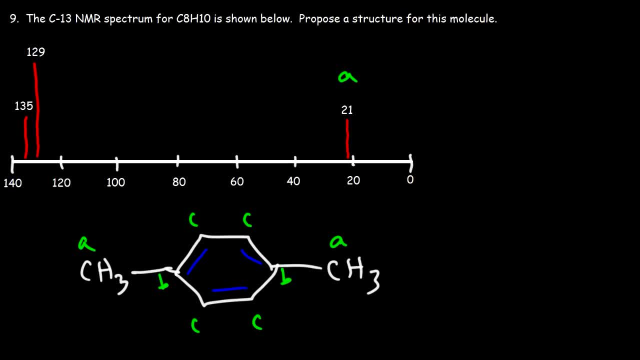 has to be the signal at 21.. That's typical of a methyl group. Now, what about carbons B and C? Notice that there's four signals that corresponds to carbon C, but only two correspond to carbon B. So carbon C. 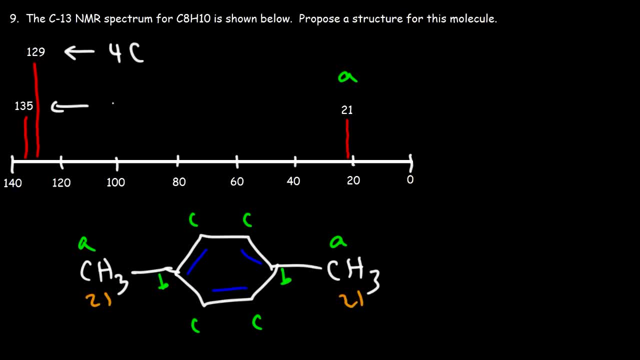 has to be the 129 signal, Carbon B has to be the 135 signal, And so height place an important role here. So this is 129, and this is going to be at 135.. And so that's how you could use. 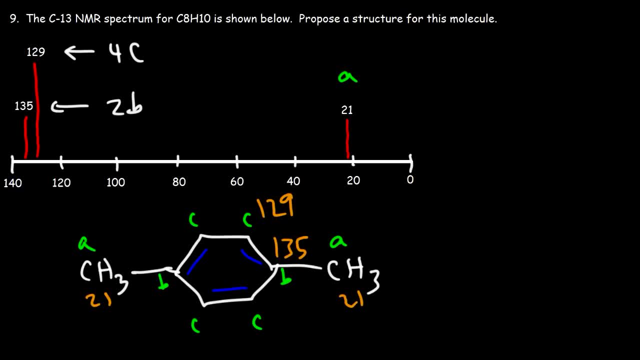 mass spectroscopy. I mean not mass spectroscopy but carbon 13 spectroscopy when dealing with benzene rings. Just know that the signals will be somewhere between 100 and 150.. And the ones that are chemically equivalent, the more carbon atoms. 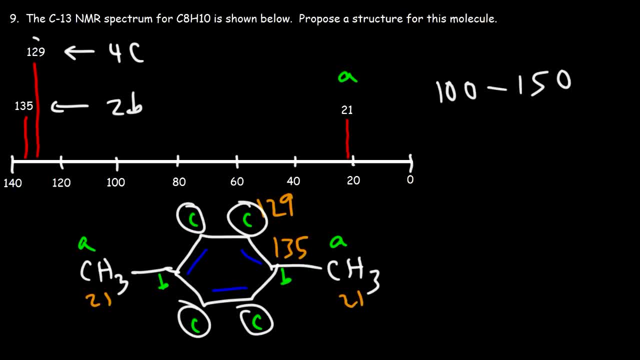 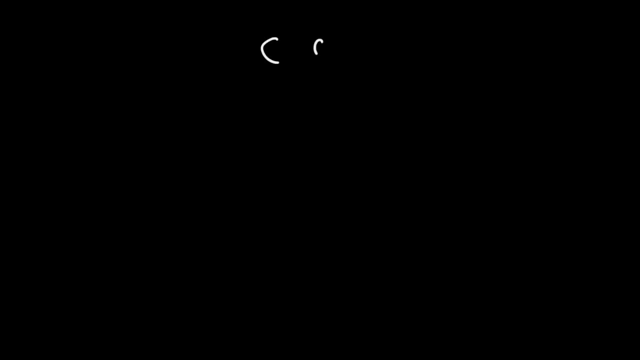 that are chemically equivalent will show up as a peak that's taller than the other ones. So keep that in mind, And then the last thing you need to use is the number of signals to distinguish one structure from another. Now let's focus on the carbonyl groups. 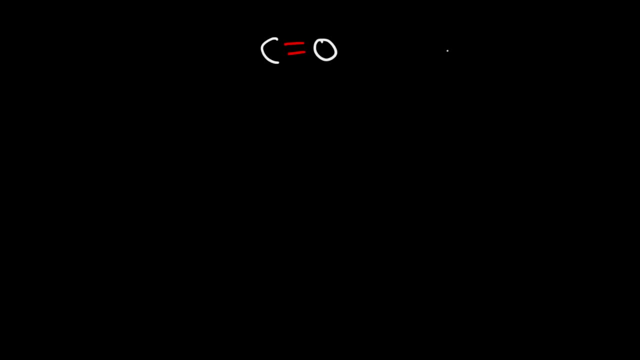 The chemical shift for this functional group varies between 150 and 220.. Now let's start with the ketones. Ketones have a higher chemical shift than the aldehydes in C13 NMR, And this is higher than the carboxylic acids. 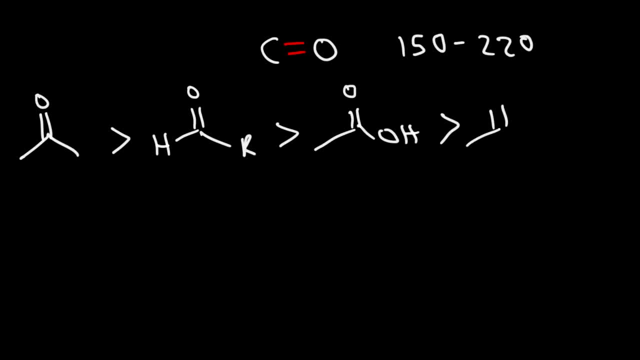 which are higher than the ester functional group And esters and amides. they're around the same range. So for a ketone it's usually around 205 to 220.. For an aldehyde, 190 to 205. 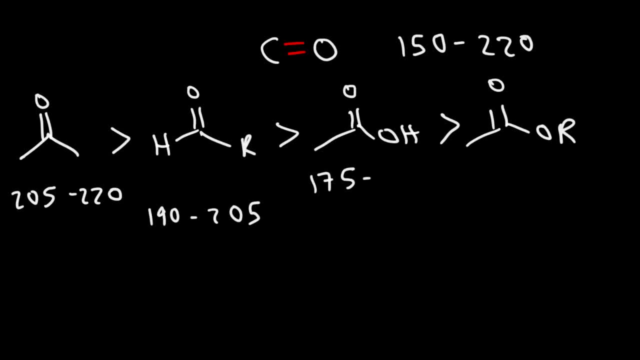 For a carboxylic acid, it's usually between 175 and 185.. And for ester and an amide, it's between 165 and 175.. Now let me give you some examples of some numbers that you might encounter. 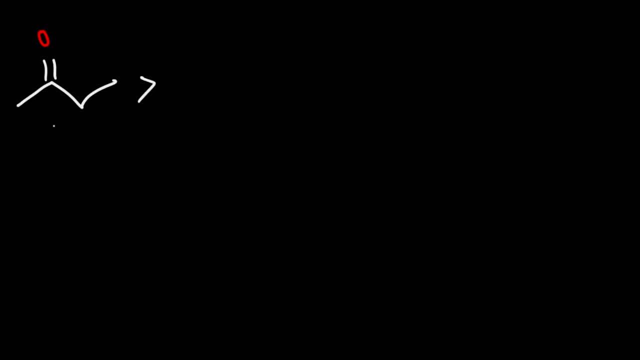 So here is butanone, And the chemical shift of the carbon in the carbonyl group is 209 for this ketone. Next we have an aldehyde. This is butanol, And the chemical shift for the carbon of this particular aldehyde. 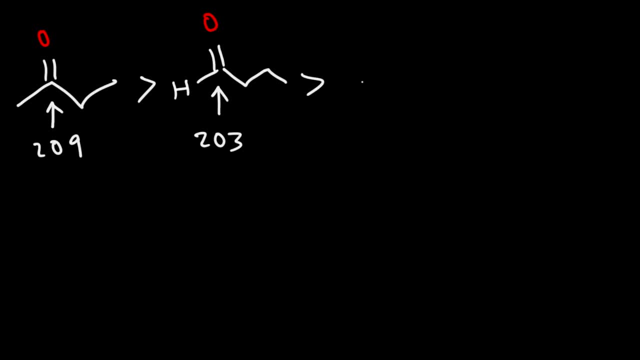 is 203.. In this example we have propanoic acid And the chemical shift of the carbon is 181. And for this example it's going to be an ester. So this is isopropyl ethanolate. 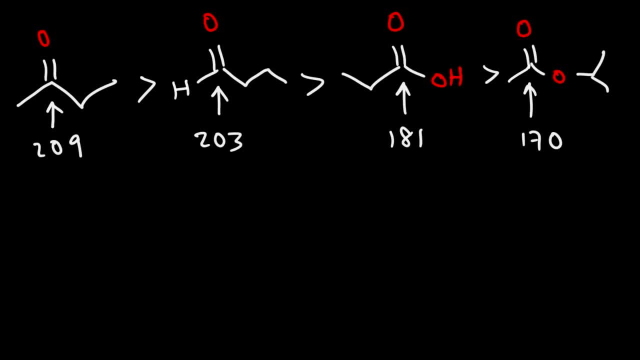 And it has a chemical shift of 170.. Now something interesting happens if you attach, let's say, a benzene ring to these functional groups. So if we have a benzene ring attached to, let's say, a ketone, 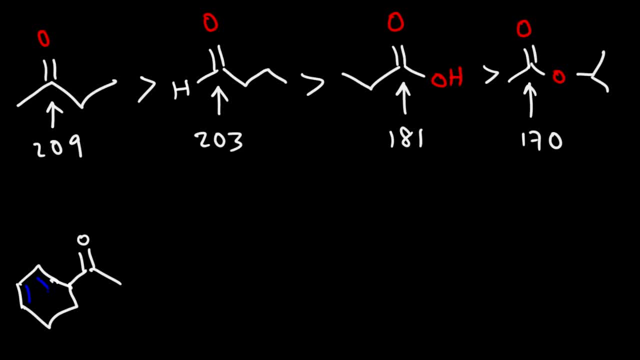 So this is acetophenone. Notice what happens. The chemical shift decreases from 209 to about 198.. And it makes sense because, let's say, if you put a carbon atom next to an electron withdrawn group, the chemical shift will go up. 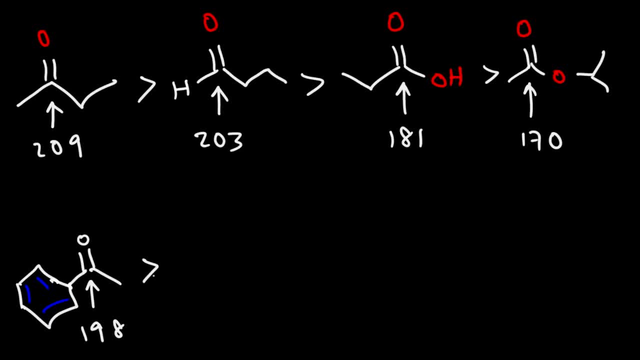 But if you put it next to an electron donating group, it's expected that the chemical shift should go down And the benzene ring can donate electron density to the carbonyl group, giving us a resonance structure that looks like this: And so 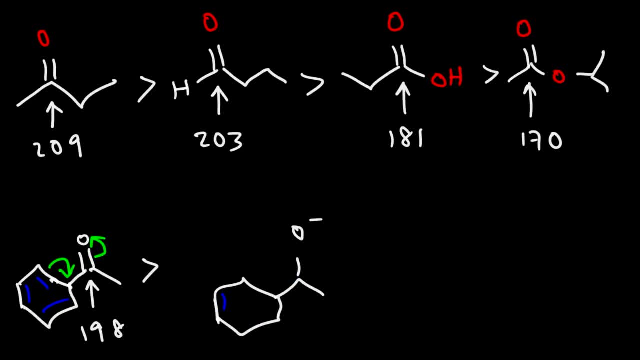 due to the resonance effect. we can see why the chemical shift decreases. Now the next one we're going to talk about is benzaldehyde. The chemical shift for this molecule will also decrease, And so it's going to be 192.. 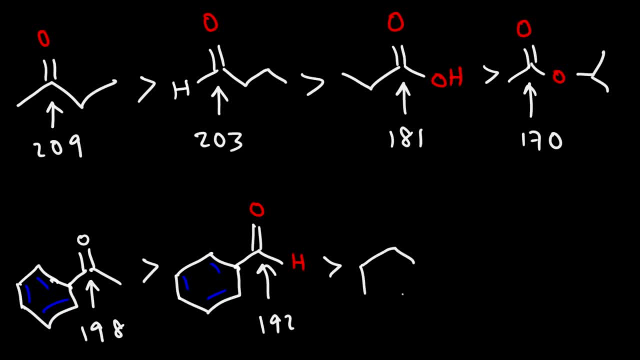 So in most cases we can see that there's a drop of, there's a drop in the chemical shift approximately about 10.. Now this one is going to be benzoic acid And the chemical shift of the carbonyl group is 172.. 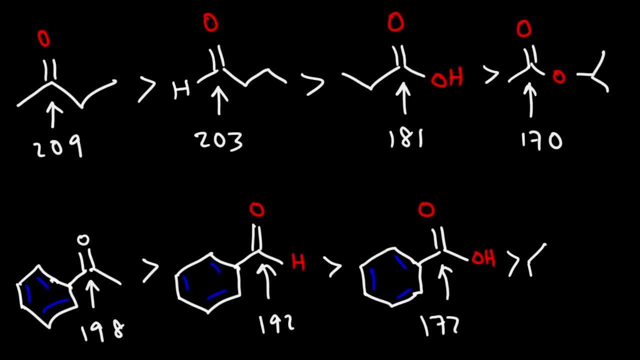 And the last one is going to be an ester- And I'm running out of space here- And the chemical shift for this one it's not that low, But it's 167.. So it's a little bit lower than what we see here. 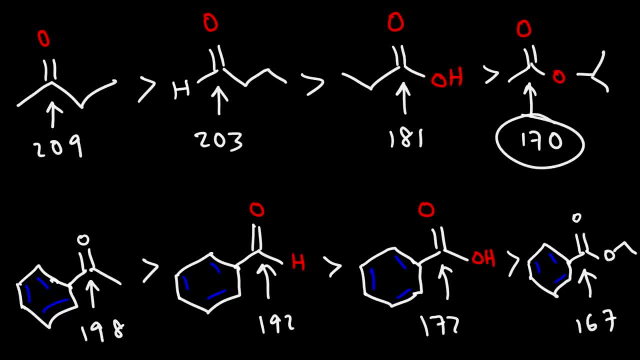 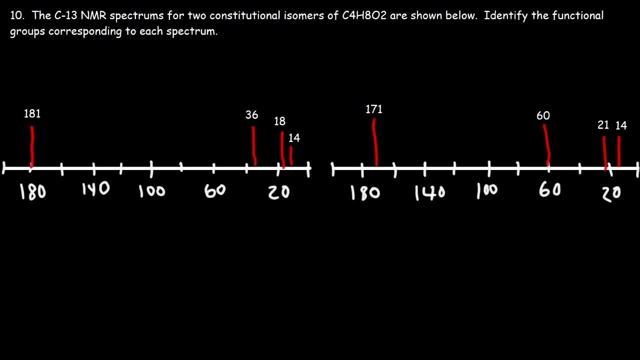 So if you add an electron donating group to a carbonyl group, it's expected that the chemical shift should decrease slightly. Number 10. The carbon 13 NMR spectrums for two constitutional isomers of C4H8O2. 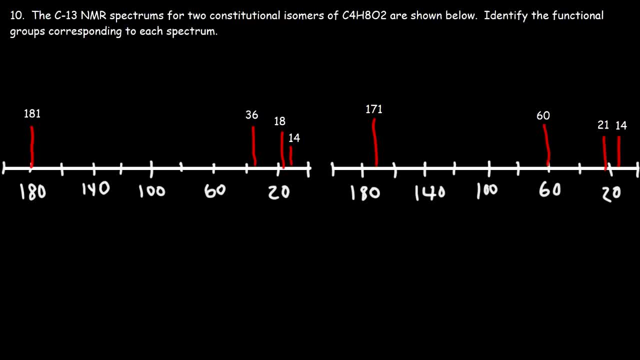 are shown below, Identify the functional groups corresponding to each spectrum. So, as always, let's begin with the IHD. So it's 2N plus 2, where N is 4 in this example, minus the number of hydrogen atoms, which is 8,. 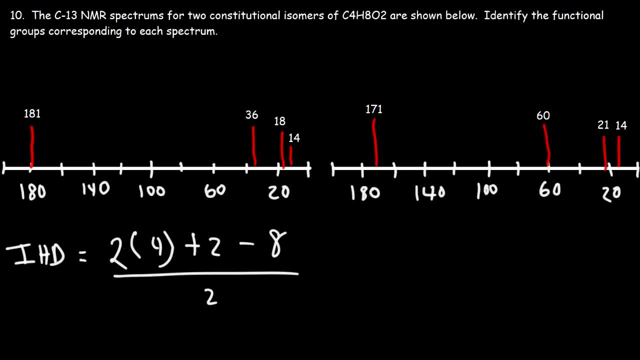 divided by 2.. Now, 2 times 4 is 8.. So that's going to cancel with this 8.. And so it's going to be 2 over 2, which is 1.. So this, either, is one double bond. 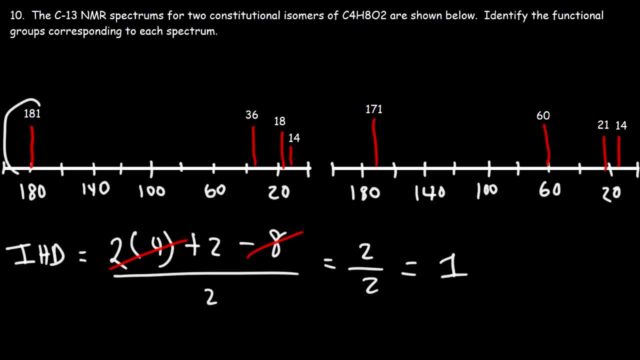 or a ring. Now, in both cases we see a signal between 150 and 220.. So that's going to be the carbonyl functional group, And so that's going to be our double bond in this situation. Now we don't have any alkenes. 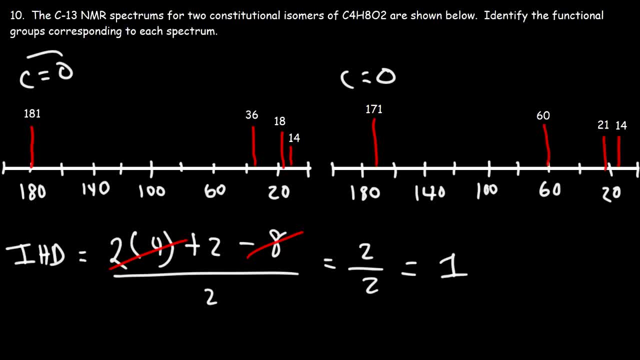 or any benzene rings. So therefore, the carbonyl groups won't be shifted down by 10, as we saw, if we attached them to a benzene ring in the last example. Now for us to have, let's say: 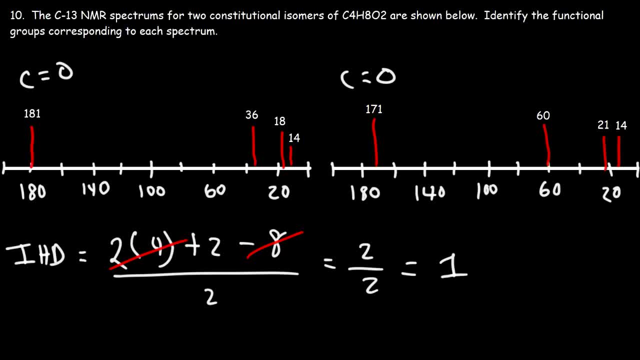 a ketone, the signal is usually around 210.. For an aldehyde, it's close to 200.. The signal at 180,- this indicates a carboxylic acid, And the signal at 170, this is likely to be. 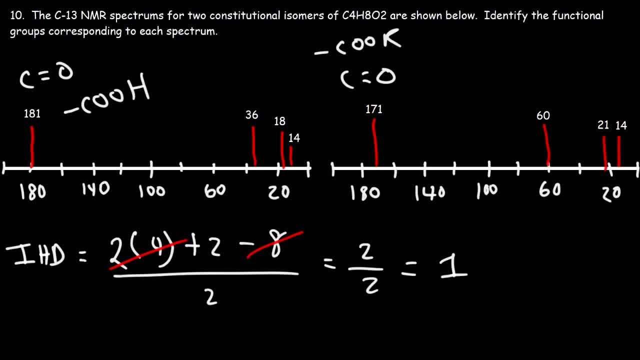 the ester. Notice that we have a signal at 60. So this is the CO bond of the ester. but we don't see that for a carboxylic acid. Now let's talk about why. because the carboxylic acid does have. 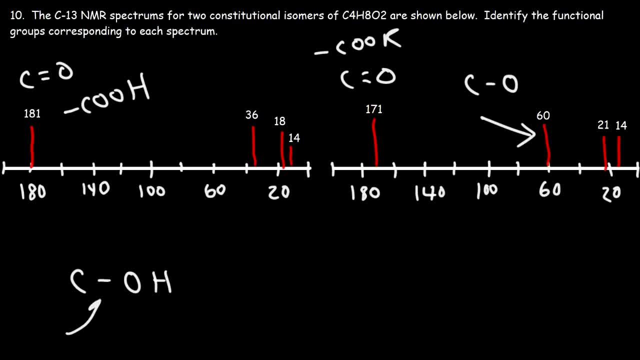 a CO bond. So why don't we see a signal between 50 and 100 for the CO bond of a carboxylic acid? What would you say For an ester notice that there's two CO bonds? This is the one that appears at 60.. 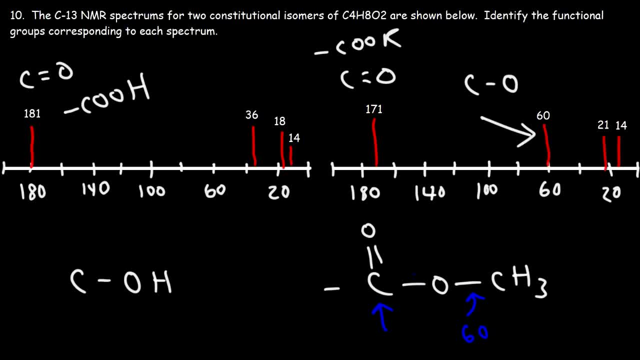 And for this one, this is part of the carbonyl system, Even though it has a CO bond, because it's attached to the carbonyl group. this is the signal that we see at 171.. In the case of a carboxylic acid, 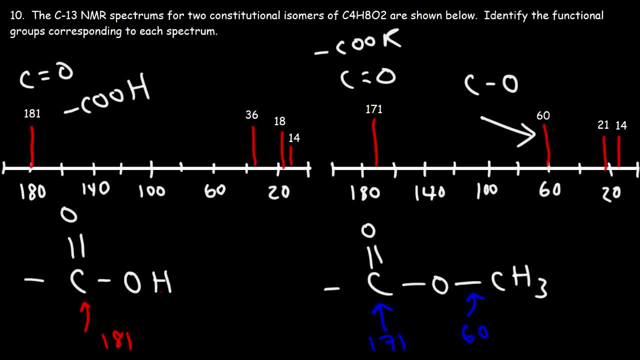 this carbon is going to appear at 181.. This CO bond is not really relevant, because that same carbon is still part of the carbonyl group, And so this is one way in which you can distinguish a carboxylic acid from an ester. An ester. 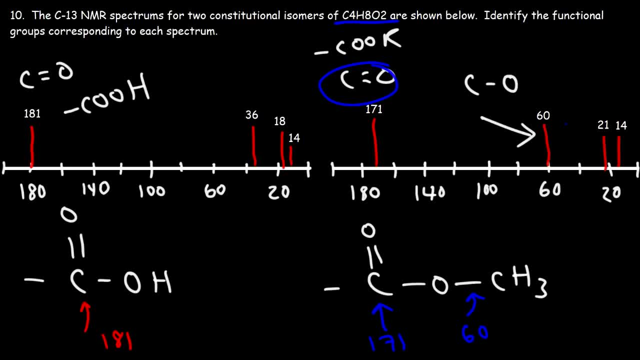 will have the signal at 170 and the CO signal between 50 and 100.. Whereas the carboxylic acid it's not going to have the CO signal between 50 and 100.. Now the spectrum on the left corresponds to: 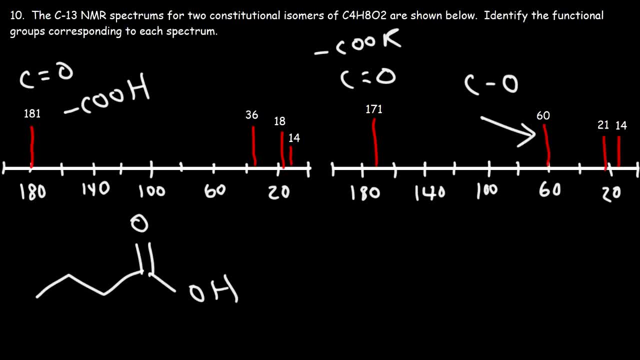 butanoic acid. So this carbon has a signal of 181.. The next one adjacent to it is 36.. The beta carbon is 18. And the gamma carbon is 14.. In the case of the ester, this corresponds: 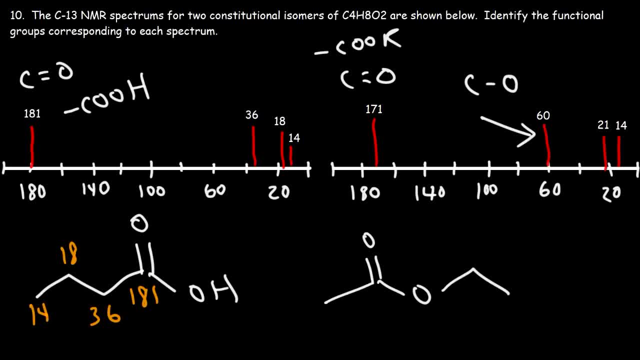 to ethyl acetate. The carbonyl carbon has a chemical shift of 171.. And this carbon here, that's the CO bond of the ester. that corresponds to 60. The methyl group on the right is 14 and the methyl group on the left is 21.. 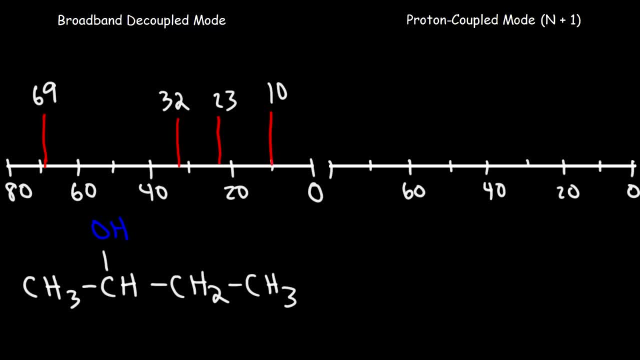 Now the examples that we've seen before. all of the spectrums that we've considered were based on this mode: broadband decoupled. All of the signals appeared as singlets. But there's another mode that you need to be familiar with. 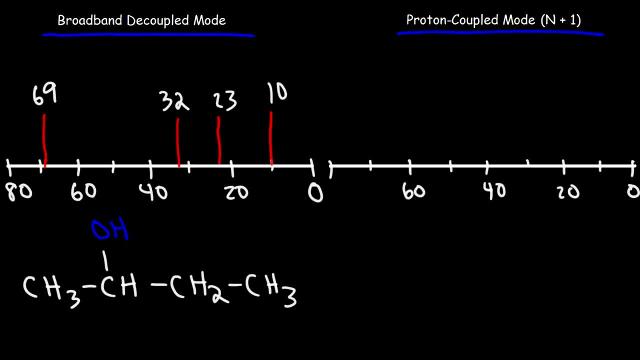 And that is the proton-coupled mode of C13 NMR. And in this case you're going to see splitting, not on, not from the adjacent hydrogens, but the hydrogens that are directly attached to the carbon. they will split those carbon signals into. 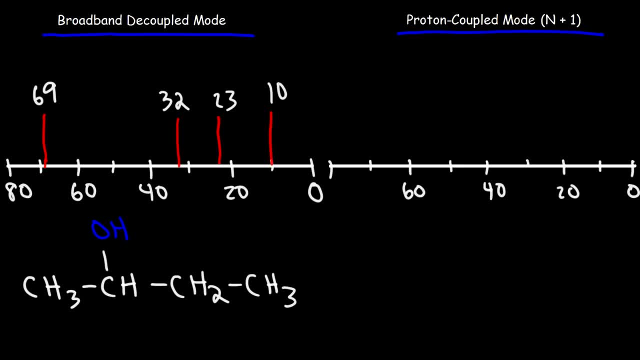 triplets, doublets and quartets. Let's call this carbon A, B, C and D. Carbon B is the signal at 69.. Carbon A is the signal at 23.. And carbon C is the signal at 32.. D is 10.. Now, what type of splitting pattern are we going to see for carbon 3?? In HNMR, we would look at the adjacent hydrogens, But for proton-coupled C13- NMR, we're not going to look at the adjacent hydrogens. 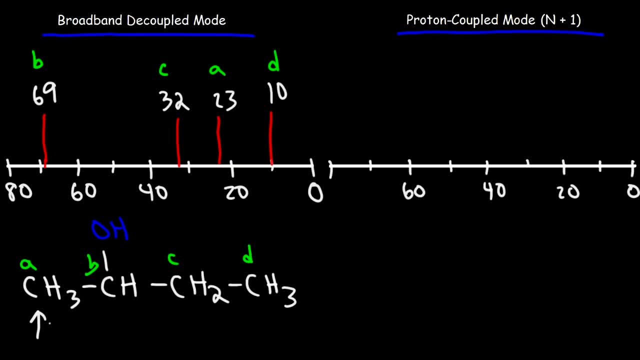 To analyze carbon B, we're going to use the hydrogen atoms that are directly attached to this particular carbon. So what is the splitting pattern that we see here for carbon A? Well, carbon A show up as a singlet, doublet, triplet or quartet. 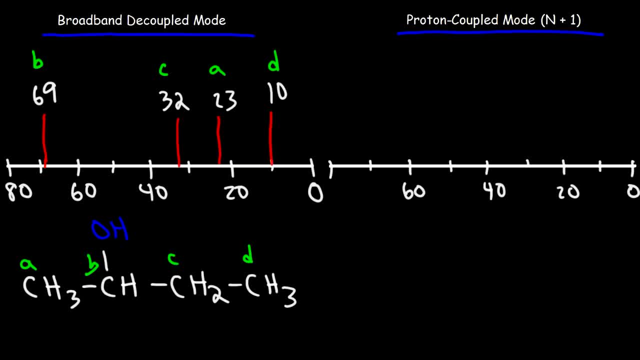 Now carbon A has three protons And so, using the N plus 1 rule, 3 plus 1 is 4.. So therefore carbon A will appear as a quartet. So carbon A is at 23.. 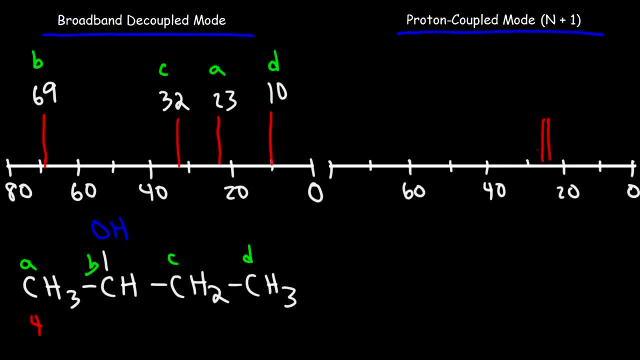 And so let's draw a quartet in this region. Now, keep in mind, you could draw it like this if you want to. Now, moving on to carbon B, Carbon B only has one proton on it, So 1 plus 1 is 2.. 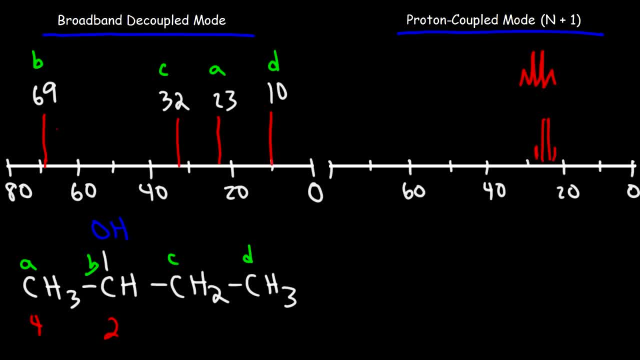 This is going to appear as a doublet, And so that's at 69.. So let's draw a doublet at 69.. Or you can draw it this way Now: carbon C has two protons. It's a methylene group. 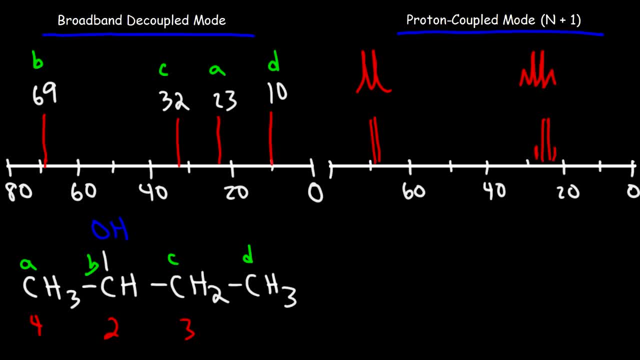 2 plus 1 is 3., And so this is going to appear as a triplet at 32.. So we can draw it like this Or like that. Now, the last one is a methyl group, So this is going to be: 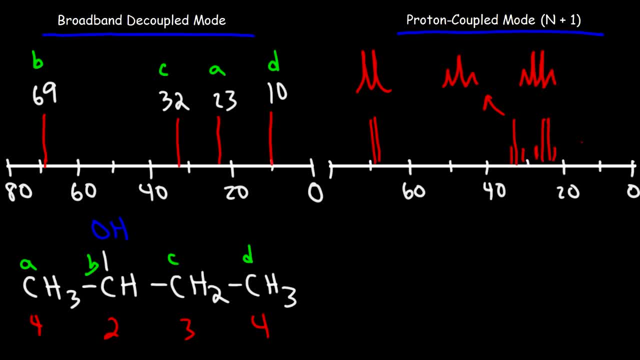 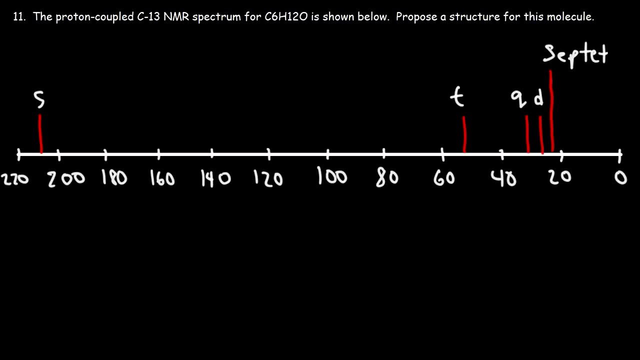 another quartet And that's at a signal of 10. So it's going to look like that Number 11.. The proton-coupled C13 NMR spectrum for C6H12O is shown below. Propose a structure for this molecule. 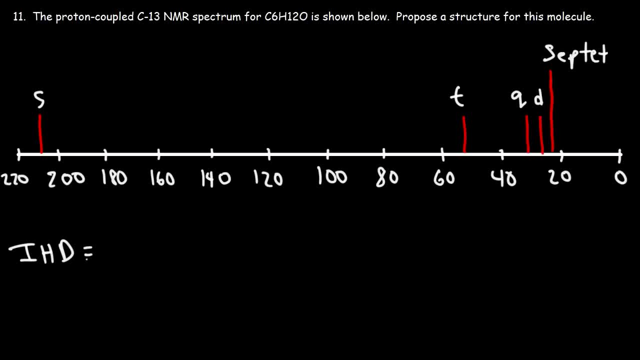 So, as always, let's begin with the IHD calculations. So it's going to be 2 times 6 plus 2 minus the 12 hydrogen atoms divided by 2.. 2 times 6 is 12., And so that's going to cancel with negative 12.. 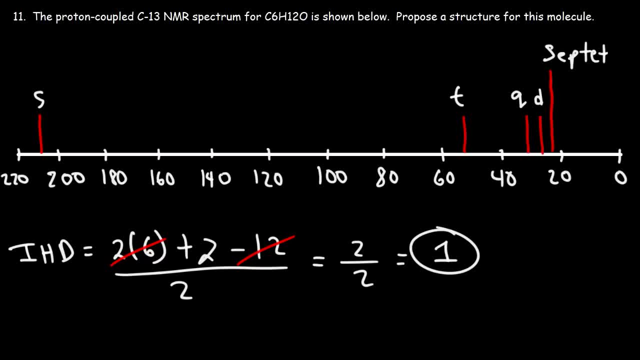 And thus we're going to get an IHD of 1.. Which means we could have one double bond or one ring. Now the double bond is going to be a carbon no group, because we see a signal close to 210.. And that's. 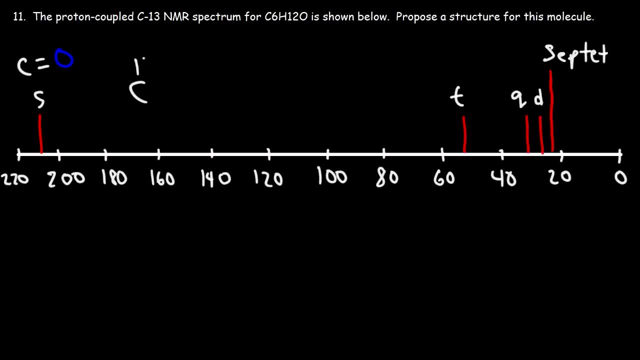 usually the signal for a ketone. Now this is going to appear as a singlet, So we got the multiplicity for the signals as well. This is a triplet, quartet, doublet and a septet, So with: 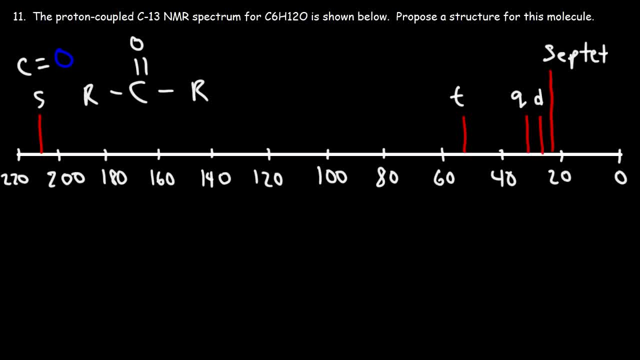 that in mind, what do you think this structure is going to be Now? for the triplet, this corresponds to a methylene group, because 2 plus 1 is 3.. For the quartet, this corresponds to a methyl group: 3 plus 1 is 4.. 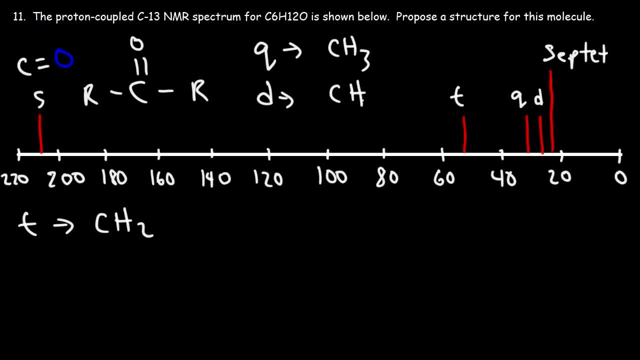 For the doublet, this corresponds to a methane group: 1 plus 1 is 2.. And for the septet, this is going to be 2 methyl groups that are attached to the same carbon atom, Because 6 plus 1 is 7.. 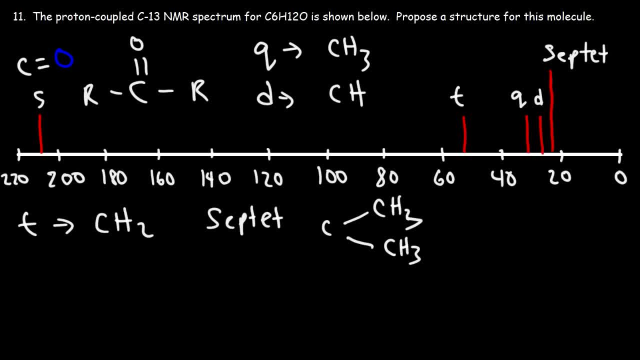 So let's see if we can put all of this together. What type of group do we have here? Will it be a CH, CH2, CH3, or just a C? Now, it can't be a CH3, because methyl groups always exist. 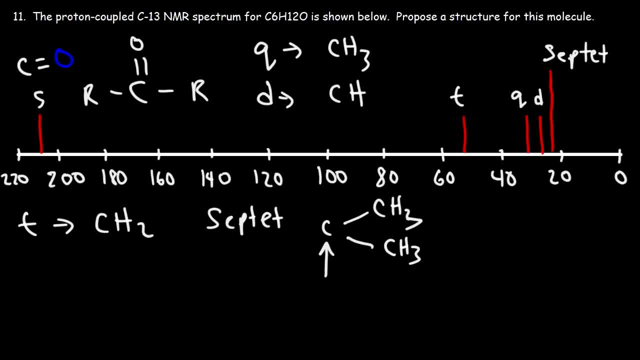 at the end of a structure. It can't be a CH2, because then we would only have a total of 3 carbons. It's either a C or a CH. Now we have a total of 6 carbons. So 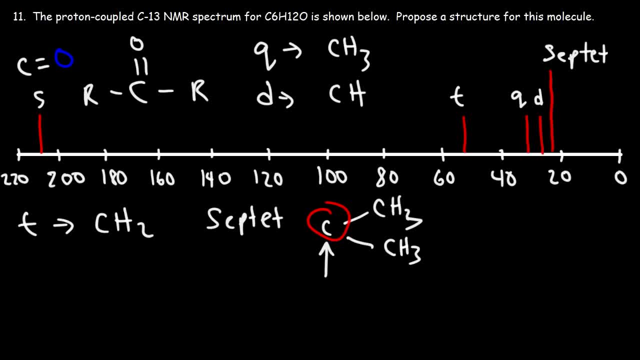 using that, how can we tell if this is going to be a C or a CH? Well, here's the first carbon, Here is the second, third, fourth, and then these two would add up to 6.. So we don't have. 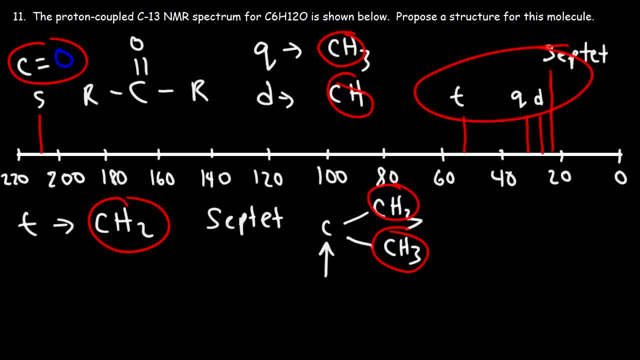 any C's in our graph, in our spectrum. There's no missing carbons that we didn't account for. So this has to be the CH. It can't be anything else. So we're going to make this the right side. 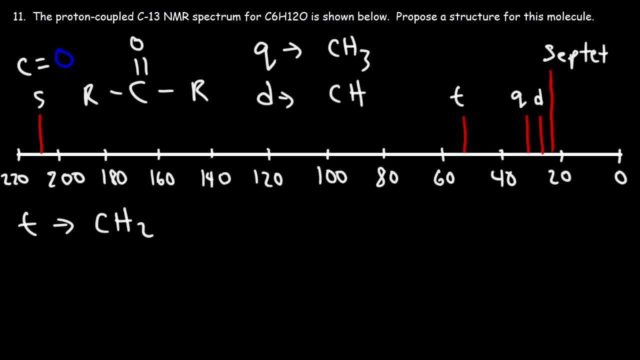 of the molecule, So we're going to make this the right side of the molecule. Okay, what just happened? This computer is acting weird, So we're going to have a CH attached to two methyl groups. So we used up this signal. 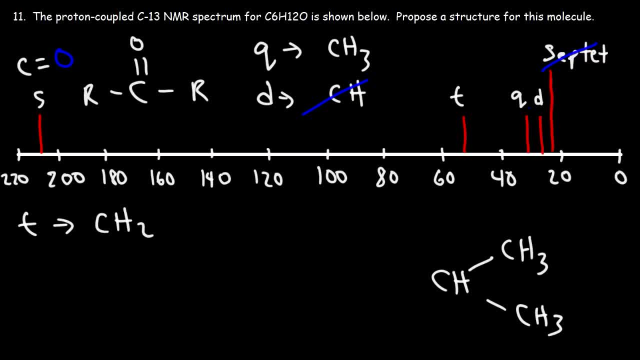 and the septet. Now we still have another methyl group to put in this molecule somewhere And we're going to put that on the left side. Let's put it over here, Since methyl groups always exist at the end of a molecule. 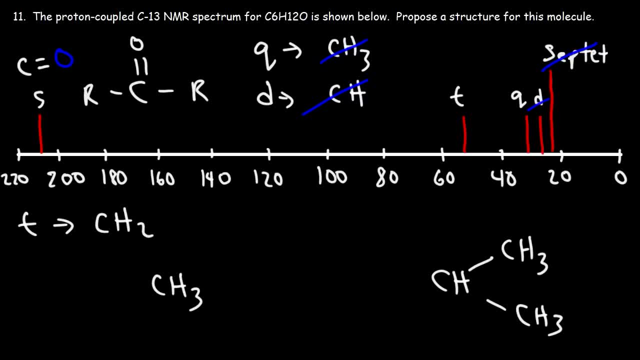 Now, the only two other things we need to put into this equation is the methylene group and the carbonyl group. So one possibility is to write it out like this. The other possibility is to put the methyl group and then the carbonyl group, followed by. 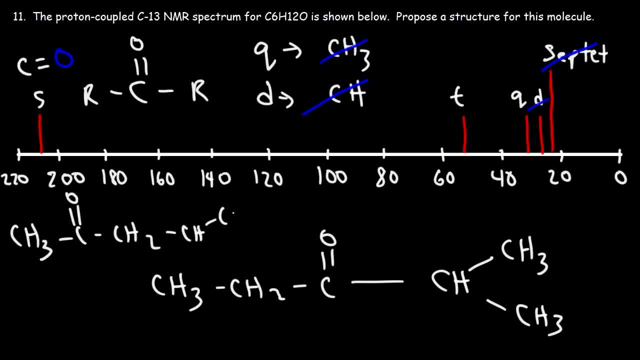 the methylene group and the isopropyl group. So those are the two ways in which we can connect all the groups that we have here, based on the spectrum. So now let's put down the signals that we have. The signal for the carbonyl. 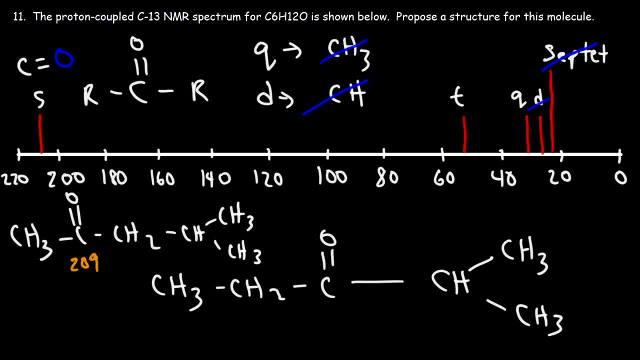 group is 209.. And for the septet that's around 23.. So that's the two methyl groups that are equivalent to each other, And we can see that, because the peak is tall, it indicates that there's two or more equivalent carbons. 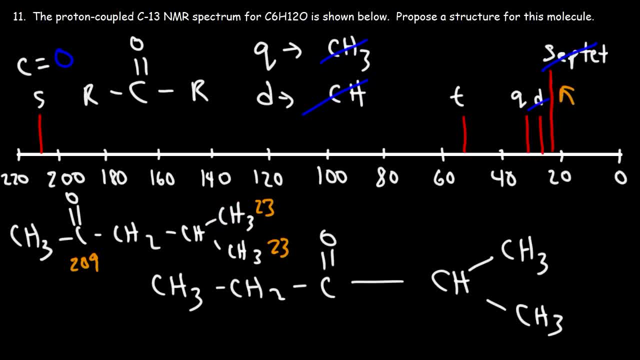 that correspond to that signal. Now the doublet, that's around 25.. So that's going to be the CH carbon, And the triplet has to be the methylene carbon. So that's going to be at 53.. 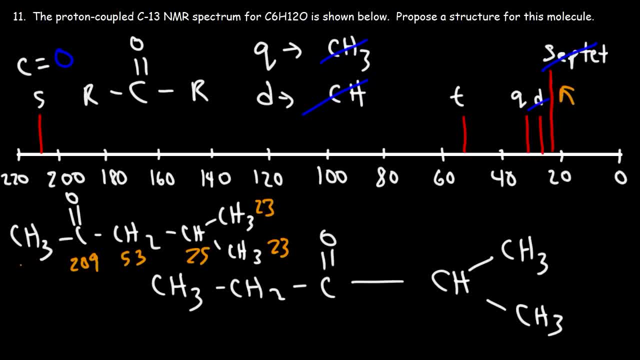 And the quartet is the methyl carbon, which is at 30. So for this molecule the numbers will be the same. Now let's use the score system to see which of these two structures is more consistent with the spectrum. So let's calculate the score value. 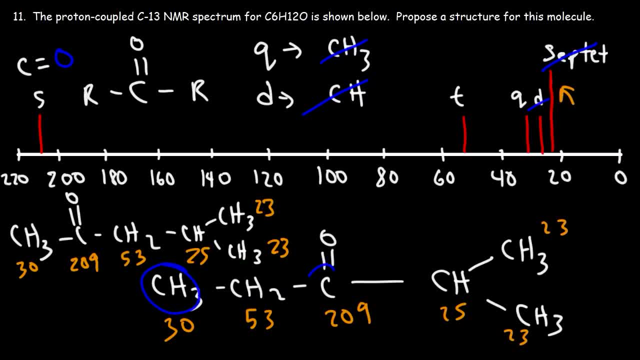 of the methylene group. So this is a primary carbon, this is a secondary carbon. So we're going to give this a score value of 3.. And for this one, the methyl group, it's next to a secondary carbon. 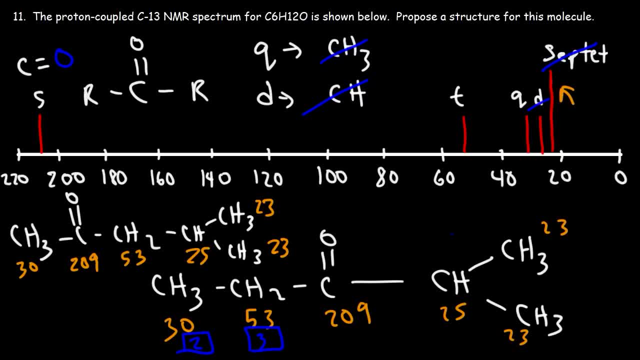 So we're going to give it a score value of 2.. Now for the methane group, it's adjacent to two primary carbons and a secondary carbon, So we're going to give it a score value of 4.. So notice that. 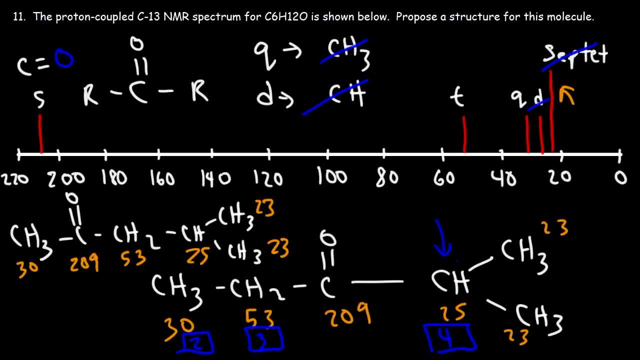 the methyl group has a higher score value but a lower chemical shift compared to the methylene group. I mean this is a methane group, or called a methyl group, But the CH group. it has a lower chemical shift of 25 compared to the CH2. 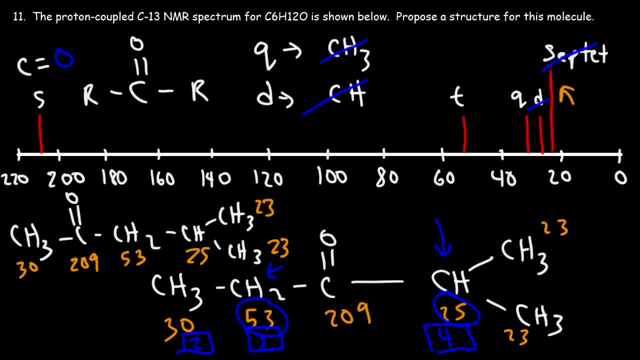 group, which is 53.. And they're both one carbon away from the carbonyl group And this has a higher score value. So it doesn't make sense that the methylene group will have a higher chemical shift. Therefore, this structure is not consistent. 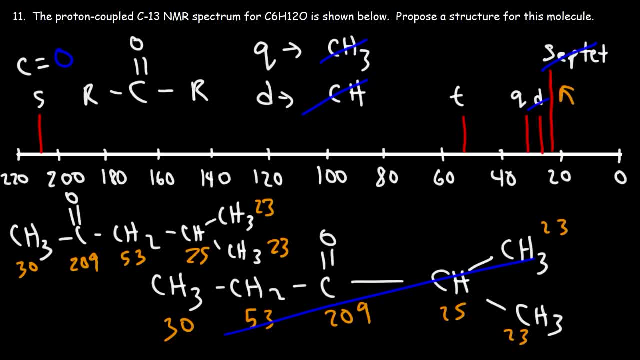 with the score system. Now let's look at this structure. The methyl group here still has a score value of 2. That's not going to change Now. the methylene group is adjacent to a secondary carbon and a tertiary carbon. 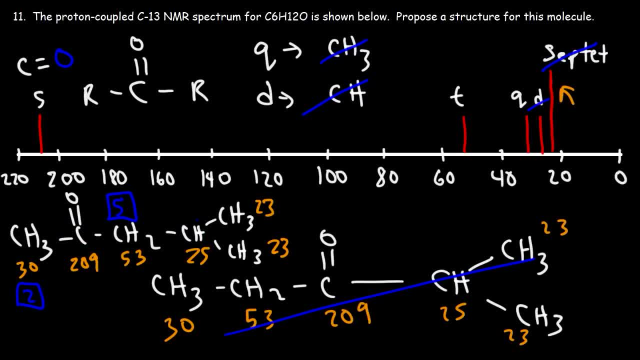 giving it a score value of 5.. The methane group is next to a primary, a primary and a secondary, Giving it a score value of 4.. So now we can see why the methylene group is much higher than the methane group. 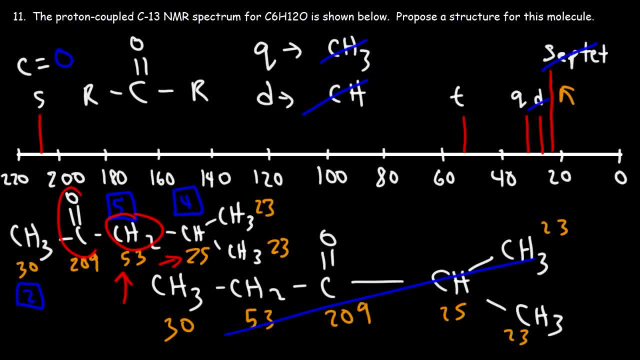 For one reason: this is next to the carbonyl group and the methane group is not, So that's one reason why this is higher than this one. The second reason is that it has a higher score, So there's two factors favoring the high chemical shift of the. 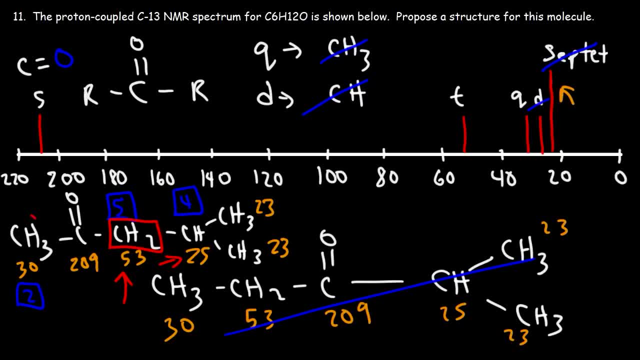 CH2 group And if we compare these two, clearly this has a higher score value, Even though these two groups are one carbon away from the carbonyl group. This has a score value of 5. This one has a score value of 2.. 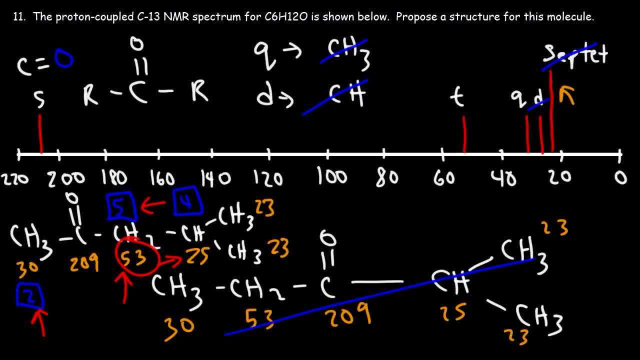 And so we can see why the CH2's chemical shift is much higher than the methyl's chemical shift. So this structure is most consistent with the data that we see in the special spectrum above, And so it turns out that this is indeed the answer. 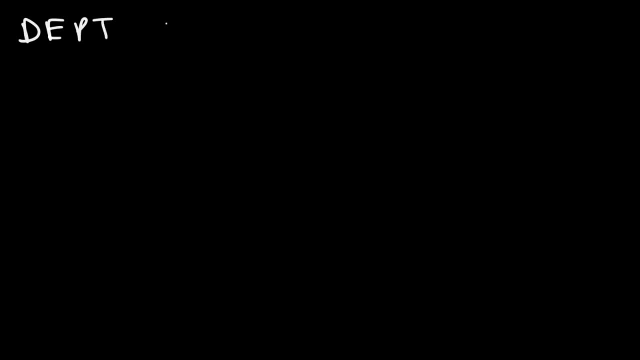 Now, the last thing that I want to discuss in this video is something called DEPT-C13 NMR spectroscopy. DEPT D-E-P-T stands for Distortionless Enhancement by Polarization Transfer. Now, what you need to know is that if the excitation angle is at 0 degrees, 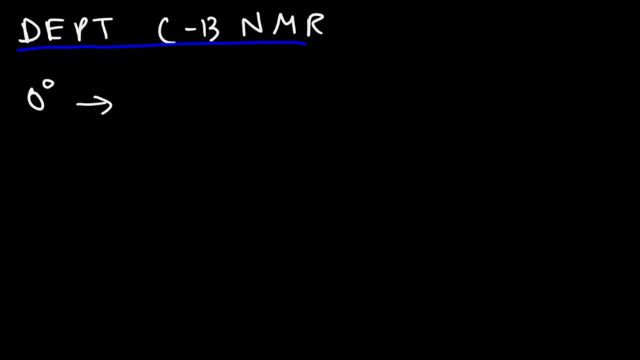 this is basically the same as a broadband decoupled C13 NMR spectrum where you'll see all the signals. You'll see the carbons, the CH's, the methylene groups and the methyl groups. Now, if the angle is at, 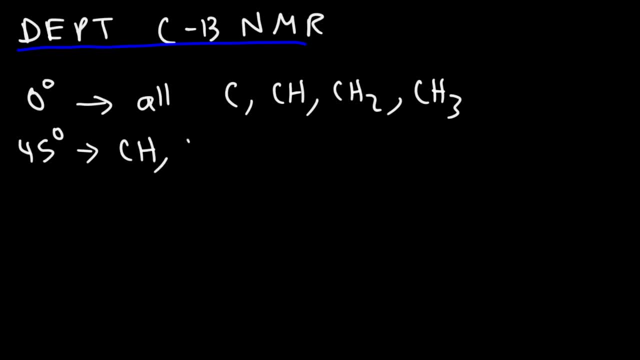 45 degrees, you'll see the methane groups, the methylene groups, the methyl groups, but you won't see any quaternary carbons. Now, if the angle is at 90, the only groups that you'll see are the methane groups. 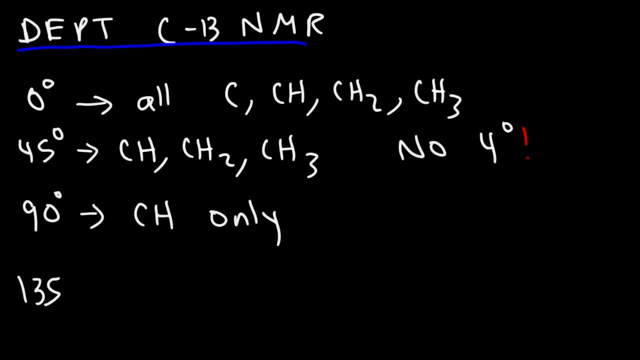 If the angle is at 135, the methane groups and the methyl groups. they will have a positive polarity, which means that the signal will be above the x-axis. The methylene groups will have basically a negative polarization, and so the signal will appear. 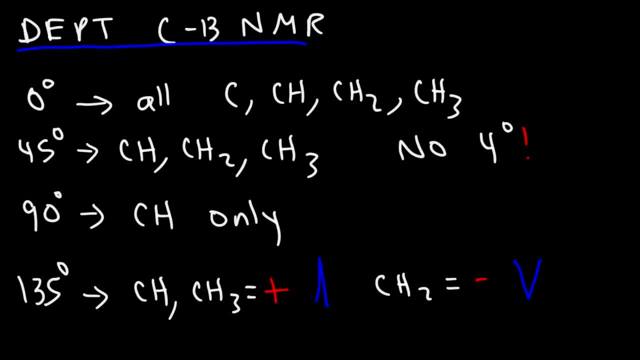 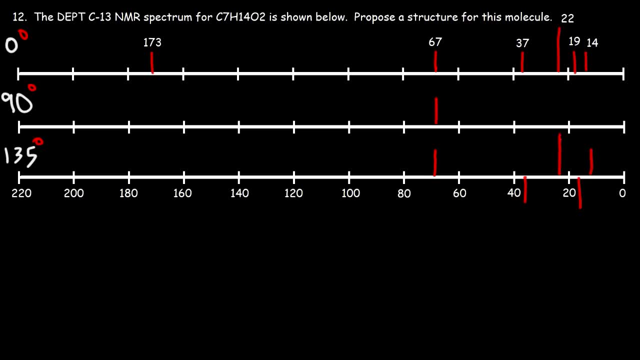 below the x-axis. So this is what you need to keep in mind when dealing with depth C13 NMR spectroscopy, Number 12.. The depth C13 NMR spectrum for C7H14O2 is shown below. Propose a structure for this. 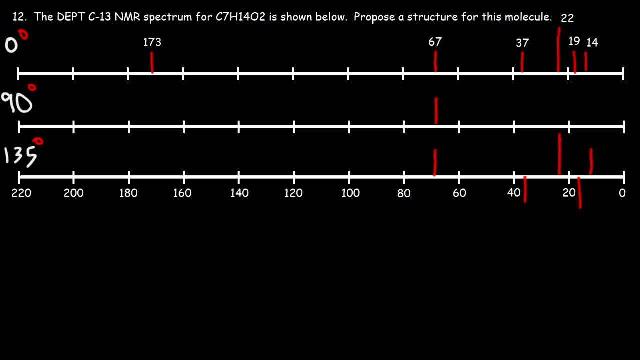 molecule. What we need to do is determine which signals correspond to a CH3 carbon, a CH2 carbon, a CH carbon or a C carbon. Now we know this corresponds to a carbonyl group. Now, it can't be an aldehyde. 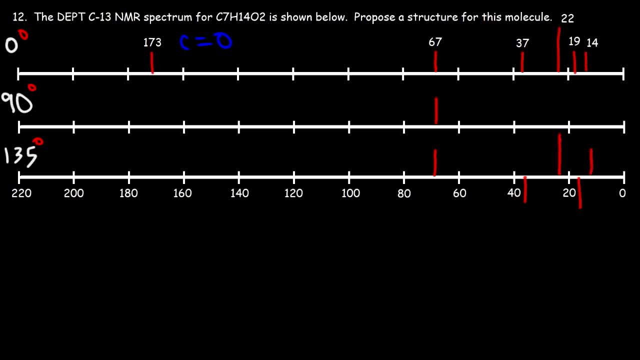 because an aldehyde would show up around 200, so it's not a CH carbonyl group, It's just a C carbonyl group. Now for 135,. notice that we got these two peaks that are below the x-axis. 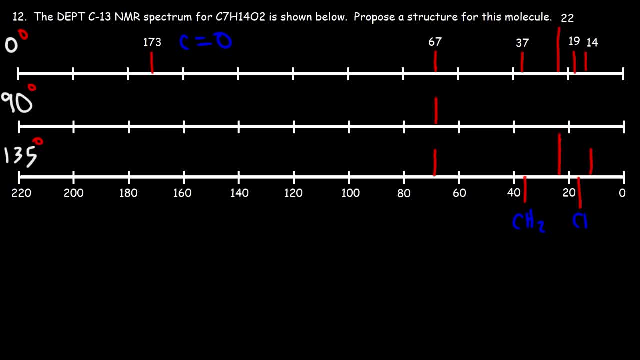 So these will correspond to the methylene CH2 group. Now 90 only shows the CH carbons, which means that the signal at 67 corresponds to a CH carbon. So these other two signals here have to be methyl groups because they're not. 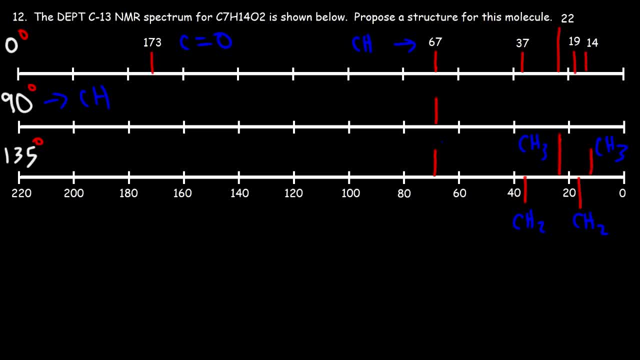 present at the 90 degree excitation angle. So at this point we've identified all the peaks that we see here. Now there's one more thing that we need to mention. That is the signal at 67.. Between 50 and 100,. 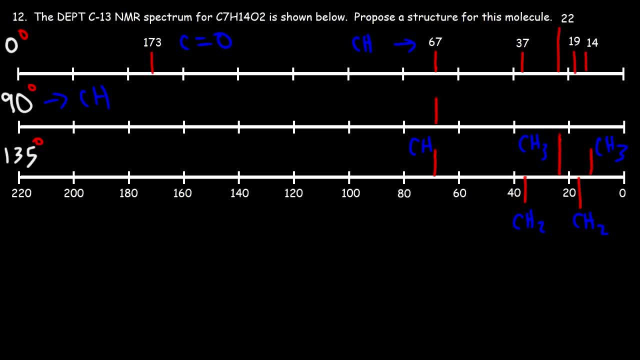 we know it could be a CO bond, like an ether, an ester, or it can be an alcohol, or the signal at 67 could be an alkyne. So we need to calculate the IHD to eliminate some possibilities. So it's going to be 2n plus 2. 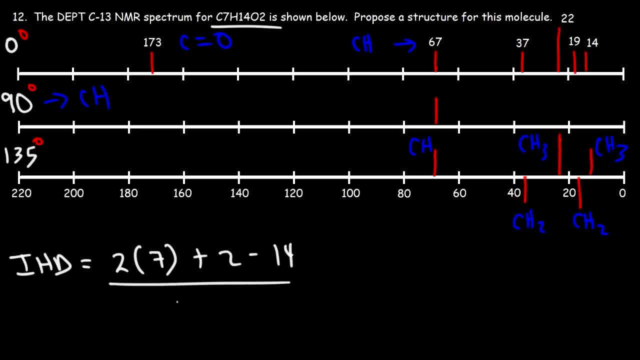 where n is 7, and there's 14 hydrogen atoms divided by 2.. 2 times 7 is 14, which cancels with the negative 14 on the right, And so we have 2 divided by 2 left over. 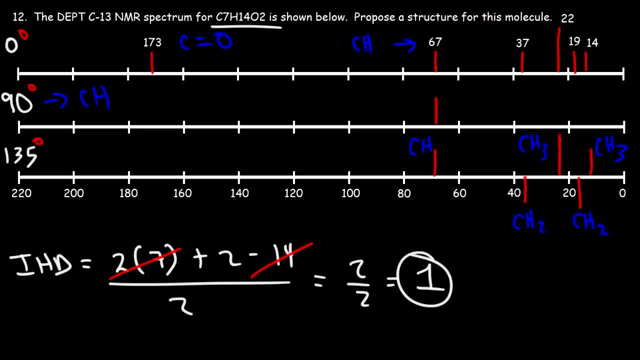 giving us an IHD of 1.. So we have either one double bond or one ring, And automatically we see that we already have a double bond here. So there's no room for a triple bond, Which means this has to correspond to a CO signal. 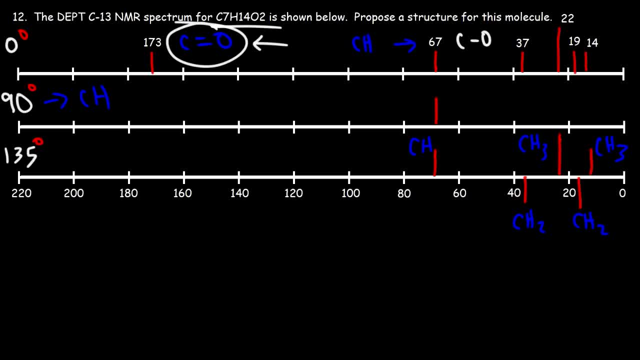 So we could have an ester, or we could have a ketone and an ether, But the signal at 173 is not consistent for ketones. Ketones exist around 210.. So this must be the carbonyl group of an ester. 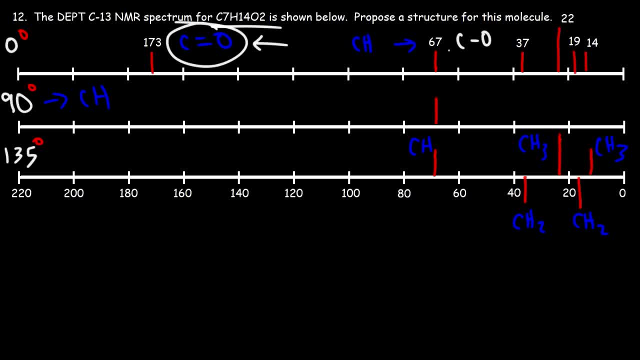 And we know it's not a carboxylic acid, because the carboxylic acid won't have a CO signal at 67.. It'll only have the carbonyl group, typically around 180.. So this indicates that we have an ester functional group. 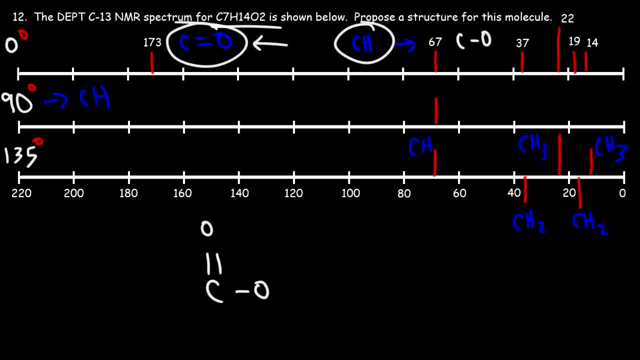 Now automatically, we know that the CH has to be attached to the oxygen. And what else do we know? Now? we have 2 methylene groups and we have 2 different types of methyl groups, So the methyl groups will be at the end. 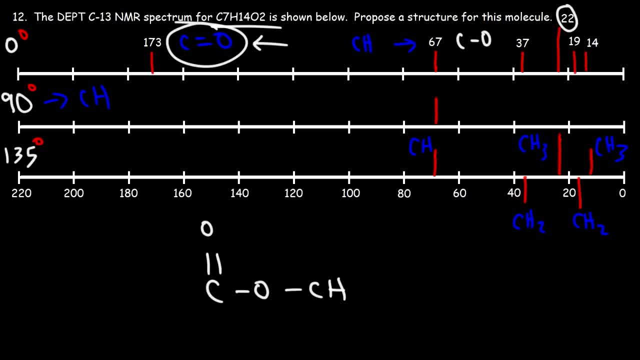 But notice that the signal at 22 is much higher than the signal at 14.. So one of the methyl groups will be an isopropyl group. So this has to correspond to 2 methyl groups, And the reason why we could say that is: 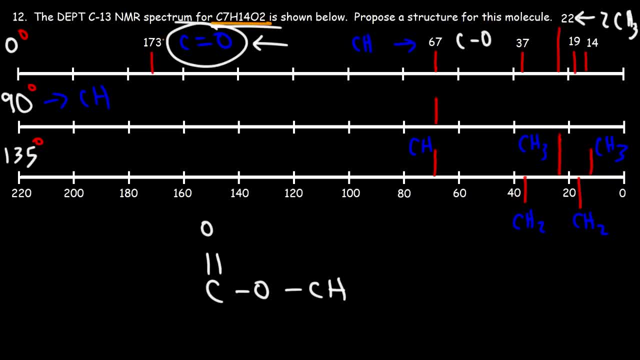 notice that we have a total of 7 carbons in this structure, but we only have 6 signals. So that means 2 carbon atoms have to be equivalent. So this indicates that we have an isopropyl group, Which is usually 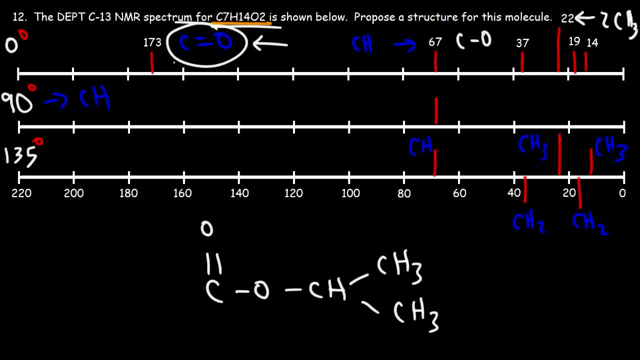 attached to a CH carbon. So far we've considered the carbonyl group, the CH carbon, the methyl group, with the one that has the tallest peak, And so left over we have 2 methylene groups and another methyl group. Now the other methyl group has: 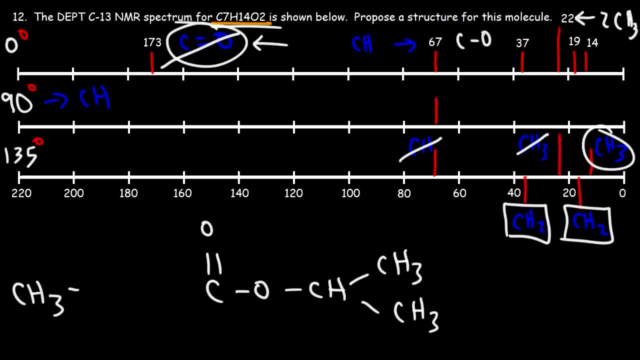 to be at the end. The methylene groups exist in the middle of a chain without any additional branching, And so the structure has to be this. So the carbonyl group is the one with the signal at 173, the CH group at 67,. 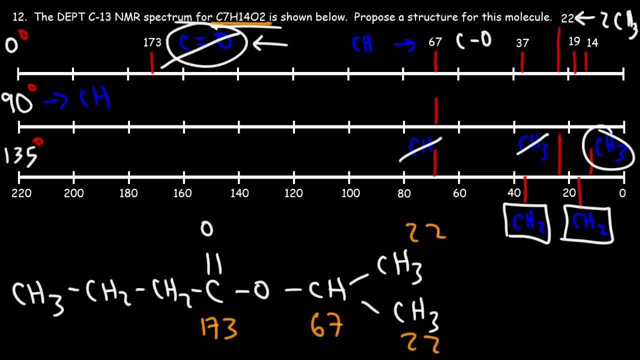 the 2 methyl groups at 22,. and then this methylene group next to the carbonyl group must be this signal here- which is at 37. The other one is at 17,, and the other methyl group is 14..